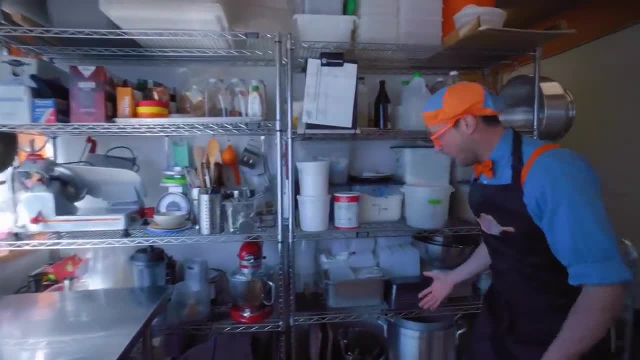 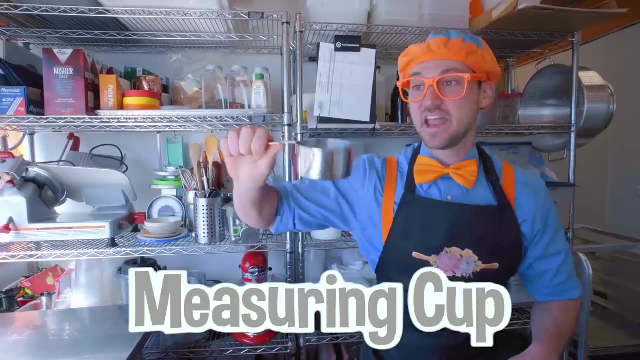 Wow, Wow. Look at this place- Whoa, there's so many cool things. Yeah, like a measuring cup. Yeah, you can put things in there and then know how much of an ingredient you have exactly in this measuring cup- Whoa. 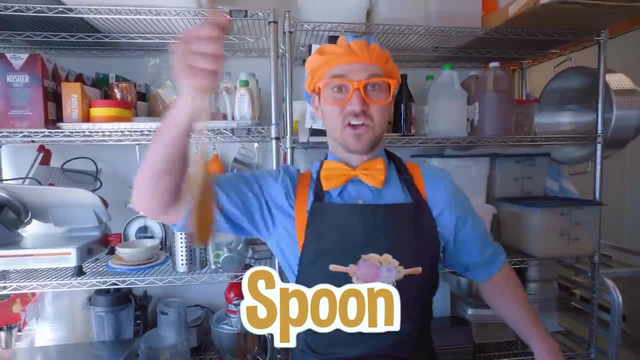 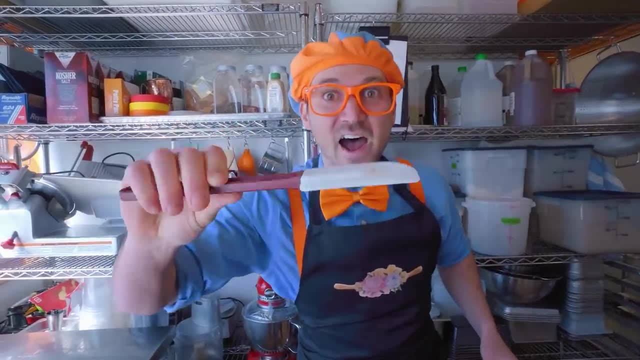 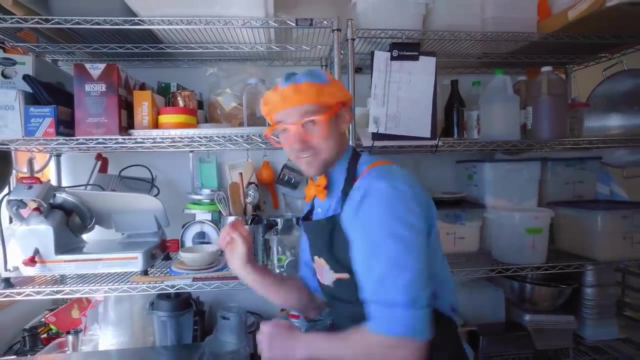 Or a giant spoon, Whoa. You can stir a lot of stuff with that Whoa, Whoa. And look at this: Yeah, a spatula Boing. That's so cool. Okay, let's set it right there for now. 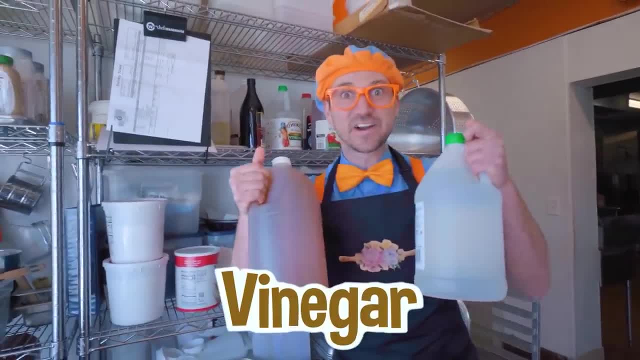 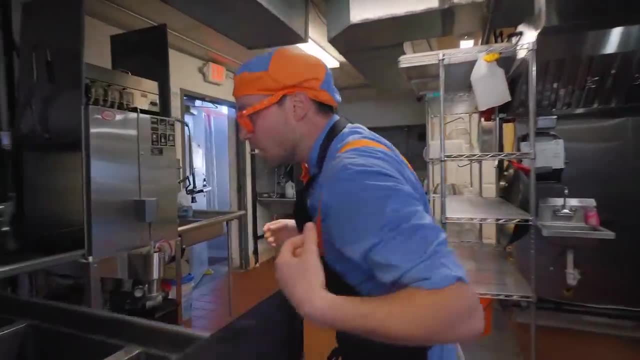 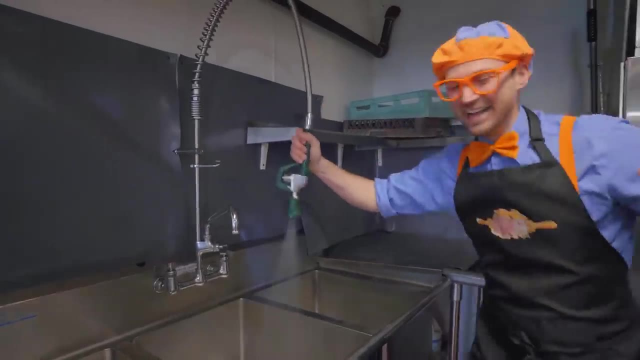 Whoa, Looks like we have some vinegar. Yum, Okay, there we go. Wow, come on. Whoa, A giant sink. Woohoo, Yeah, This is where I clean a lot of dishes, Woohoo. 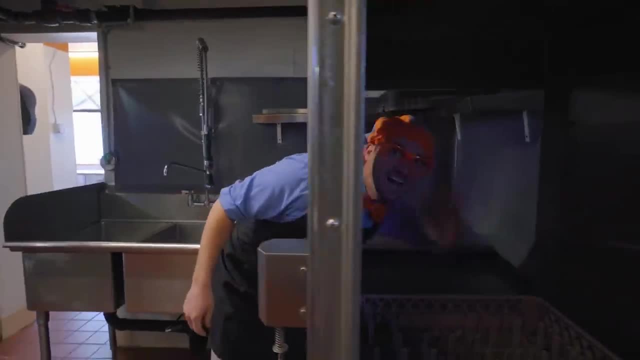 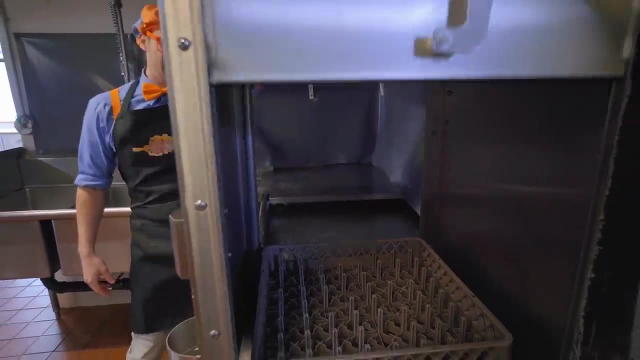 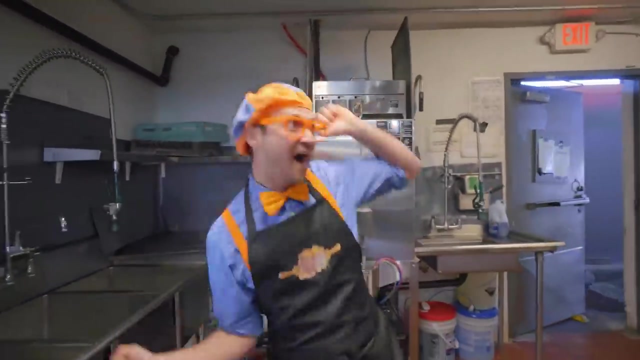 Oh, speaking of cleaning dishes, Whoa, Hello, Look, This is a dishwasher. You put a lot of dirty dishes right here and then You close it down. Yeah, That is awesome. Woohoo, Whoa, Check it out. 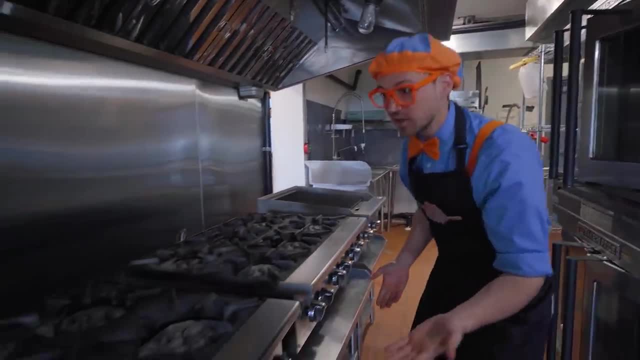 This is a stove top. Whoa, You can cook so much food right here. Whoa, There's so many stove tops. Whoa, do you see the little fire right there? It's a fire, It's a fire, It's a fire. 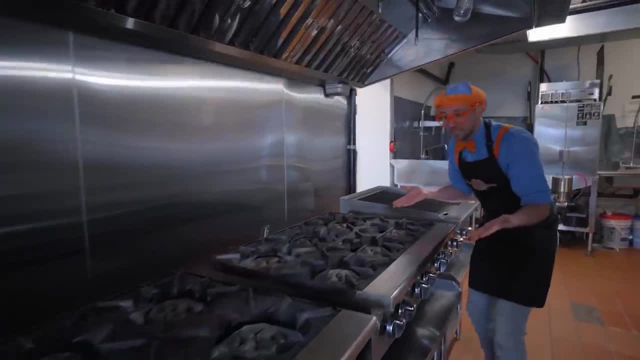 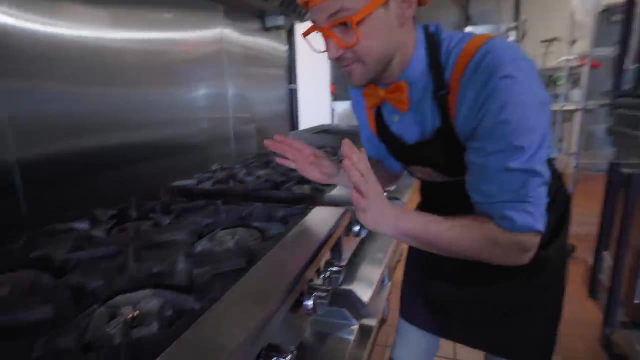 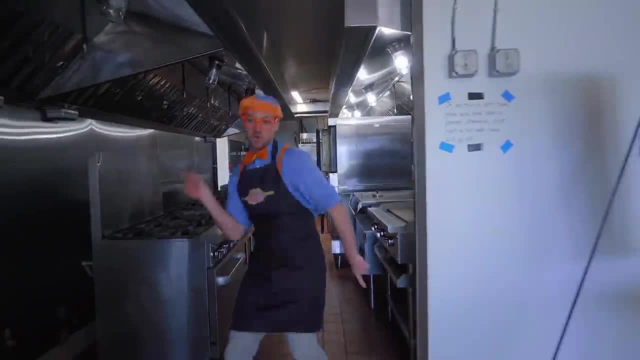 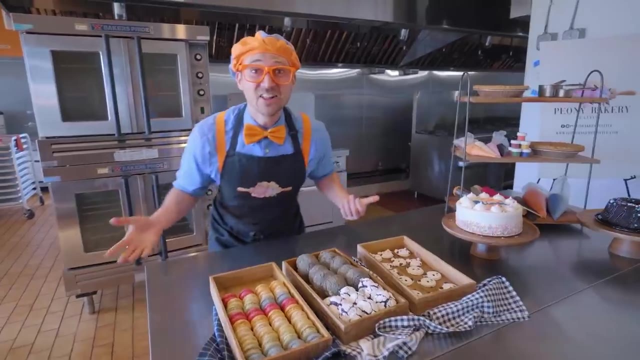 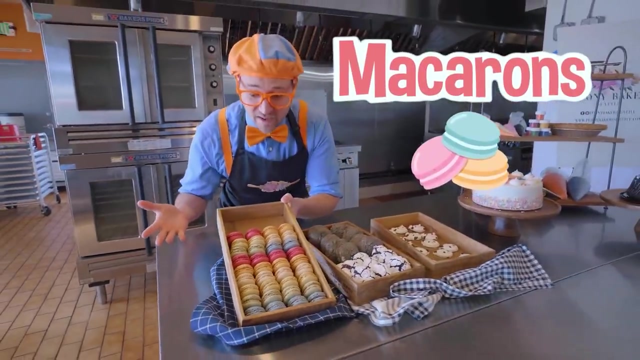 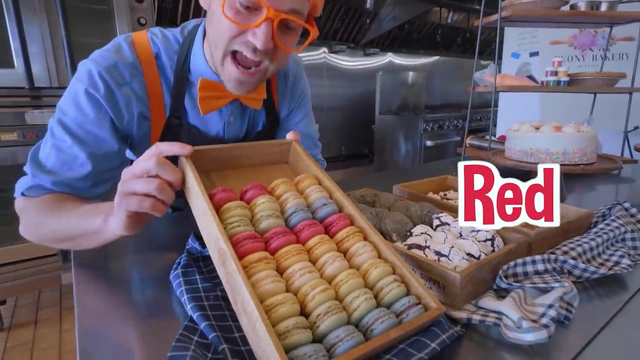 Haha, Whoa, Yum, Yeah. Look at these sweet treats. Wow, These are macarons and they look so yummy. Look at this one. This one is the color red. Whoa, Looks like we have some green and some blue and some orange. 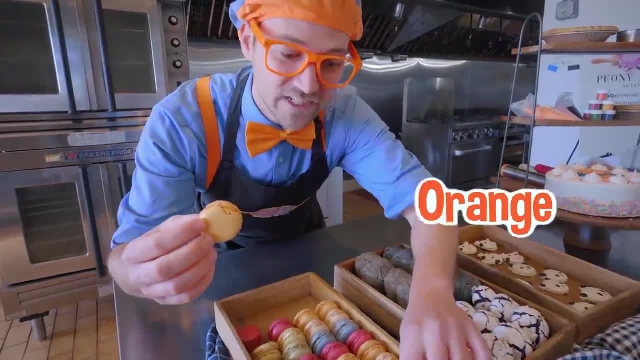 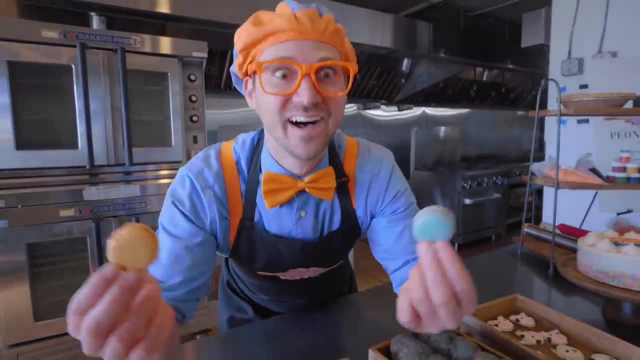 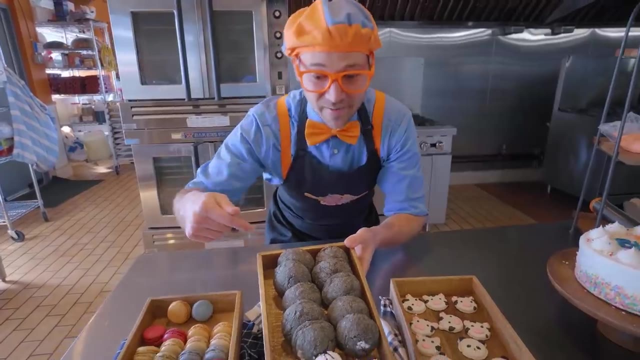 Whoa, Look, I'll grab an orange and a blue, My two favorite colors. I'll eat these later. Whoa, We have some black sesame cookies- Yum, And some ube cookies- Yum. Check these out. 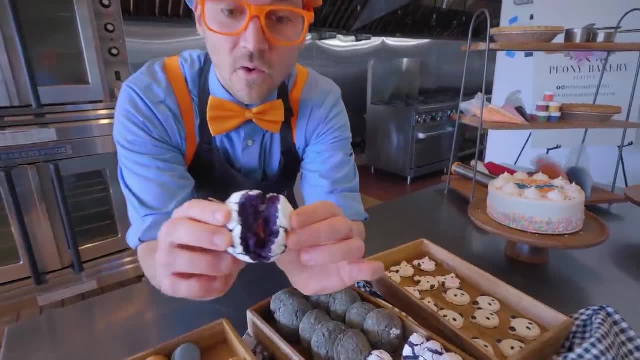 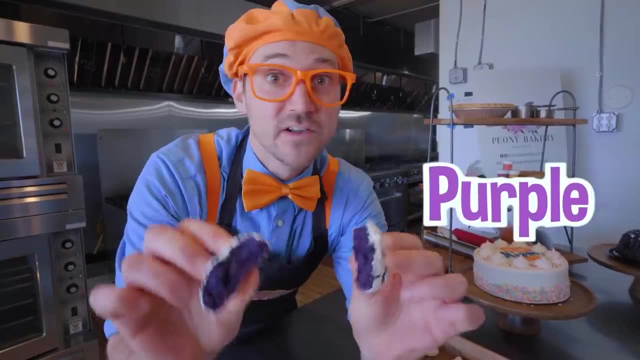 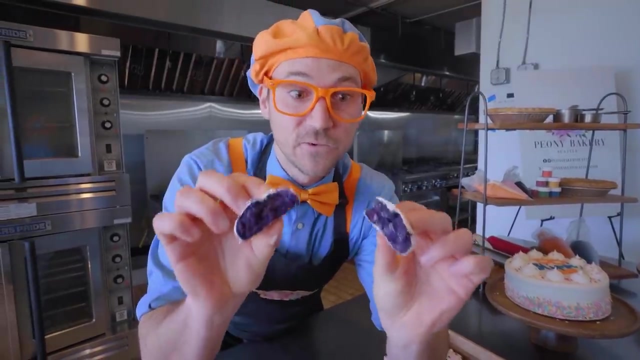 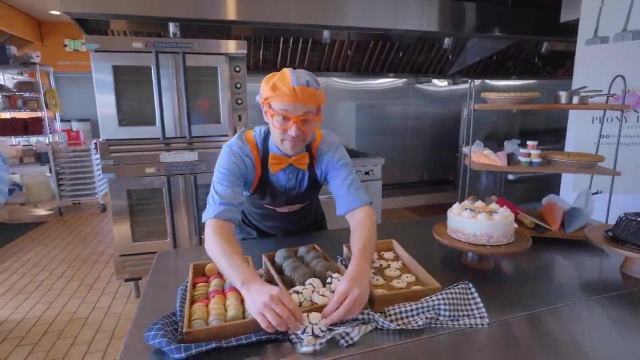 Open these up. Wow, What color is that? Yeah, the color purple. Yeah, there's no food coloring in this. That, yeah, that is the color of the food that was added into this cookie. That's so cool. Okay, we'll put that right there for me to eat later. 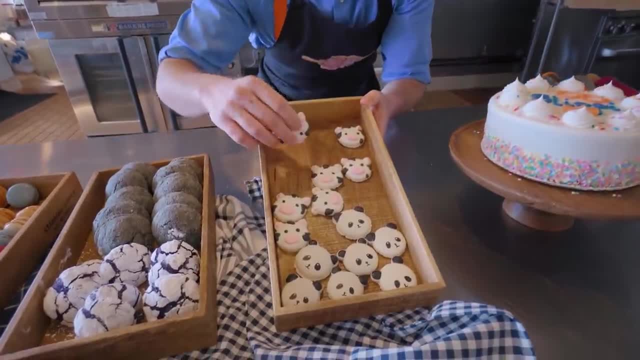 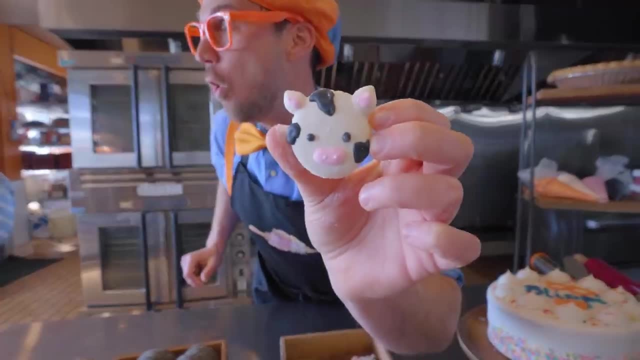 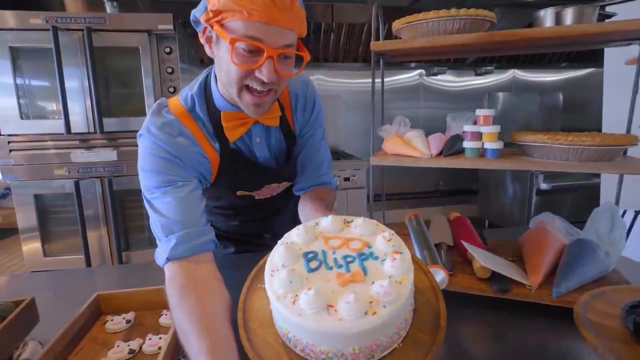 Whoa, Look at these cute things. Look so cute. Looks like What animal is that? Yeah, Moo Moo. Yeah, A cow. Whoa A vanilla cake. Yeah, Blippi party cake. Will you spell my name with me? 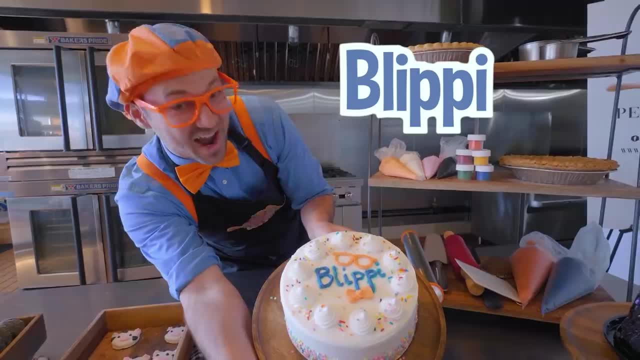 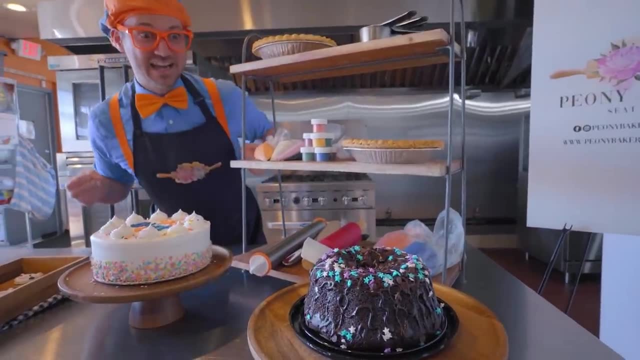 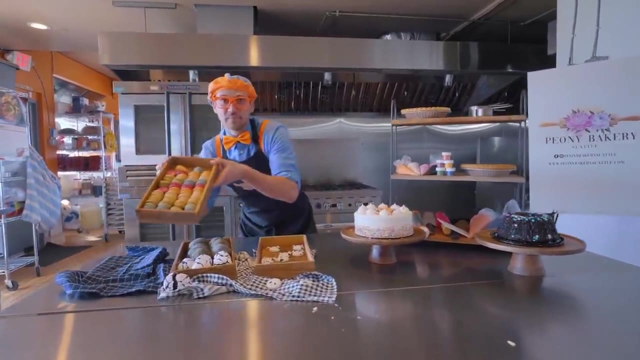 B-L-I-P-P-I Blippi, Yeah, And a triple chocolate cake That looks so yummy. Well, hey, maybe you and I can cook and bake some of this. Yeah, how about today we make some macarons? 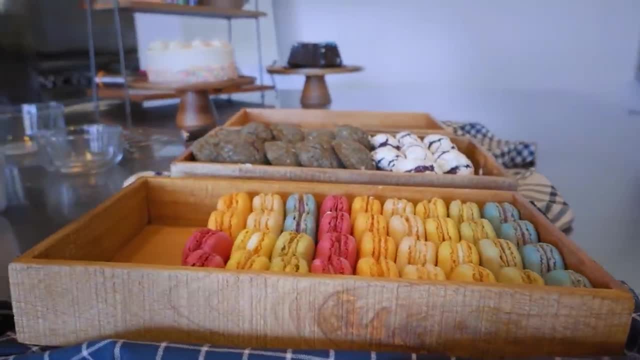 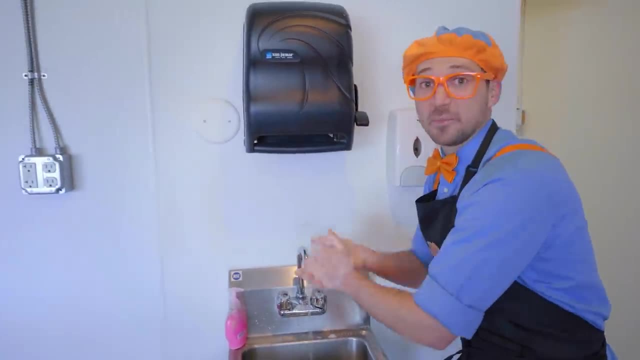 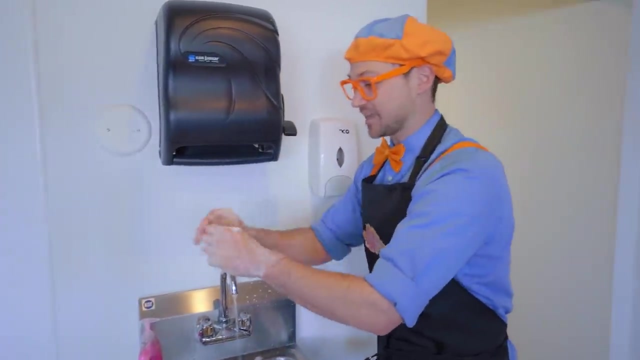 Yeah, Whoa, check it out. I'm washing my hands and I'm scrubbing them for 20 seconds. Yeah, do you know how long 20 seconds is? Yeah, it's about the same length as when you sing the ABCs. 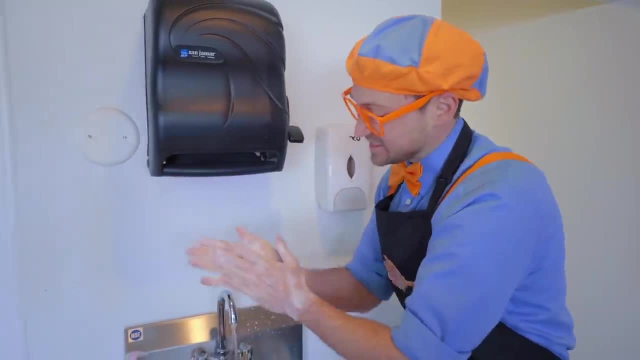 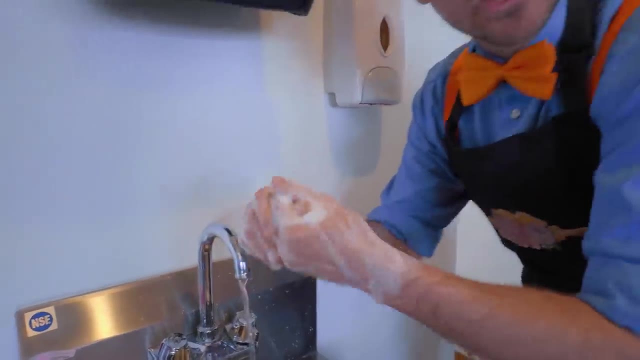 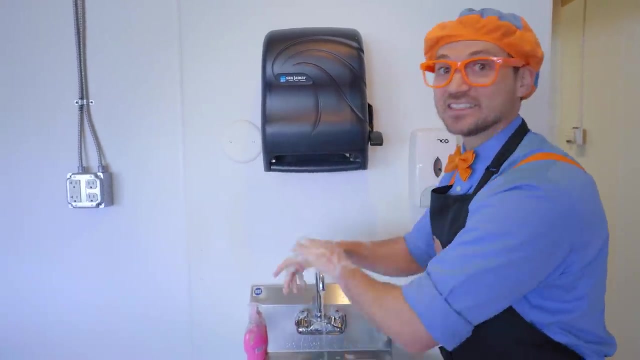 Will you sing with me: A, B, C, D, E, F, G, H, I, J, K, L, M, N, O, P, Q, R, S, T, U, V, W, X, Y and Z. 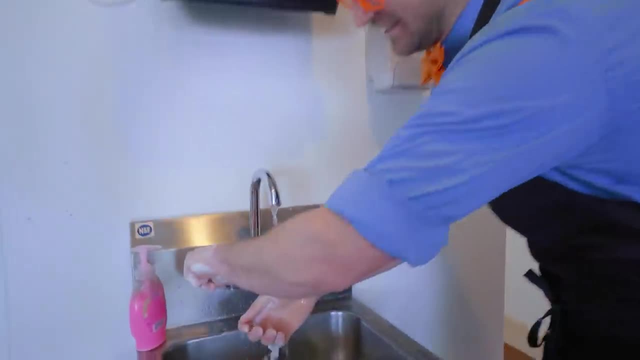 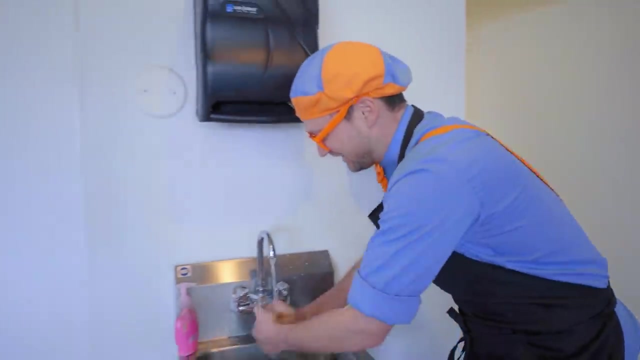 Hey, There we go. Okay, let's rinse them all off. Whoa, They're nice and clean. now, Okay, Perfect, Shut off the water. Oh wow, And now I'm ready to make some delicious treats. Oh hey, who are you? 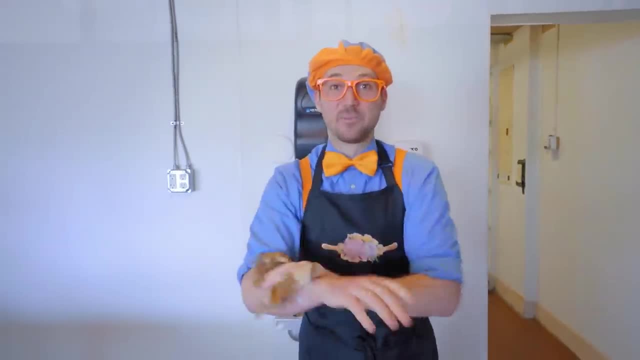 Hi, I'm Jennifer. I'm the baker for Candy Bakery. Whoa, nice to meet you. I'm Blippi. Are these the ingredients? Yeah, these are some ingredients for some macarons. Ooh well, what do we have here? 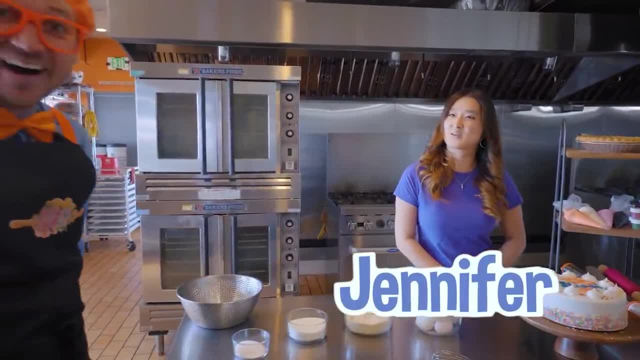 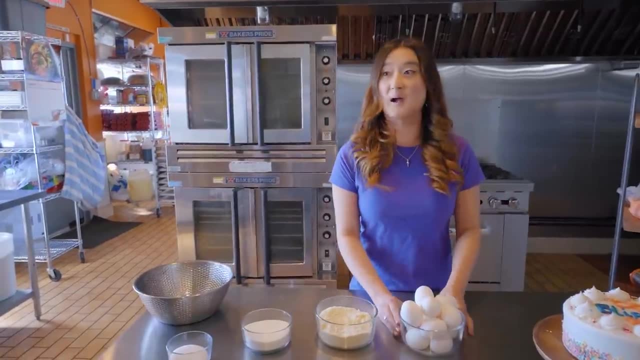 Well, first we have eggs and we have almond flour, we have sugar and we have an important ingredient. Okay, So what are we going to make today? We're going to make some macarons, Okay, So what are we going to make today? 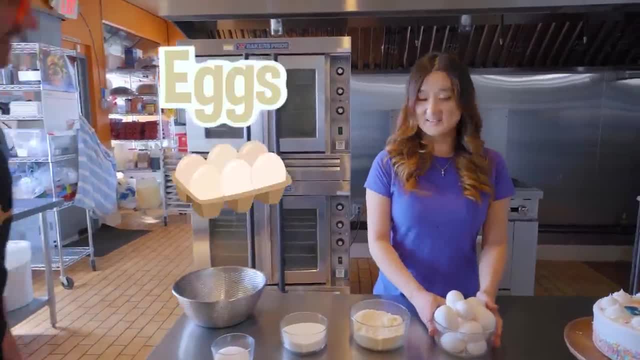 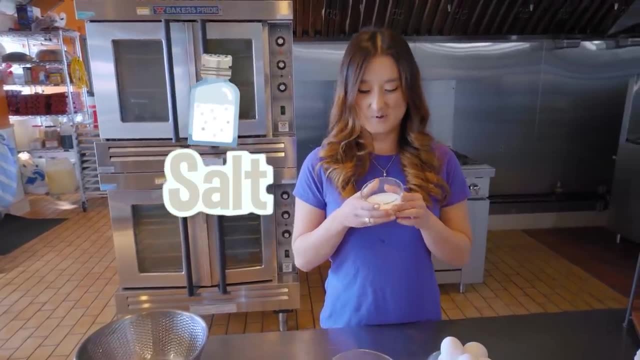 We're going to make some macarons, Okay. So what are we going to make today? We have eggs and we have almond flour, we have sugar and we have an important ingredient called salt, And when you eat it it's really salty, but when you put it in desserts it actually makes. 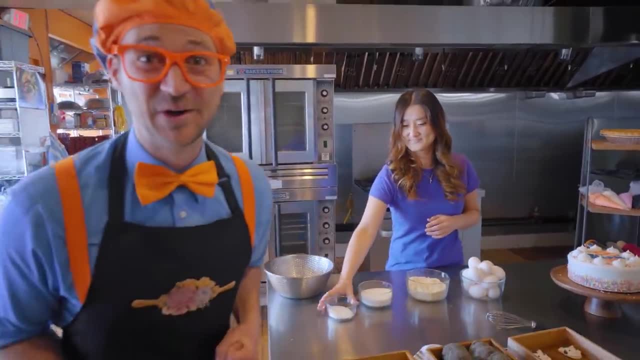 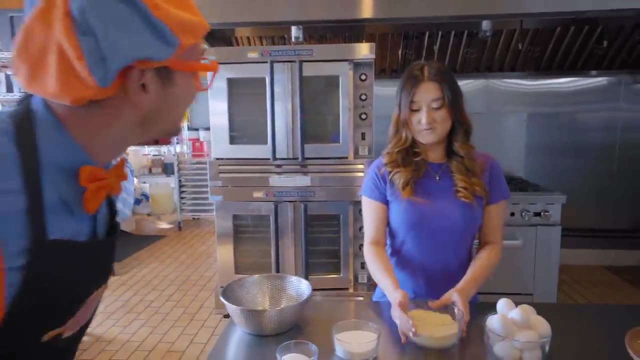 it sweeter and tastier. Ooh, that sounds so yummy. And you said almond flour. Why are we using that rather than all-purpose flour? So almond flour is special because when you put it in macarons it makes it less sticky. 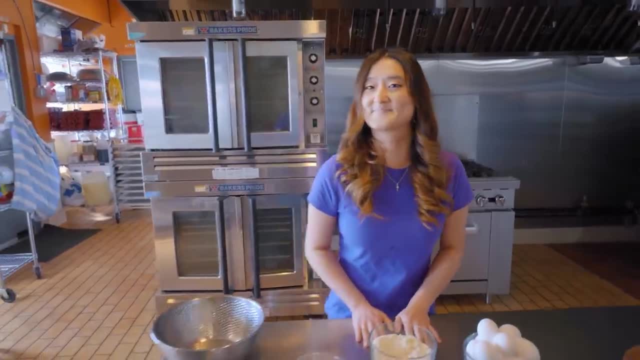 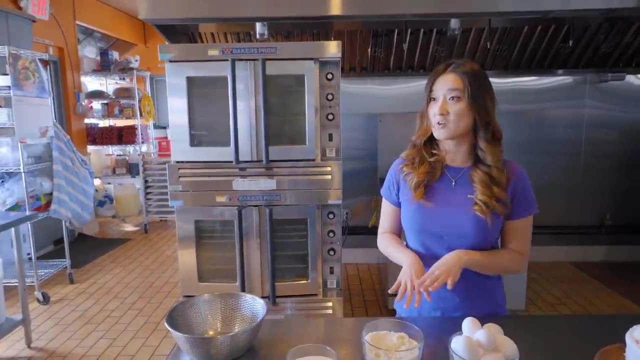 than flour and makes it really light. Wow, That is so cool. Well, hey, Do you mind if I mix all these ingredients? Yeah, How about you throw all the ingredients into a bowl and throw it into the mixer and I'll. 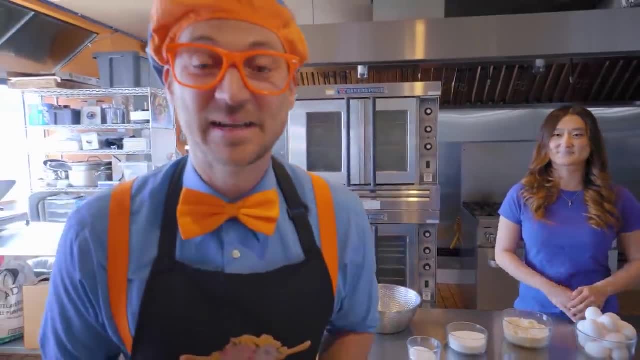 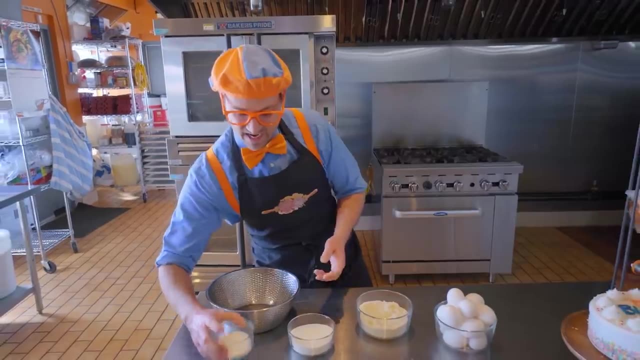 go get the oven ready. Okay, Woohoo. All right, Let's mix all the ingredients together and then we'll put it in the mixer. All right, First let's add the salt- Perfect- And then we'll add the sugar. 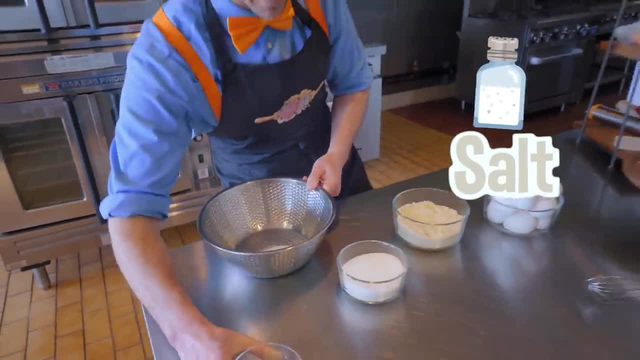 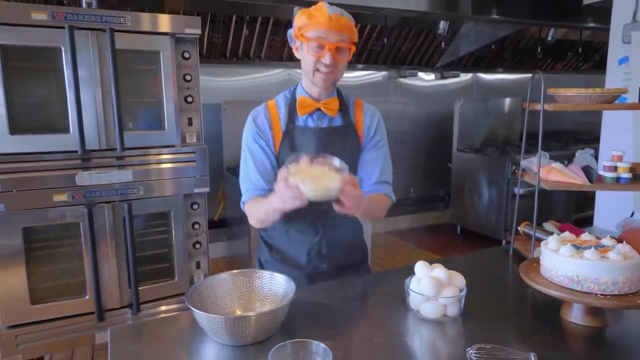 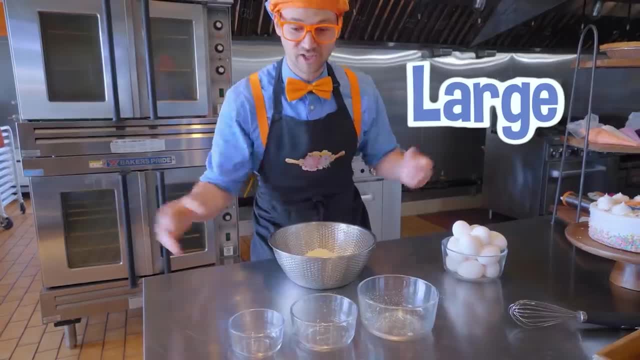 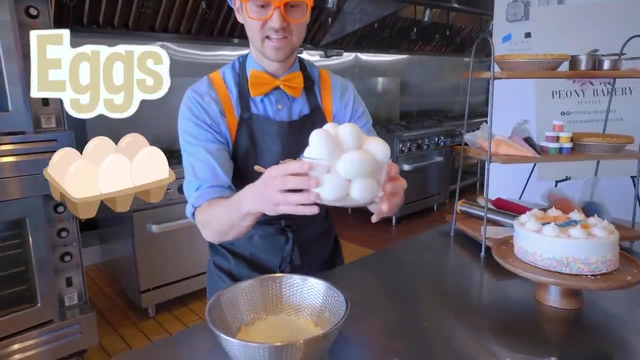 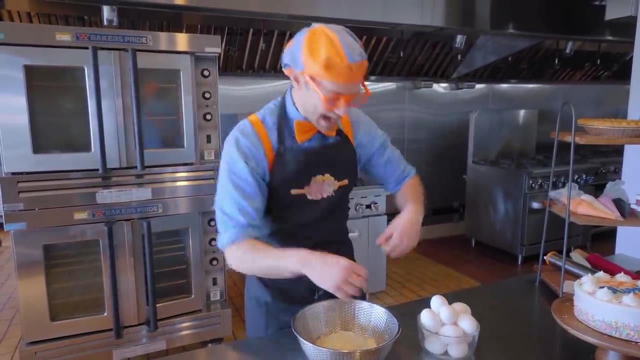 Perfect. Oh hey, Check it out. A small bowl, medium and large, There we go. Perfect. And for the eggs: oh, wait a second, I probably have to break them open. All right, here we go. 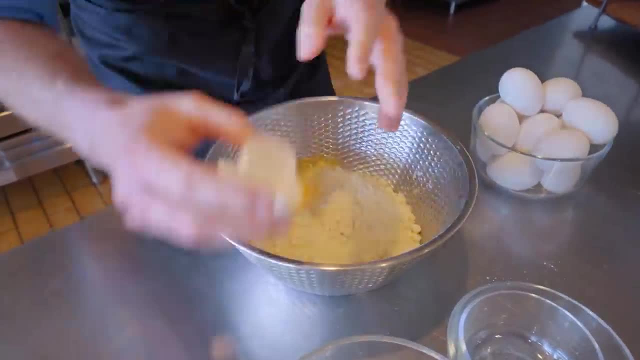 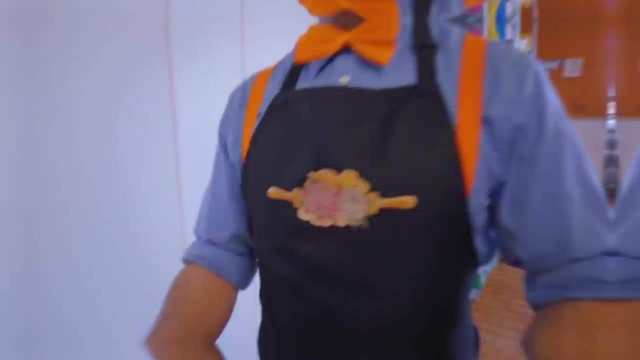 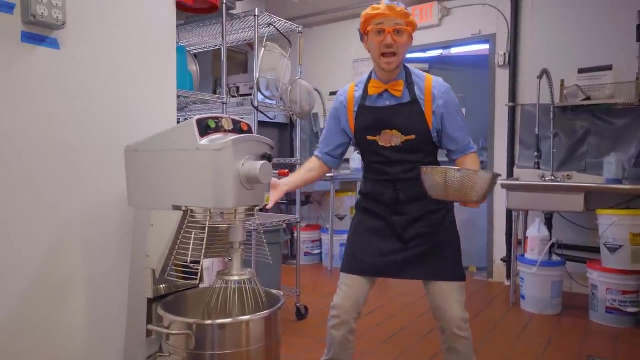 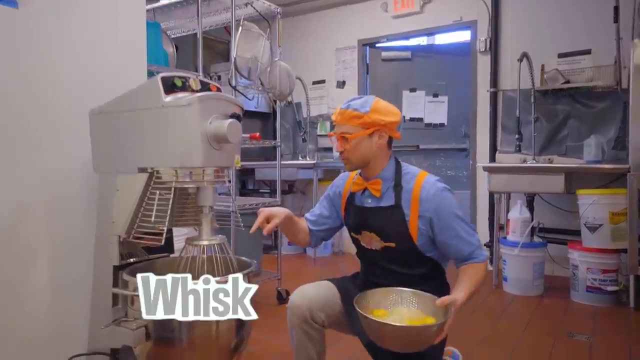 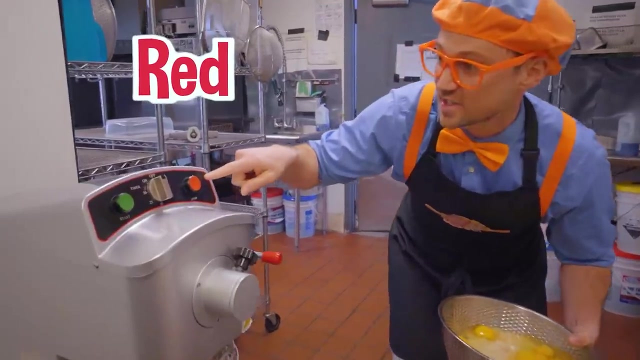 Ha ha. Now I'm gonna go put it in the mixer. Whoa, Hey, Check it out. This is a massive mixing machine. Whoa, Look how big it is. There's a giant whisk right here. Wow, Looks like there's a green on button, a red stop button. 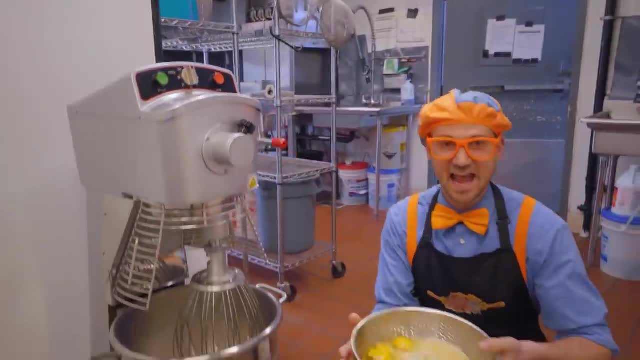 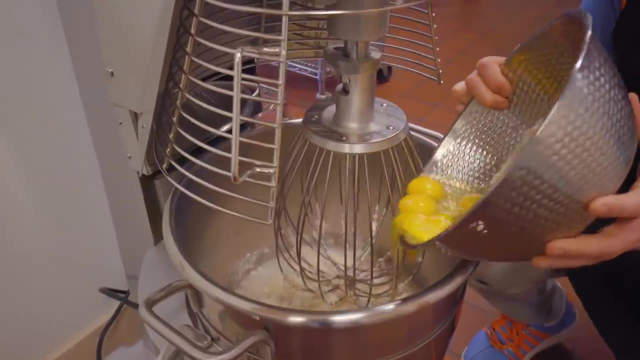 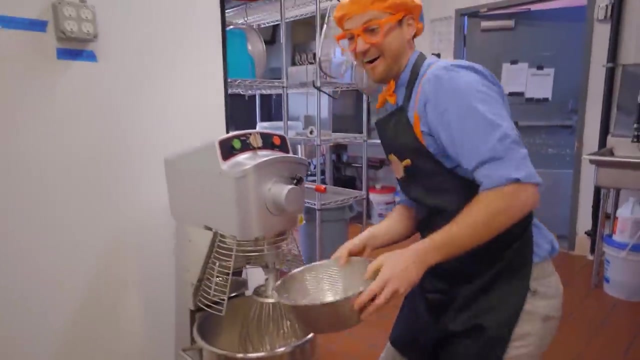 and a big bowl for me to add all the ingredients. Alright, here we go, Pour it in. Looks like we already made some earlier. Yeah, this is going to be a big batch. Alright, now that all the ingredients are in there, we need to make sure that the cover is closed. 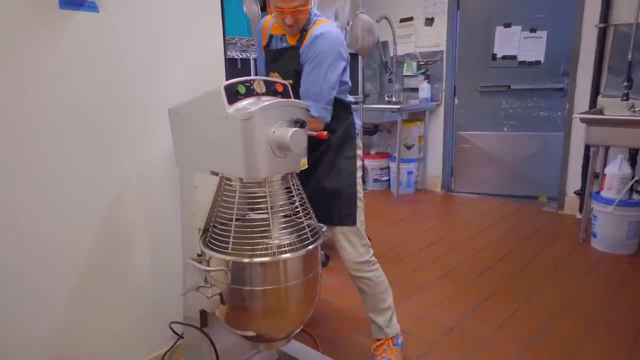 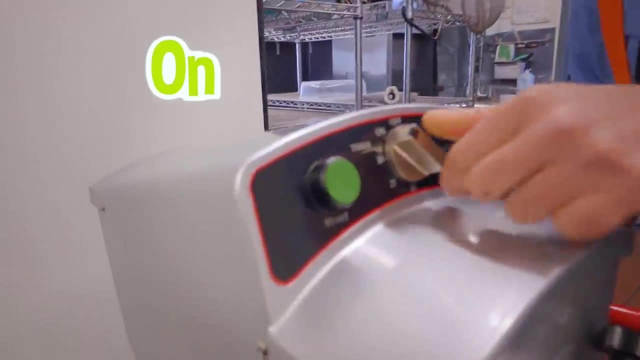 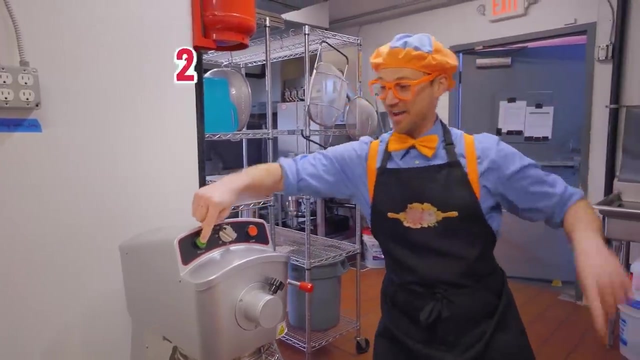 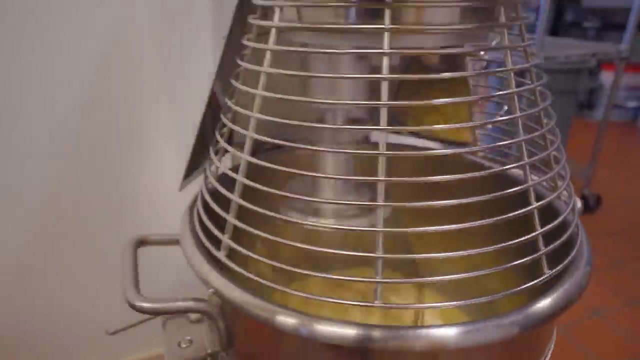 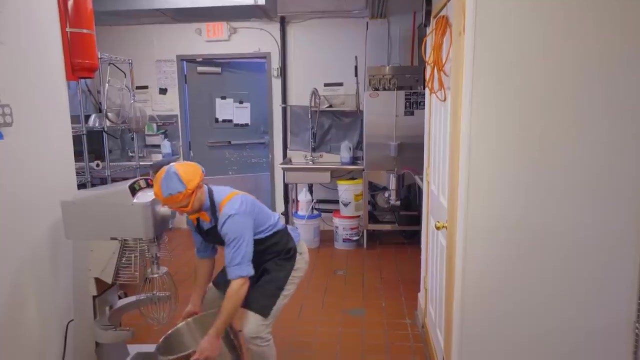 We need to raise up the bowl. There we go, And now we need to turn this to the on position. There we go, And we'll push the green start button in three, two, one, Yeah, Look at it, mix, Wow, Yeah. 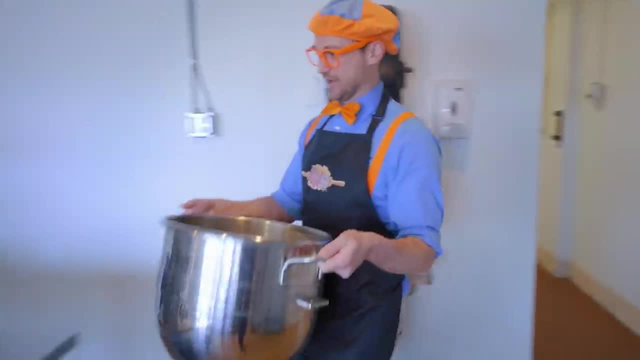 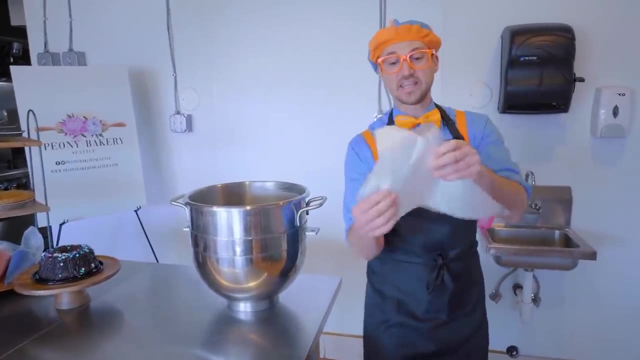 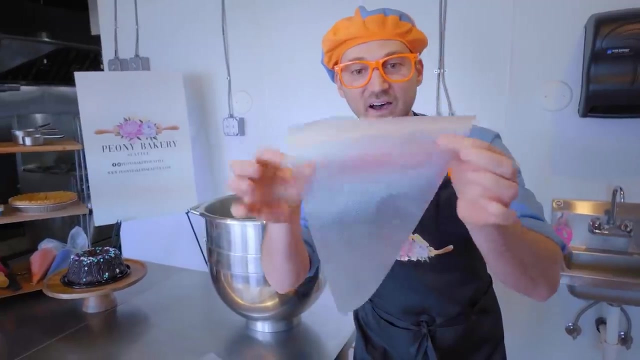 The batter is finished. Whoa, This is a big bowl. Okay, the next step that we need to do, yeah, is take some of this batter and put it inside these piping bags. Yeah, What shape is this piping bag? Oh, Yeah, 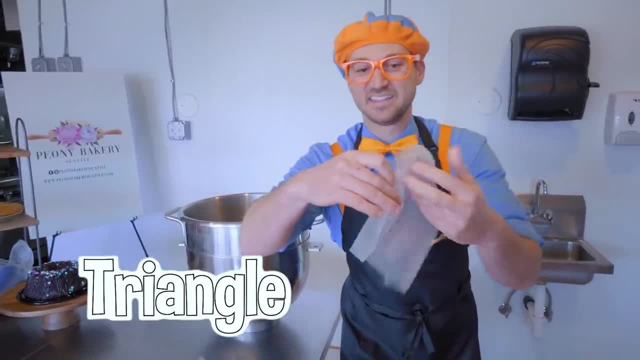 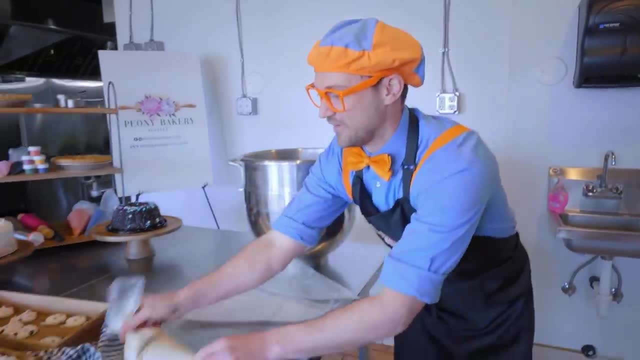 Looks like a triangle. Perfect. And do you see how you open it up? Yeah, That's where you put all the batter. But hey, check it out. Yeah, we have some batter already in a piping bag, Woo-hoo-hoo. 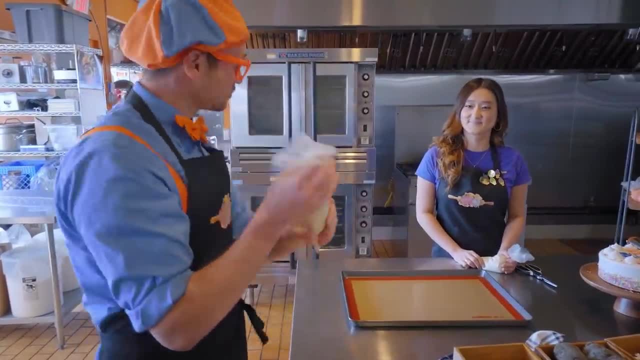 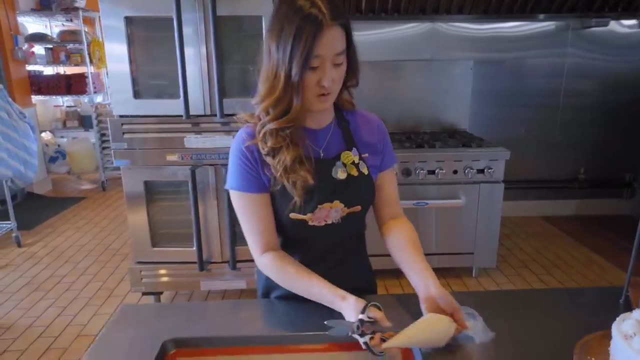 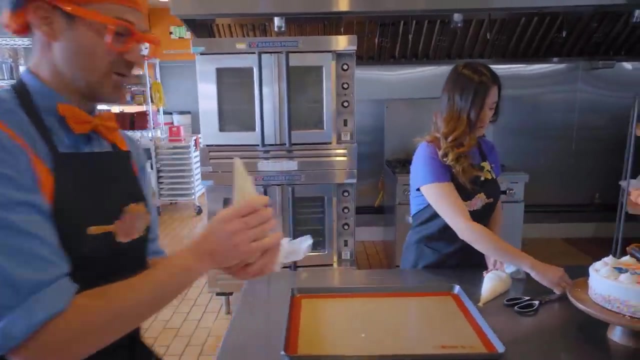 Okay, Jennifer, now that we have the batter in the piping bags, what do we do now? Well, first we need to cut the bag. Okay, Cut one, Okay, And we're going to make some cow macarons. Ooh. 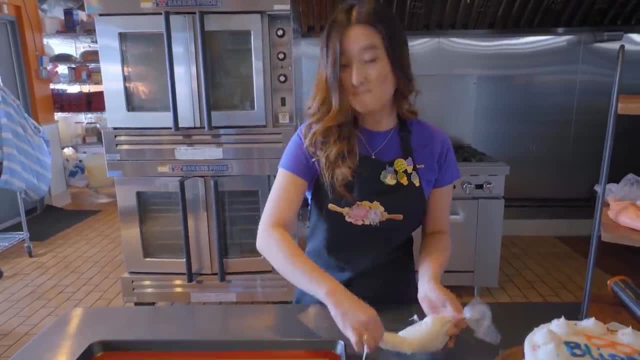 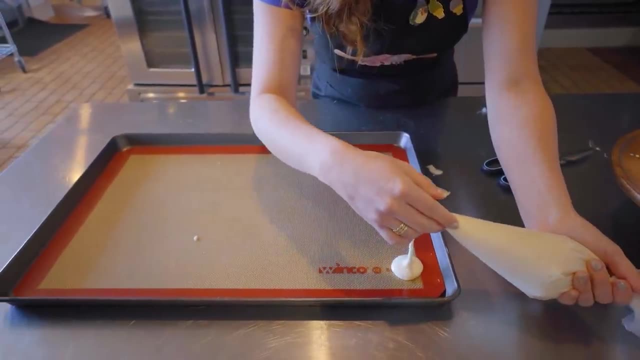 So to do that first, you're going to need one big circle. Okay, I'm going to make cow macarons And we need a big circle, for is that the head? That's going to be the head, yeah, Okay. 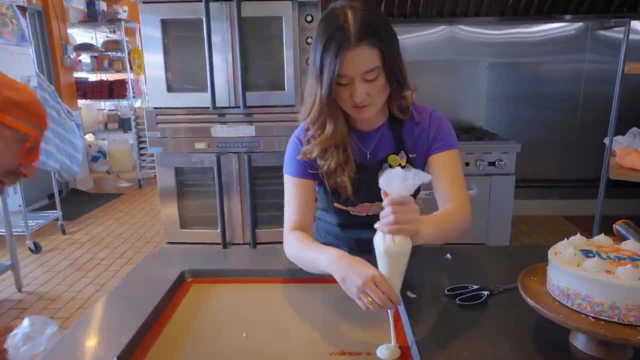 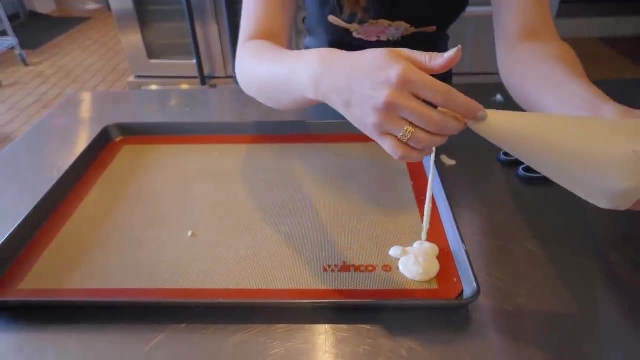 Then we need two small circles on the top for its ears. Okay, That is not how I want it to look. That's funny. That's okay. Okay, I see it. Yeah, the head and then two ears Here, let me try. 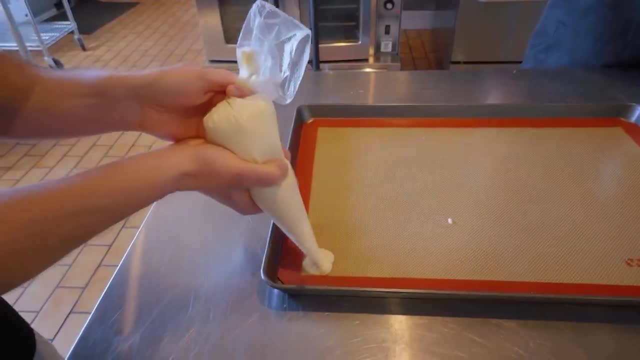 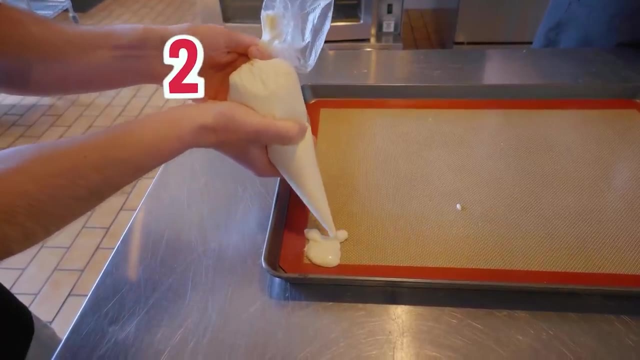 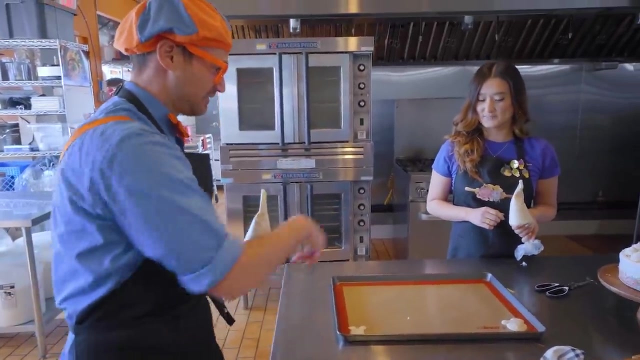 All right, There we go. Yeah, just like that. And then one ear, two ears, Perfect, That's going to be one great cow. Okay, do we fill it up now? Yeah, let's fill up the whole pan. 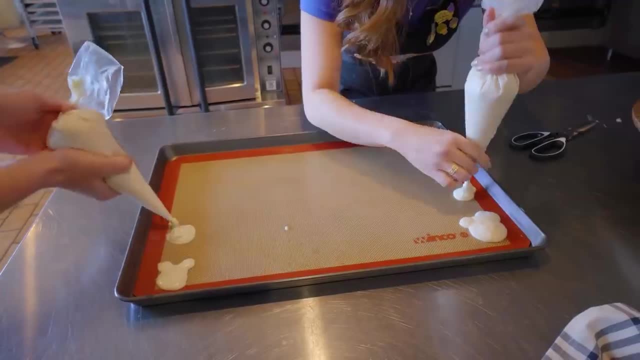 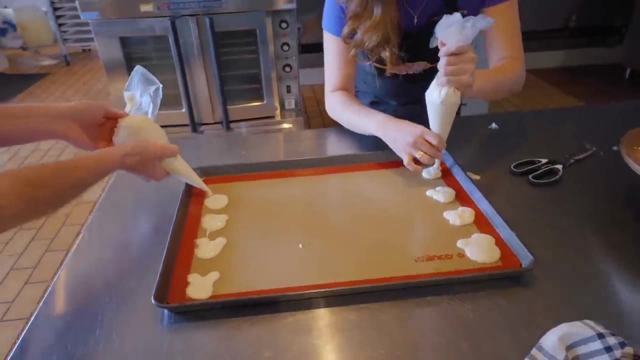 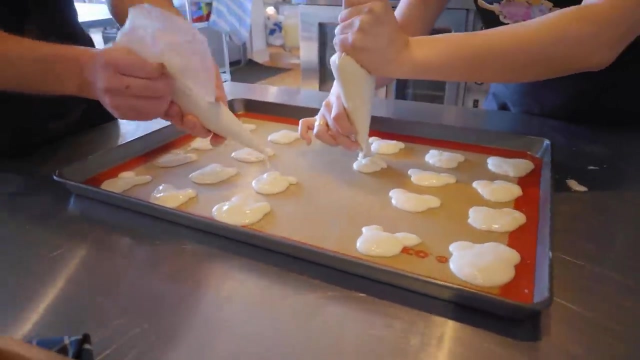 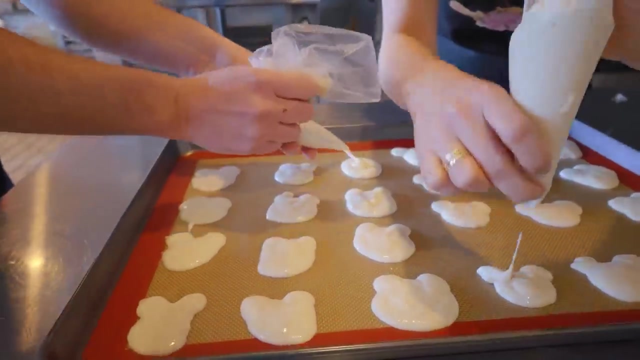 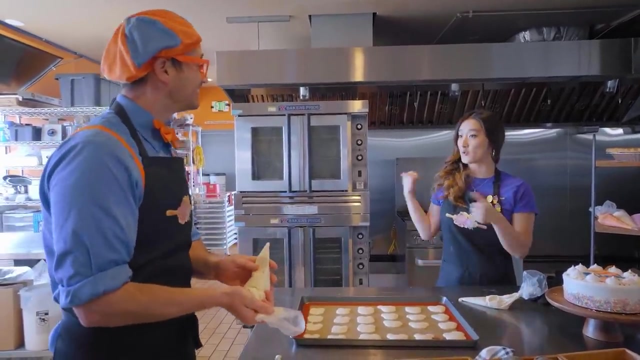 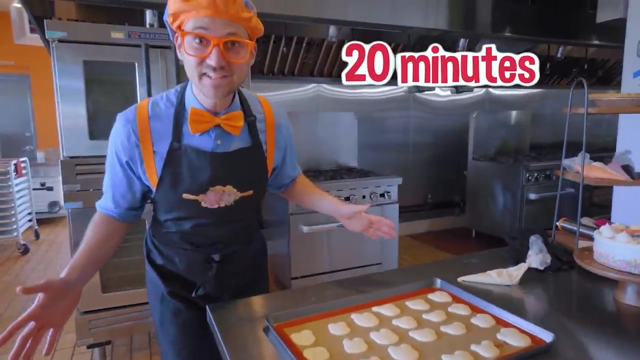 All right, let's do it. Yeah, Whoa, That was so much fun. Yeah, now that we're done, why don't you throw them into the oven for 20 minutes and I'll get the buttercream ready? Okay, All right, So I need to throw these in the oven for 20 minutes? Whoa. 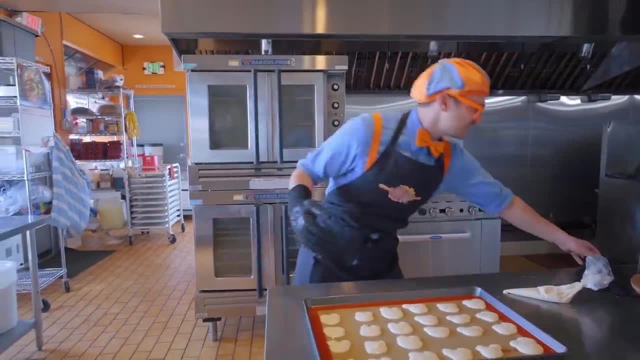 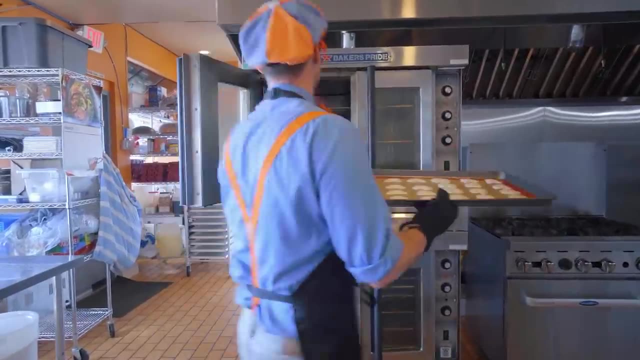 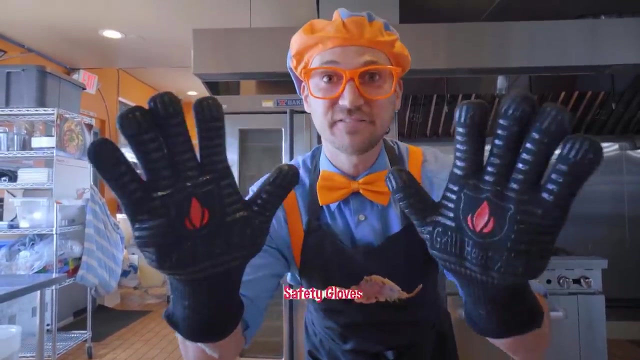 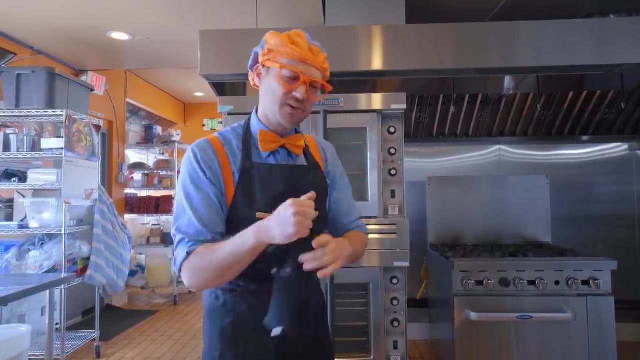 All right, So I'm going to put on these safety gloves, All right? Yeah, Here we go. Wow, I used my safety gloves because ovens are not a toy. You need to be very careful. Okay, what did Jennifer say? She said 20 minutes. 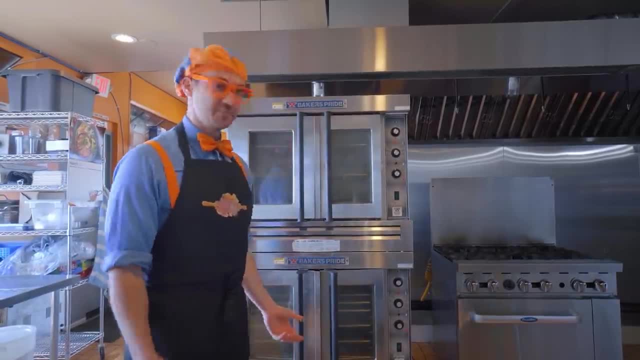 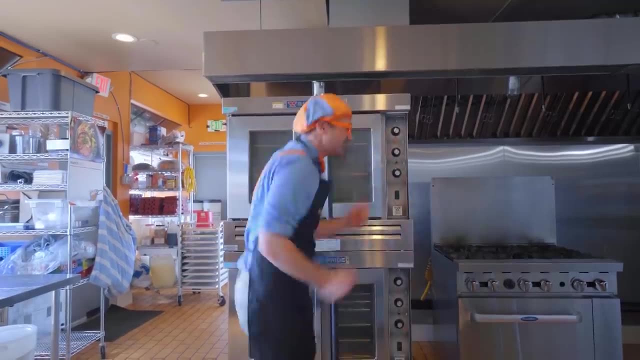 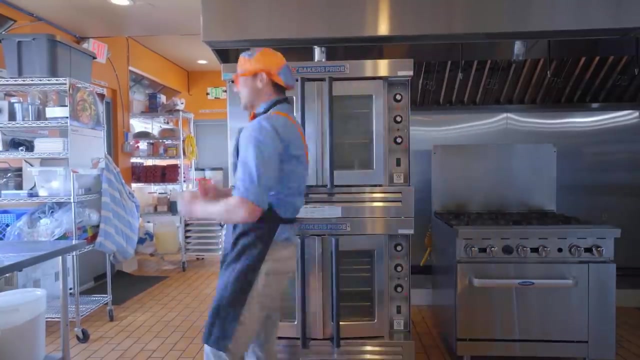 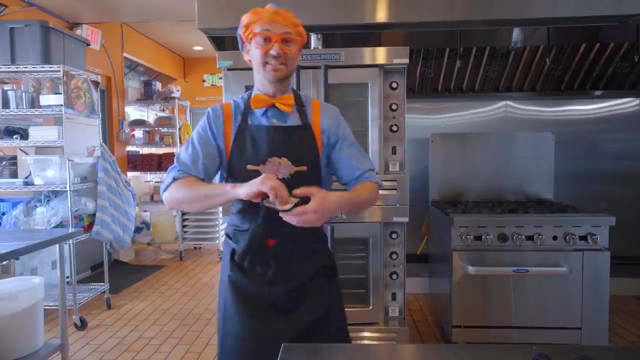 Oh, that's a long time Wait. But wait a second. You know what I like to do when I wait? Yeah, I like to dance. Woohoo, Did you hear that? Yeah, That buzzer means that they're probably done. Yeah. 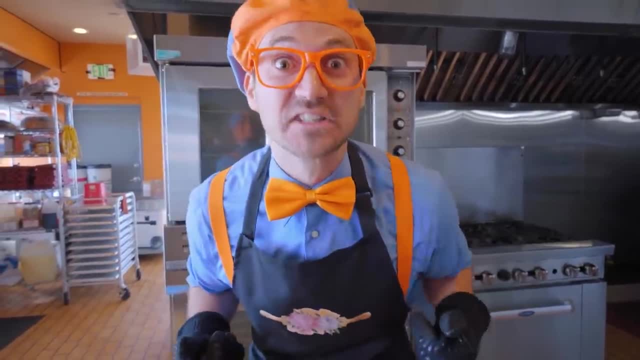 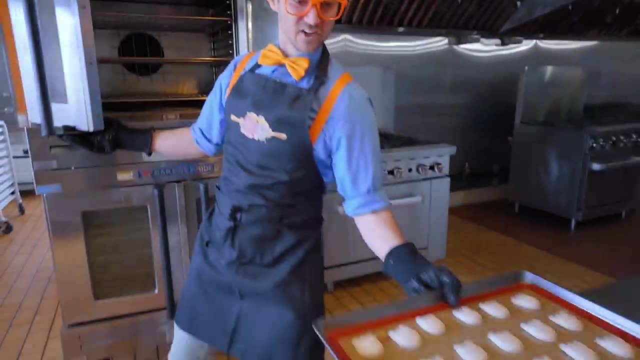 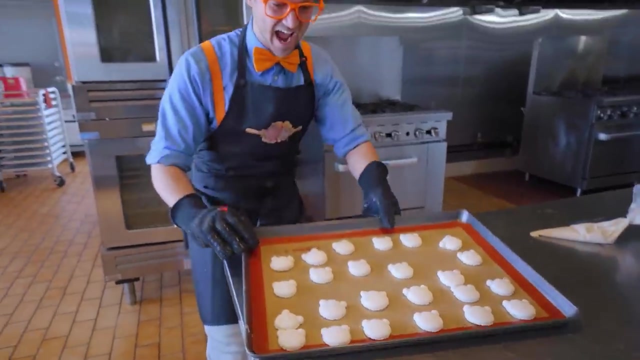 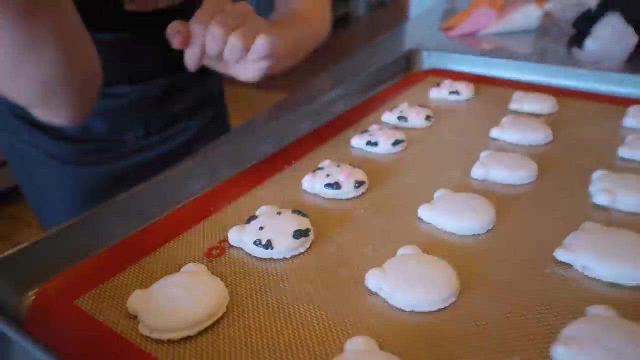 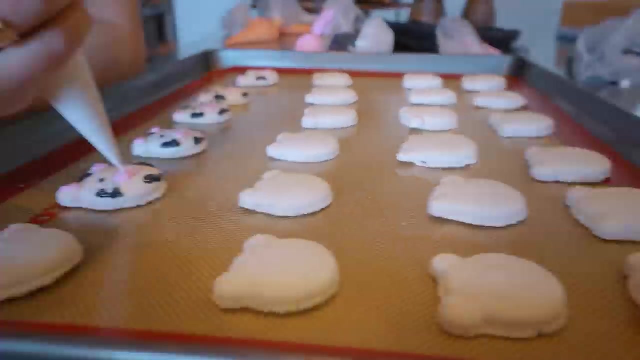 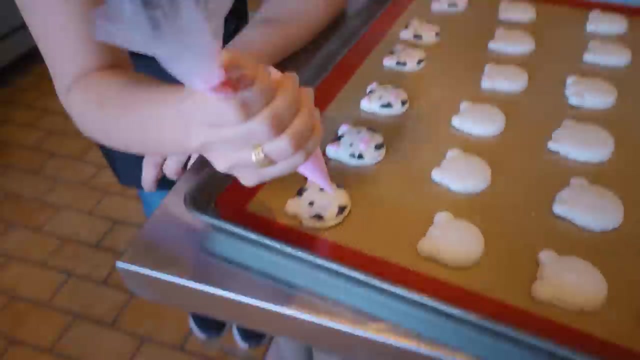 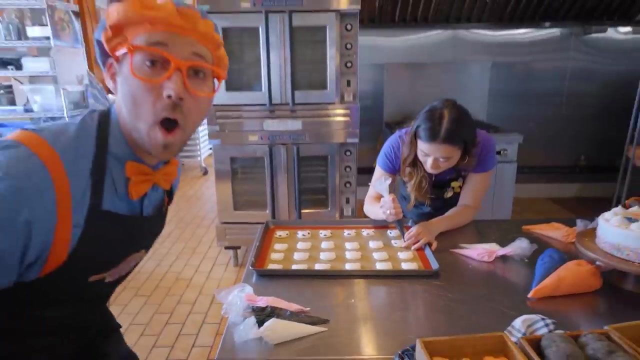 Let's open it up and then see the macarons: Whoa, Woohoo, That is hot, Woo, And they look so yummy. Wow, Check it out. Now it's time to decorate. Haha, Wow, That looks like so much fun. Hey, can I try? 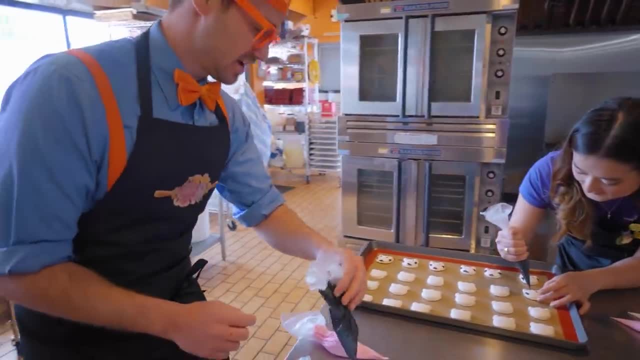 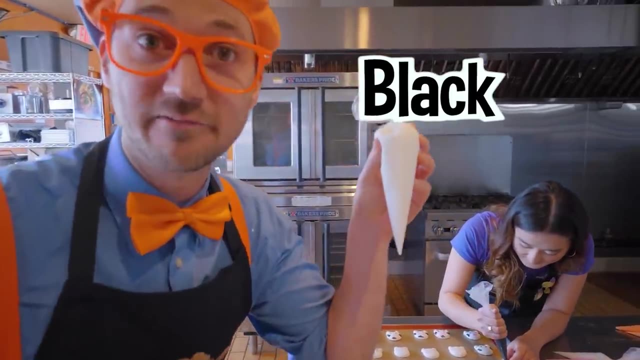 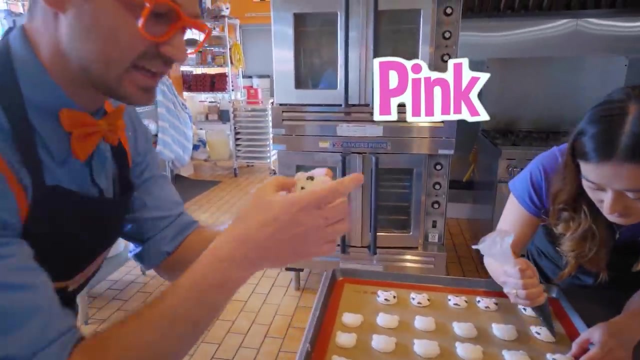 Sure, Blippi, Go ahead and give it a try. Sure, Okay. Well, looks like we have three colors here. We have black and then looks like we have white And then looks like we have the color pink. Let's see What are we making. 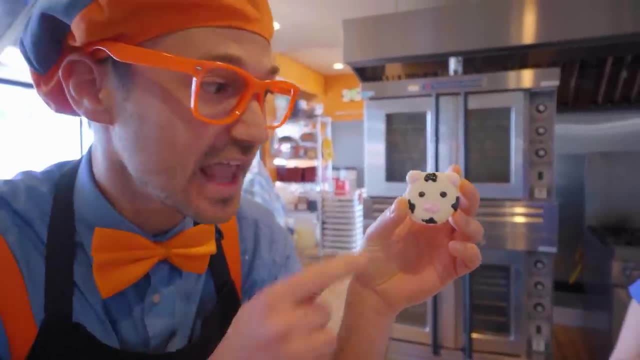 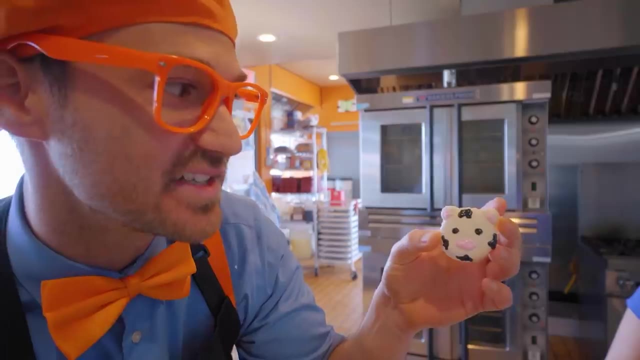 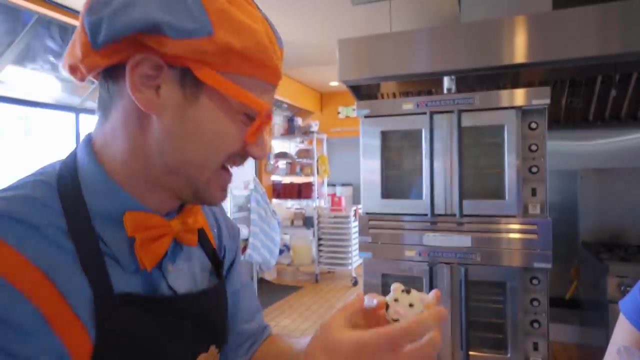 Oh yeah, Remember these from earlier. Yeah, a cow, A cute cow, Moo, Haha. Yeah, it has two eyes, has two ears, has some spots and a really cute nose, Haha. Okay, let's put that down right here. I'm going to start with the black. 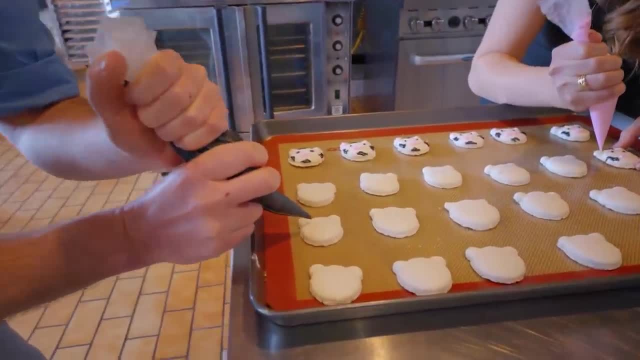 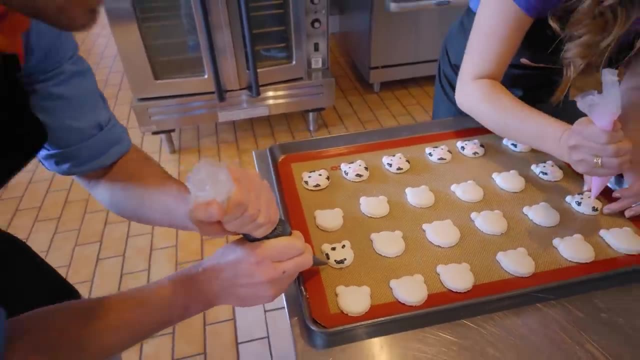 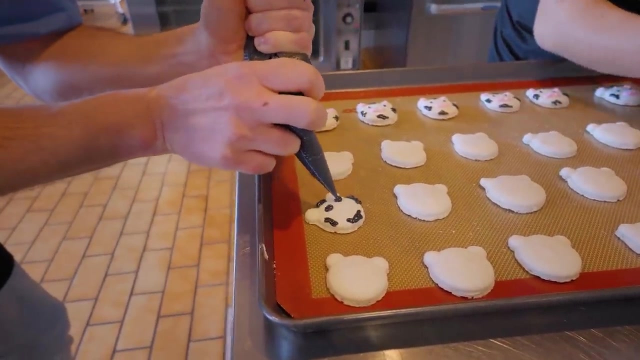 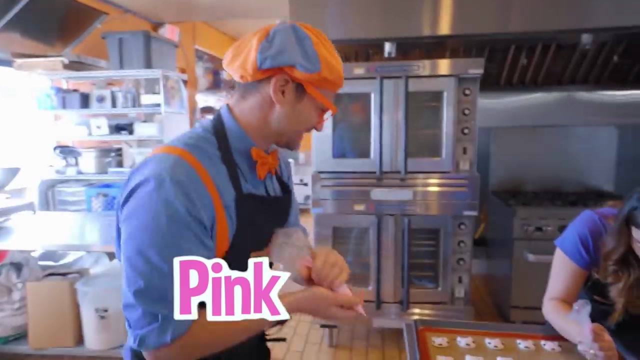 Alright, Looks like we'll do two eyes And we need to do the spots- Cute little hair thing on top, Haha, Okay. So now let me move to the color pink. Haha, Alright, Looks like pink. I'm going to put it on the ears. 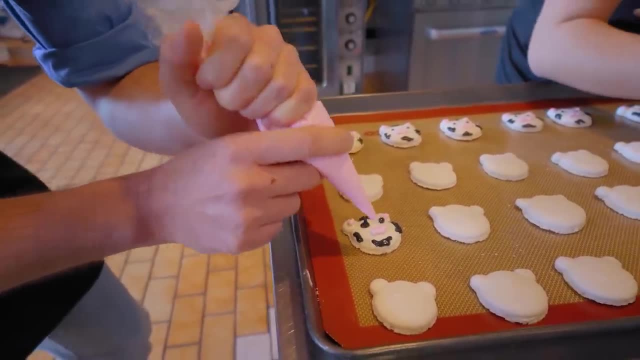 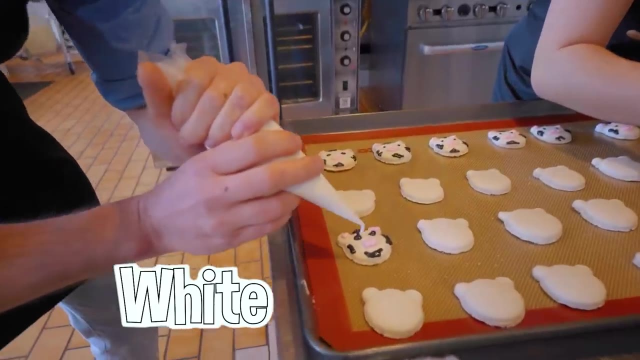 And it's the base for the nose. Last but not least, the color white, Haha, And we just put a little. Uh-oh, I put a little too much, But that's okay, There we go, Haha. 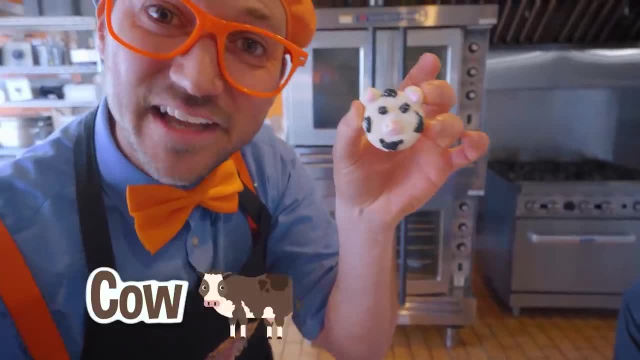 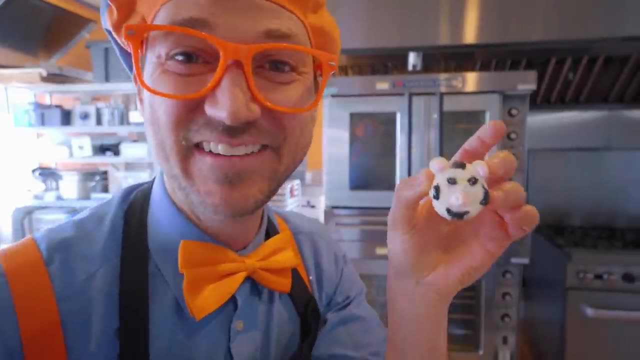 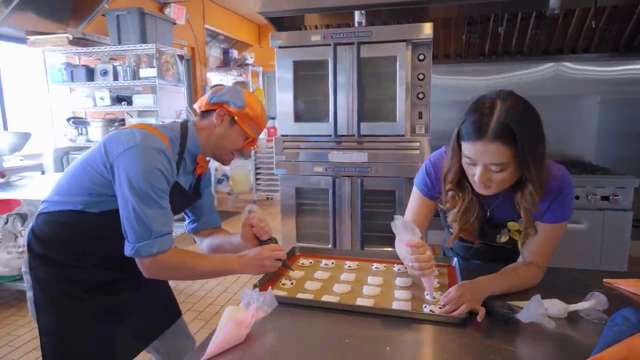 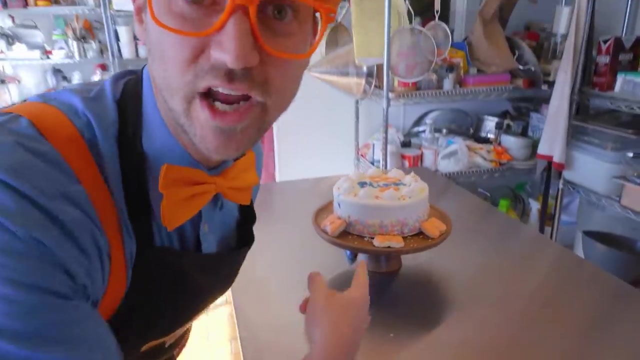 How does it look? Yeah, does that look like a cow? Moo Moo, Haha. Wow, That looks so good, Haha. Alright, Let's keep on decorating. Whoa, Check it out. Yeah, a Blippi party cake, Yum, Haha. 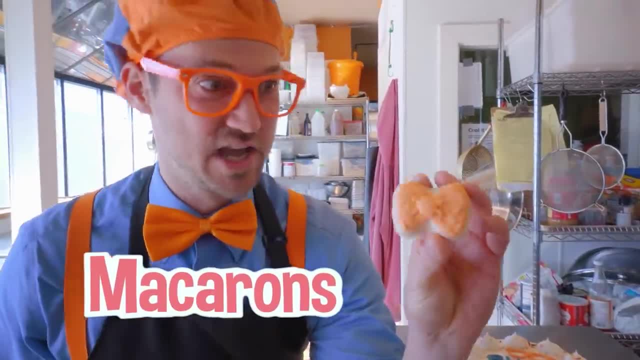 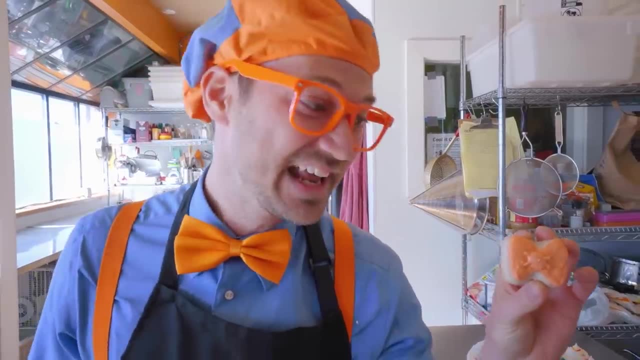 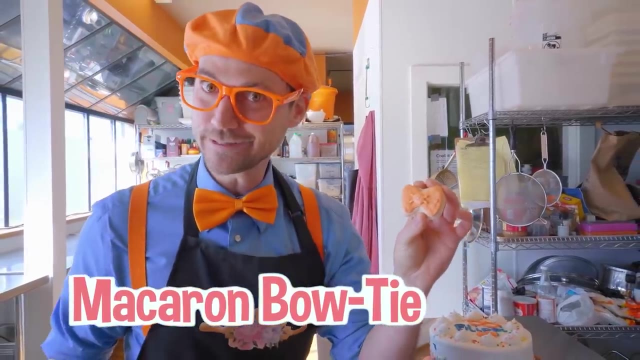 Whoa, What are these? Yeah, macarons. Yum, They're so tasty. What is this, though? Yeah, Does it look like my bow tie? Yeah, It's an orange Blippi macarons bow tie. And it looks so tasty, doesn't it? Yeah? 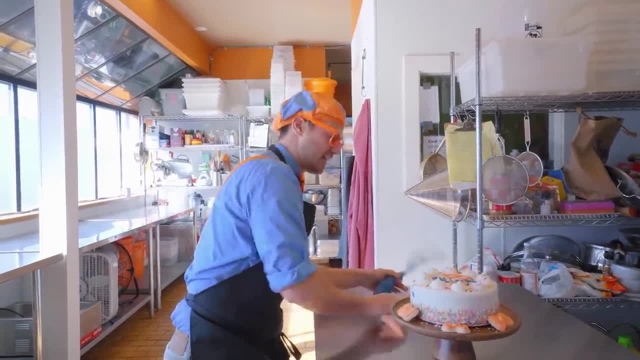 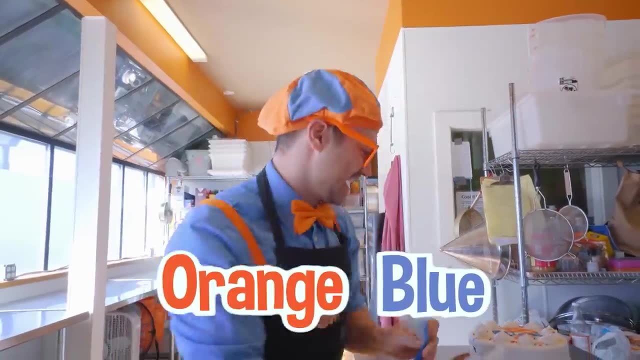 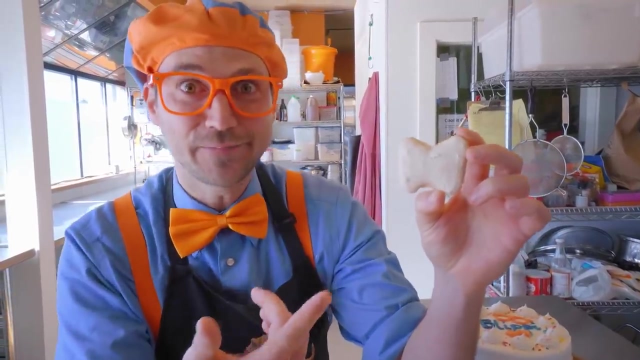 Well, hey, check this out. I have two things of Icy, My two favorite colors, Blue and orange- And check it out. I have a Blippi macarons That's empty, No colors at all, So maybe, just maybe. 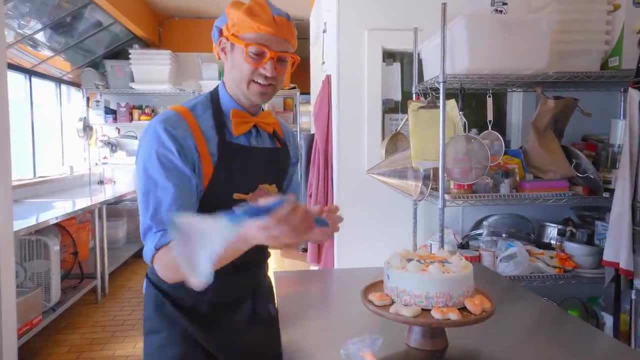 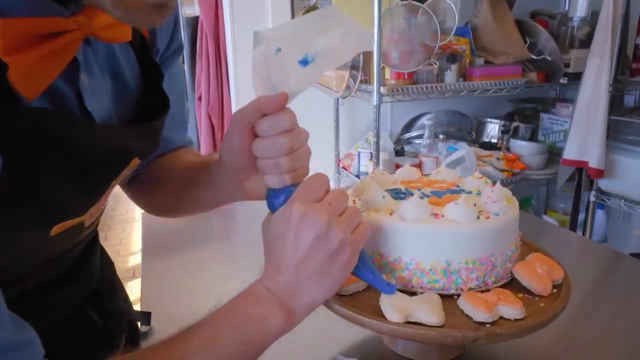 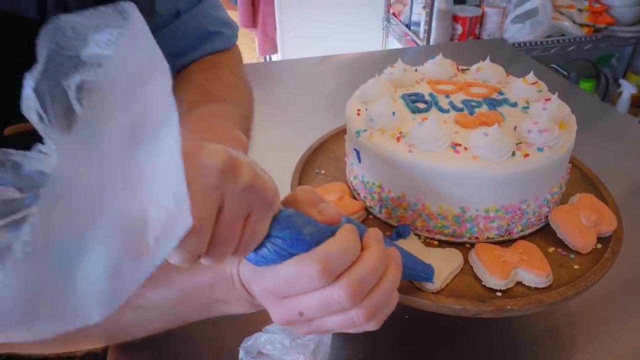 we can use some of this icing to decorate it. So my normal bow tie is orange, But I'm actually going to use some blue too, So let's just squirt some out. Whoa, That looks cool. Let's do a big dot there. Do a big dot there. How about one right there? 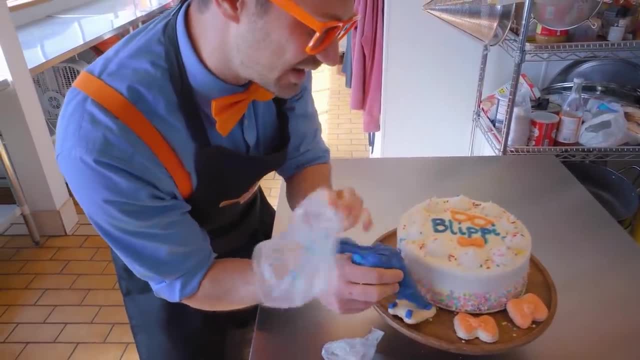 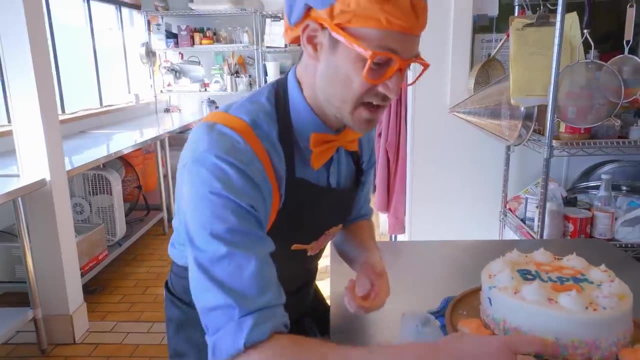 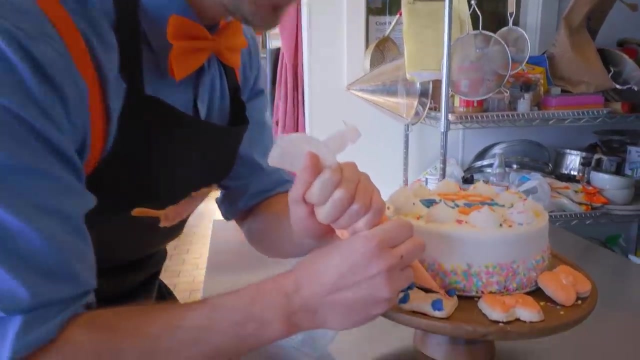 Oh, and one way over there. Whoa, That doesn't look like my bow tie, does it? No, That's okay, though. Sometimes, when you're being creative- yeah, actually all the times when you're being creative- you can do whatever you want. 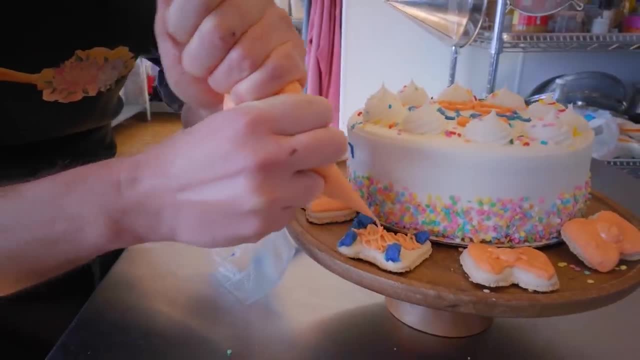 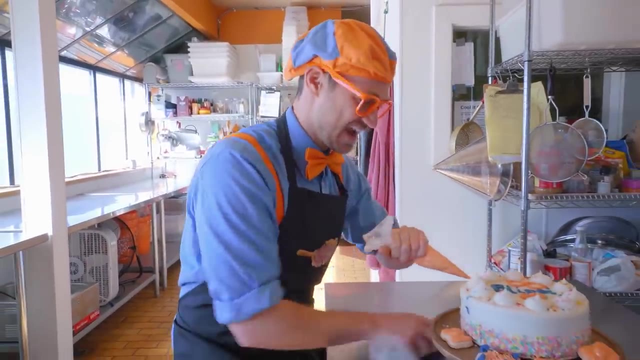 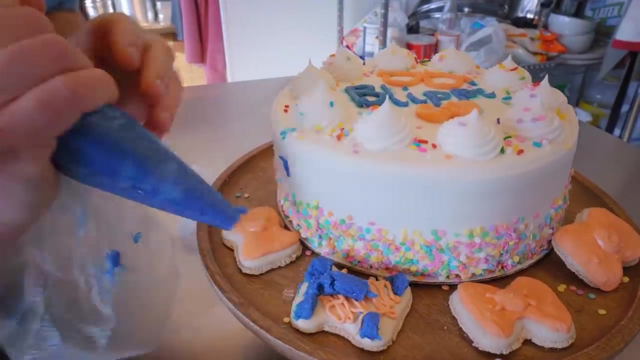 Yeah, like this. Woohoo, Check it out. Whoa Yum, Doesn't that look tasty, Yum. And hey, watch this. I'm going to do another big blob. Yeah, a blue. I will just finish that all the way across there. 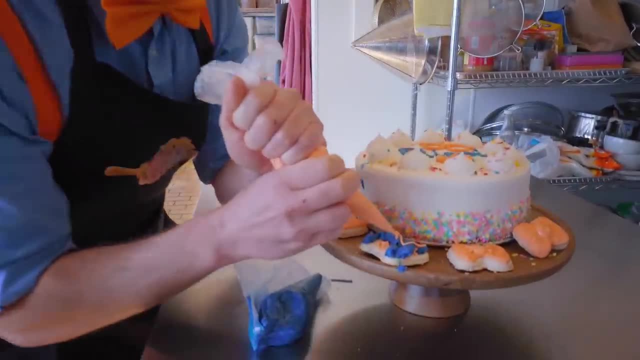 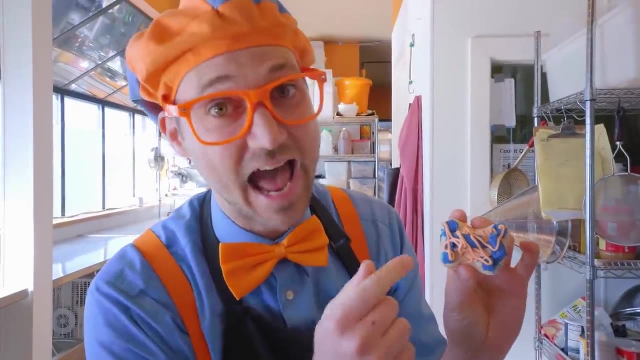 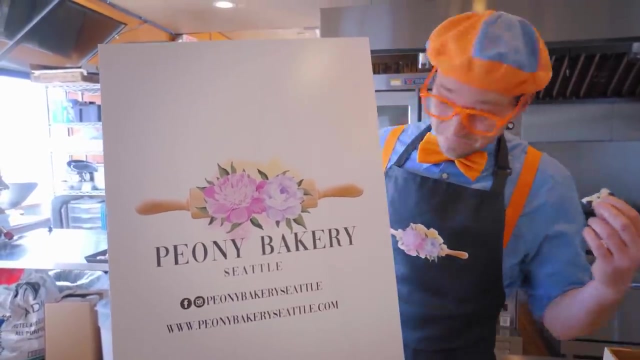 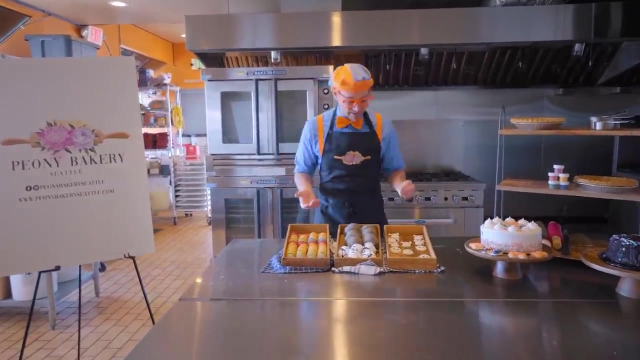 And then I'll put some orange on top of that. Wow, Now does that look tasty, Or does that look tasty? Yum, Mmm, These are so tasty, Whoa, That has been so much fun Making all these sweet treats with you, hasn't it? 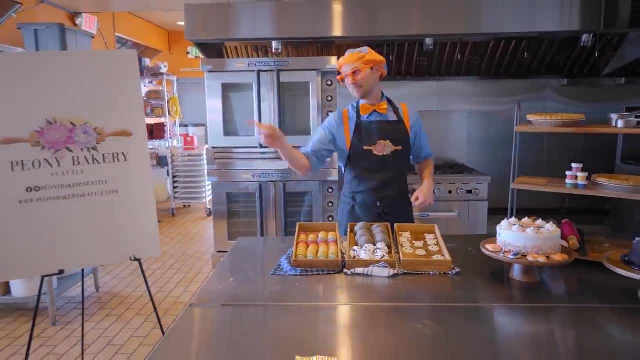 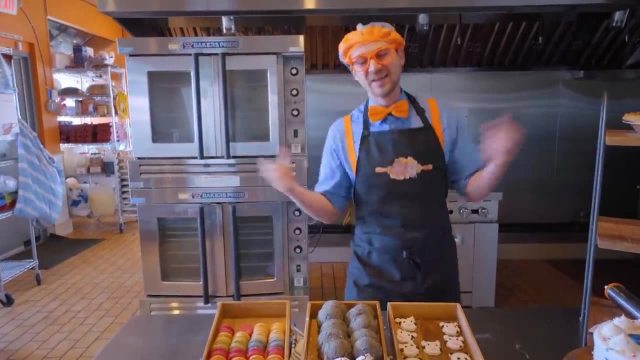 Yeah, I want to give a special thanks to Jennifer at Peony Bakery in Seattle, Washington. Wow, She did such a good job and they are so yummy. Well, this is the end of this video, but if you want to watch more of my videos, 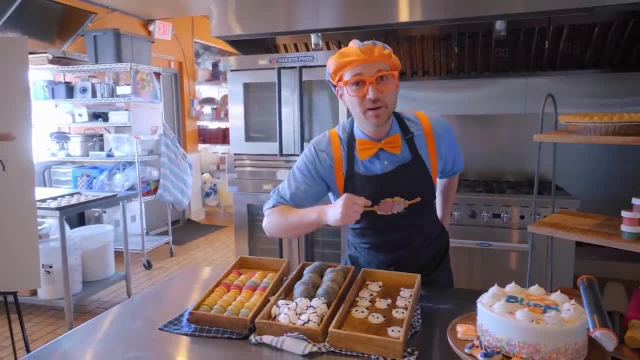 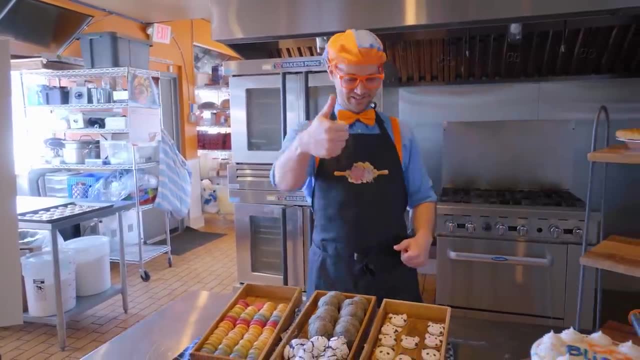 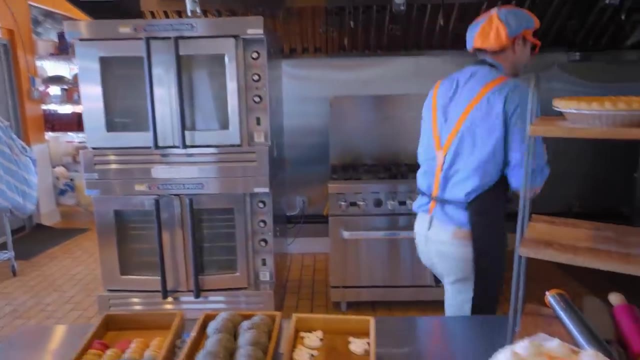 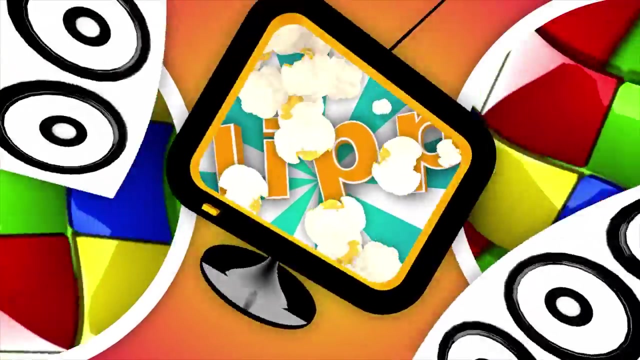 all you have to do is search for my name. Will you spell my name with me? Ready, B-L-I-P-P-I, Flippy. Good job, All right, See you again. Bye-bye. So much to learn about. It'll make you want to shout. 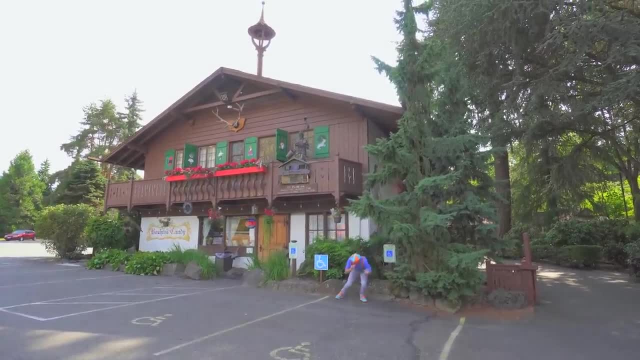 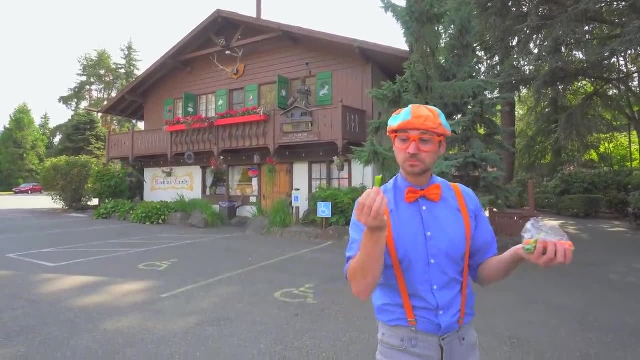 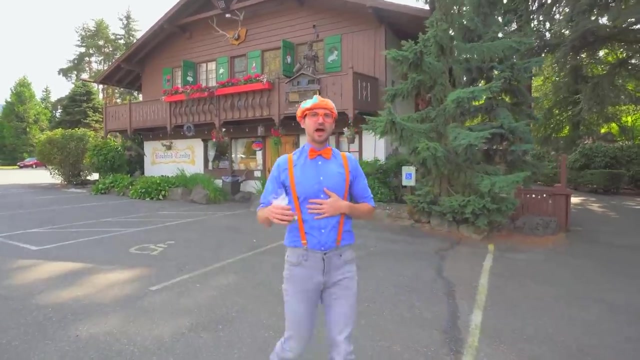 Flippy- Hey, It's me Flippy. Ooh, And look at what I have. Mmm, Some tasty vegetables. They were really healthy, But I'm really full. now and after you eat a nice healthy meal. 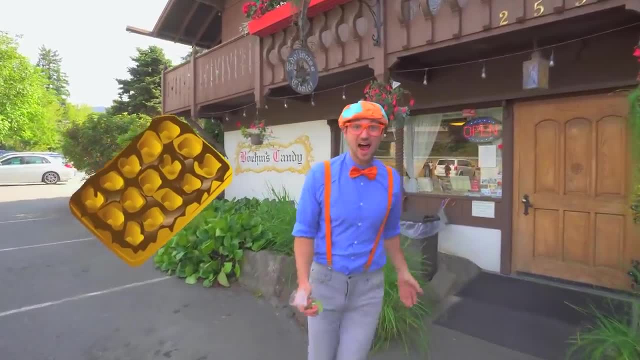 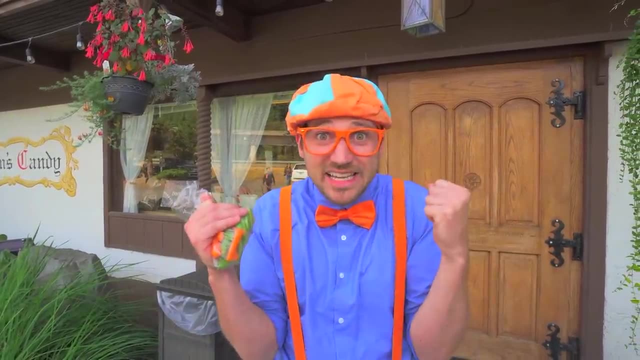 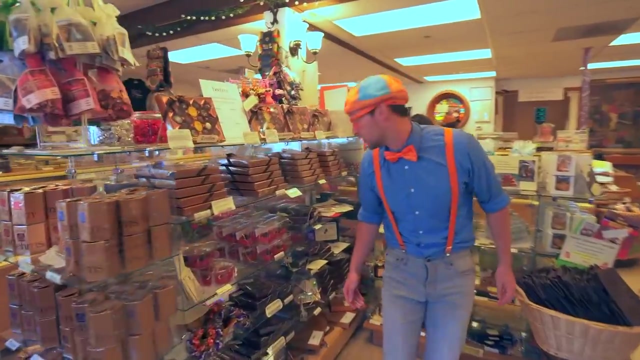 guess what you get to eat next? Yeah, Dessert. And today we are at Boom's Candy in Issaquah, Washington. This is going to be so tasty. Come on, Ooh, Look at this place, Yum. 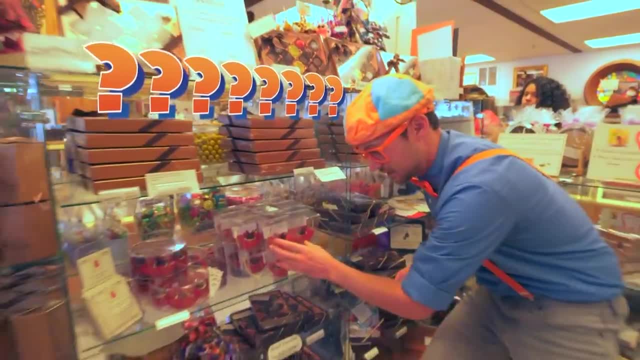 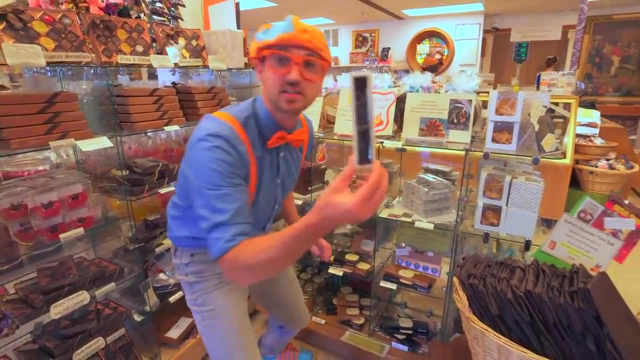 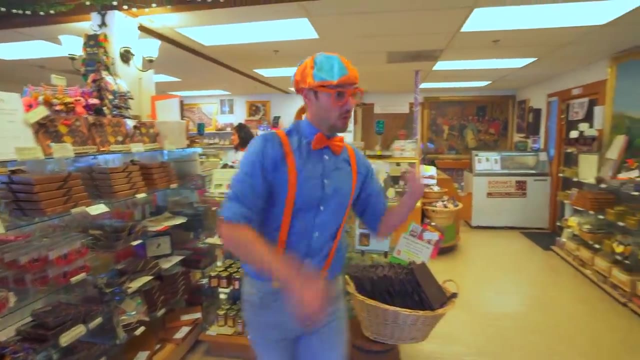 Oh, I don't even know what that is, but it looks so good. Whoa Hey, Some caramel. Ooh, Some chocolate. Yum, Hey, I think we should learn how to make some of these tasty treats, Woo-hoo. 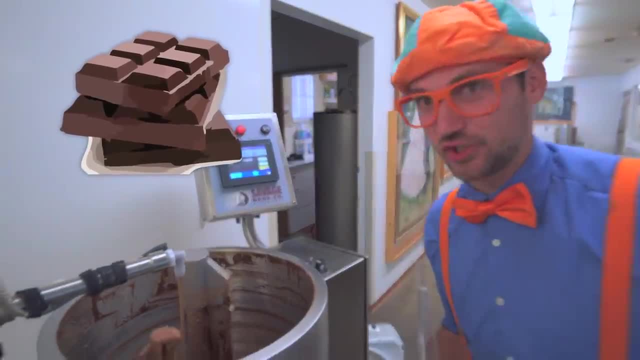 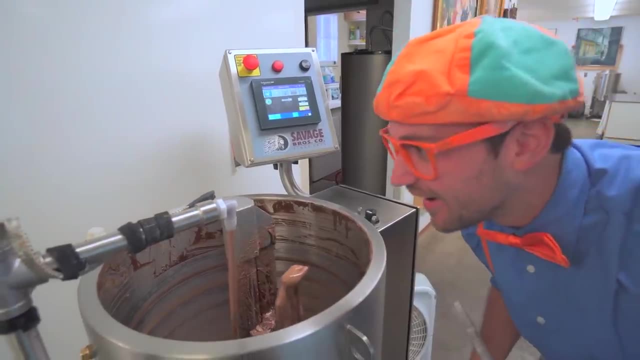 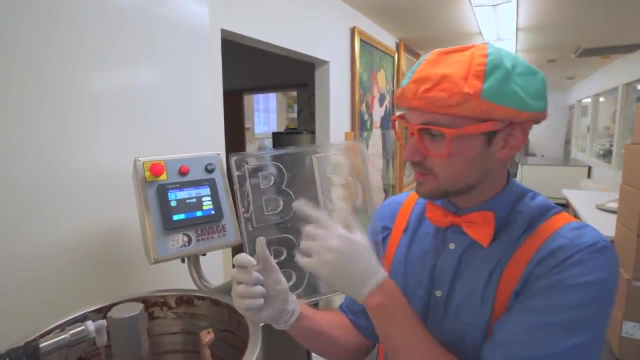 Ooh, Chocolate, chocolate, chocolate. I sure do love chocolate. Hey, Look at it. Look at it. come out of the spout right here. Do you see, Whoa? And look at what I have? Ooh, A plastic thing that has some letters on it. 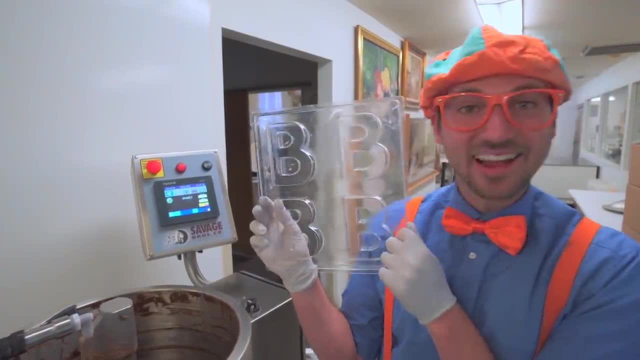 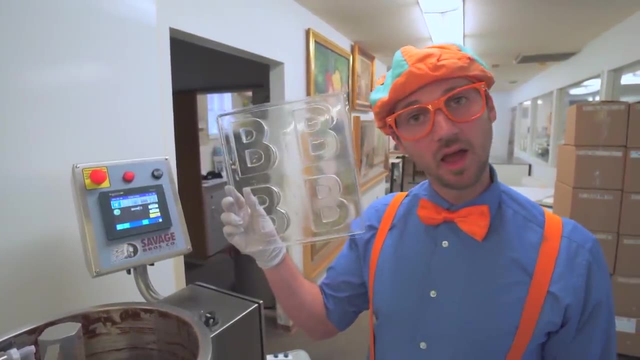 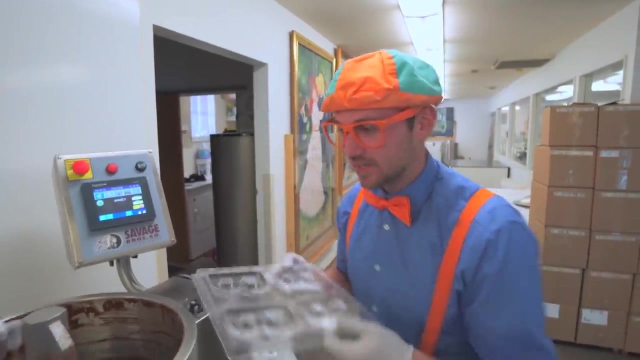 Do you know what letter this is? Yeah, It's the letter B. Do you know someone's name that starts with the letter B? Yeah, My name does Flippy. Hey, I have an idea. Let's fill up one of these B's with. 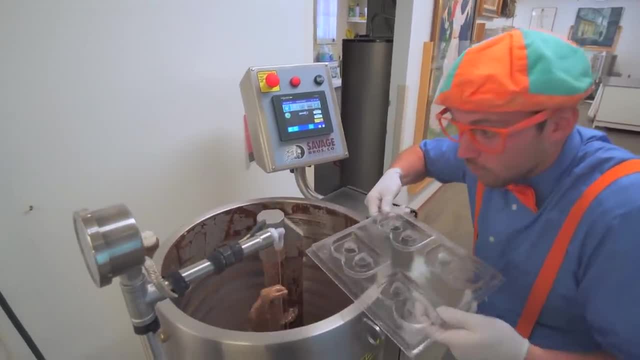 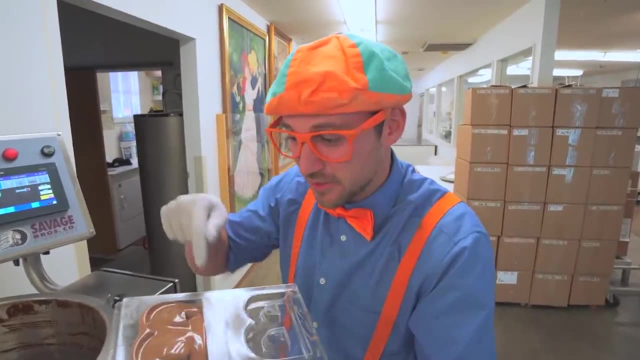 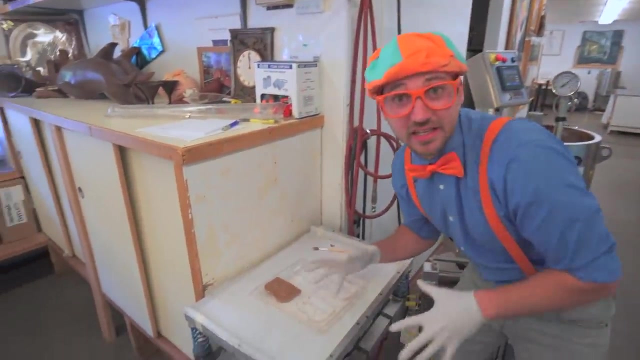 warm chocolate Ready. Whoa, Whoa, Whoa. Look at it, It just squirted a bunch of chocolate right there. Okay, now we need to take it right over here and we need to shake it and get all the air bubbles out of it. 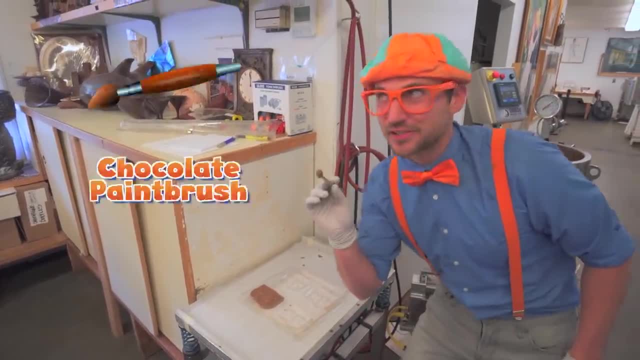 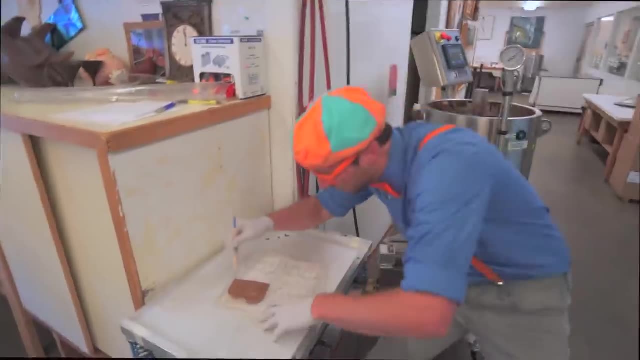 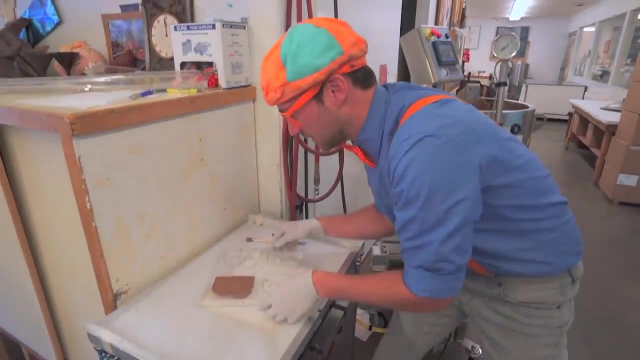 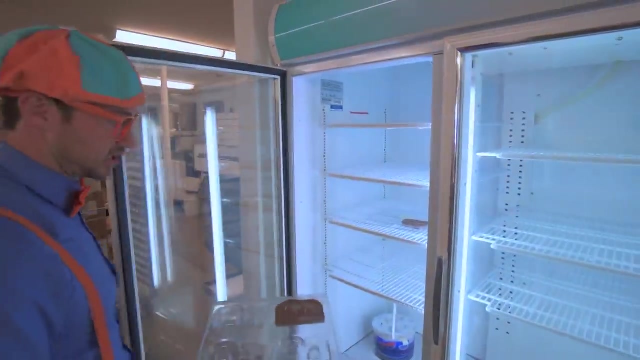 And use this chocolate paint brush Or a chocolate brush. Okay, Turn it on. All right, Now that all of the air bubbles are out of here, let's put it in the fridge. Hey, Do you know why we're putting it in the fridge? 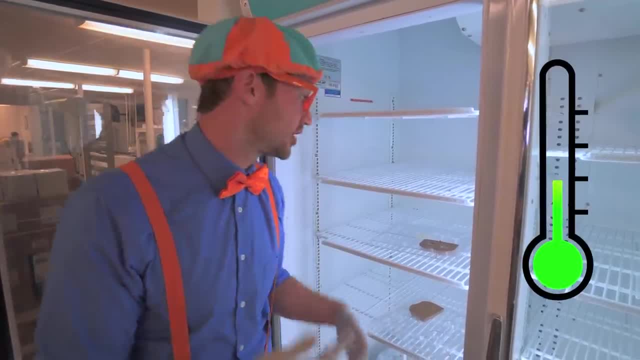 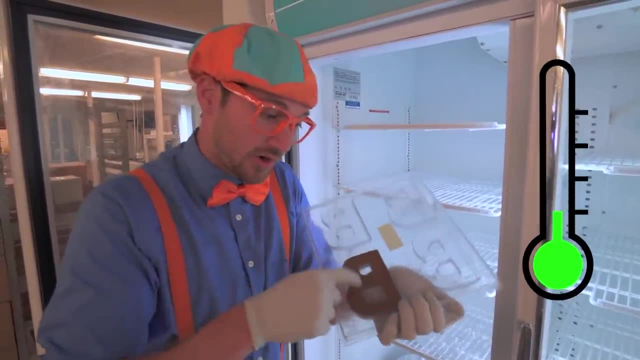 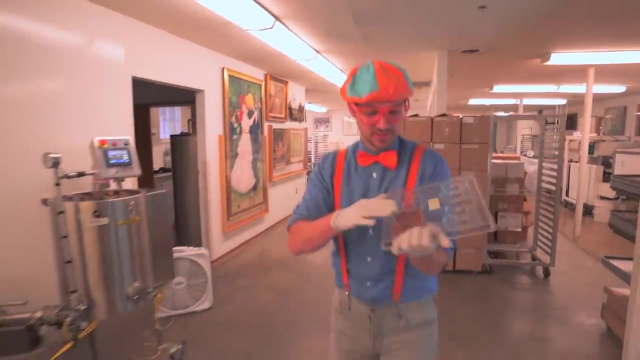 Yeah, Because remember earlier I said the chocolate is really warm and we need to cool it down. so then it gets nice and hard. Chocolate is hard when it's cold. See, No chocolate on my fingers. All right, Now the next step. 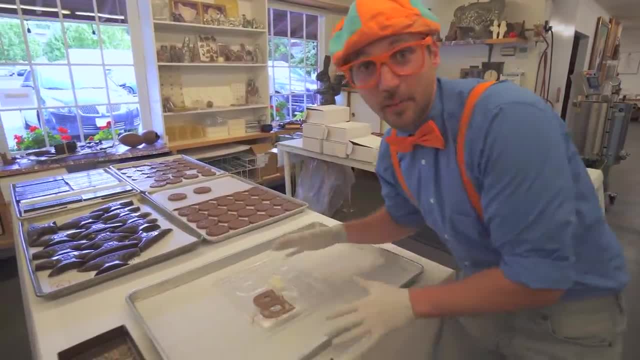 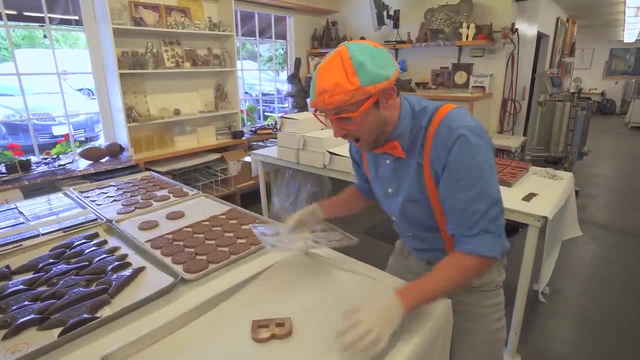 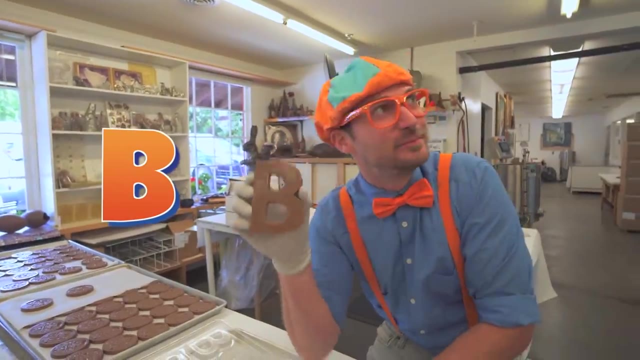 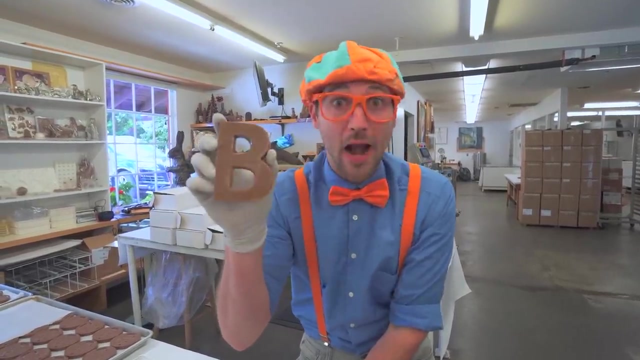 Put it on this tray and we need to pop it out. Okay, Here we go. Yeah, Look A chocolate, B, B. What other words can we think of that? start with the letter B: Um Brown, Yeah, This chocolate is the color brown. 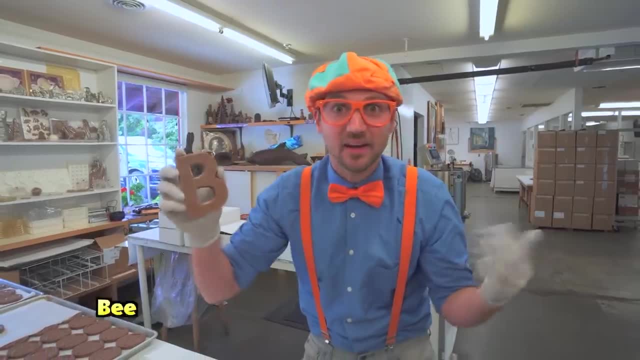 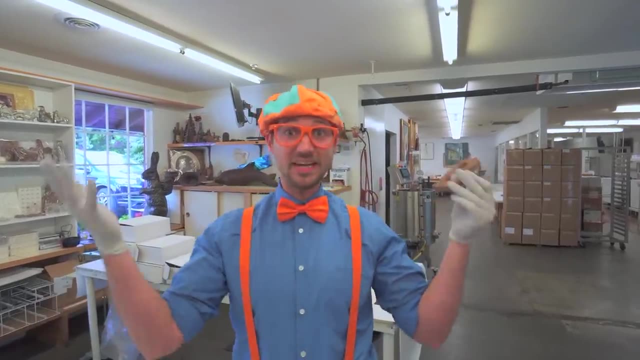 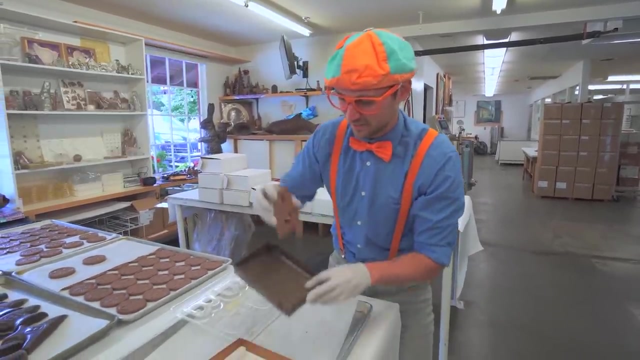 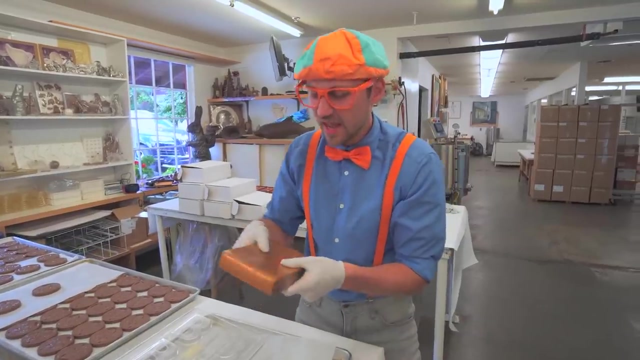 What about B? Whoa, Whoa, Yeah, Like a bumble bee. Okay, Let's put it in this box. Box also starts with the letter B. Okay, Bye-bye B, There we go. Hey, Speaking of boxing up chocolate, check it out. 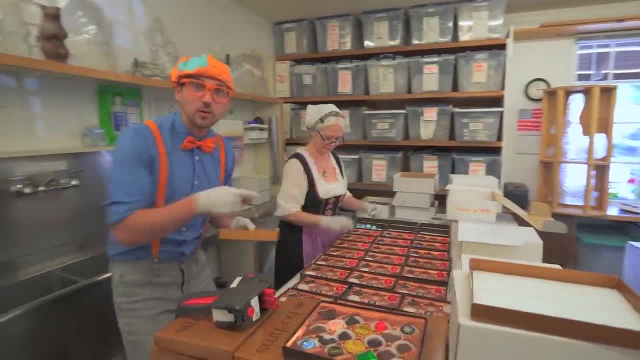 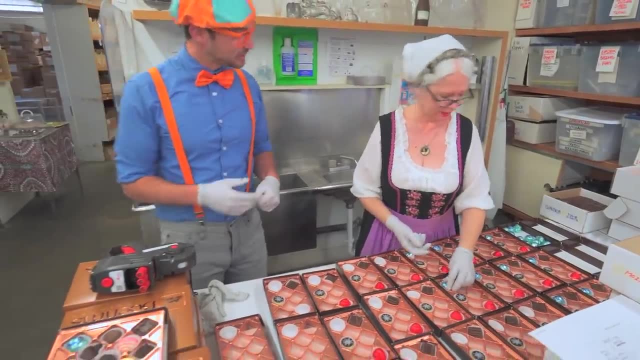 Okay, Ooh Whoa. Look at what she's doing. She's putting a lot of chocolate in all of these boxes. Wow, Good job. Thank you, sir. Are you having fun? Oh, Blippi, I'm having a lot of fun, I really am. 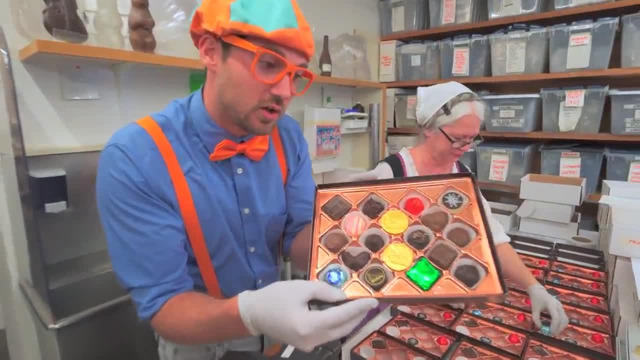 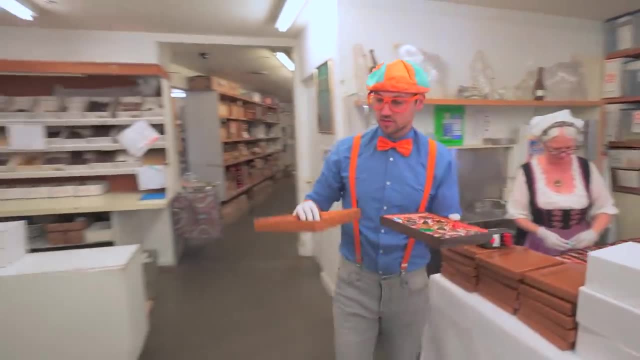 Cool. Well, this is what it's going to look like when she's all done. Isn't that beautiful? It sure is Okay. Now let's complete the process. So we need to take this box of chocolates, put this pad on top. 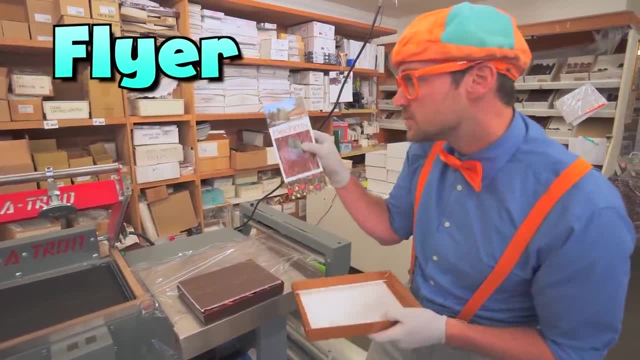 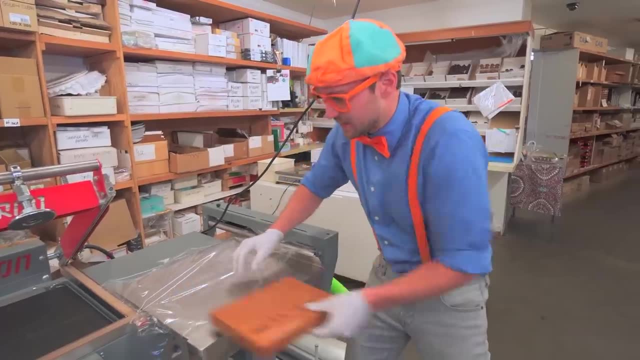 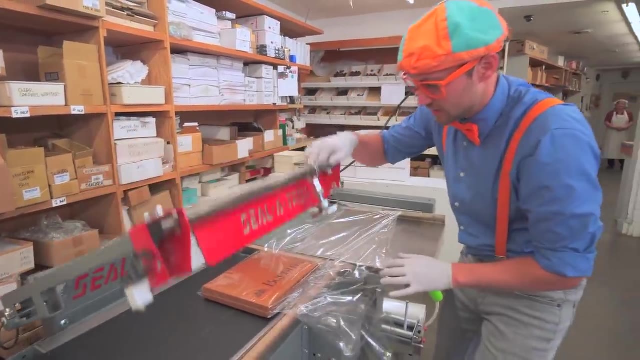 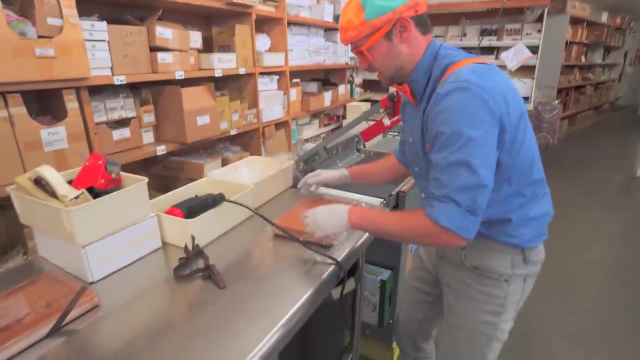 and then this flyer Bones Chocolates. Put it right on top. And then let's put the top of the box on, slide it inside the plastic, push it onto the conveyor belt, shut it. Ooh, Perfect, Okay, Now we need to take this heat gun. 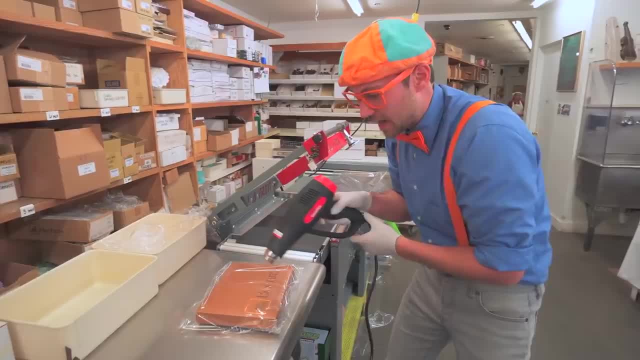 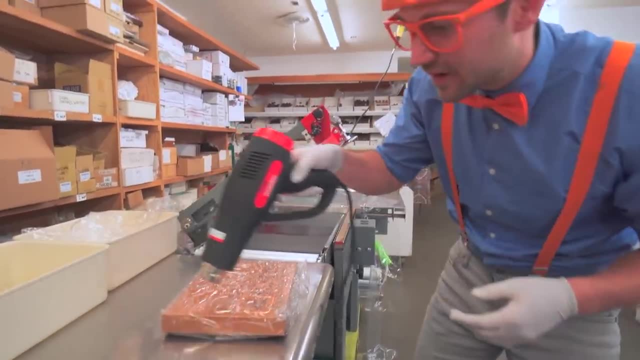 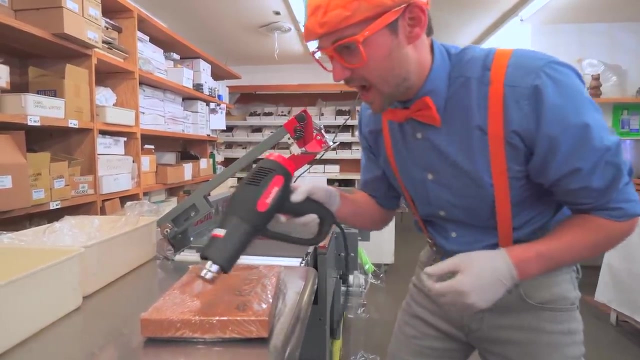 and this is called shrink wrap. It tightens up the plastic, It makes it nice and tight. There we go. Oh, this is kind of fun. Whoa, Whoa. Yeah, That's looking real good. Okay, There we go. 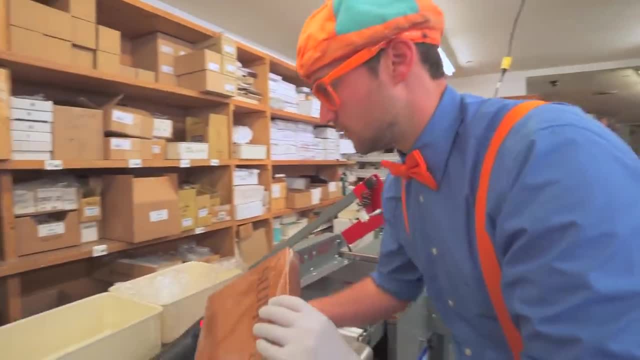 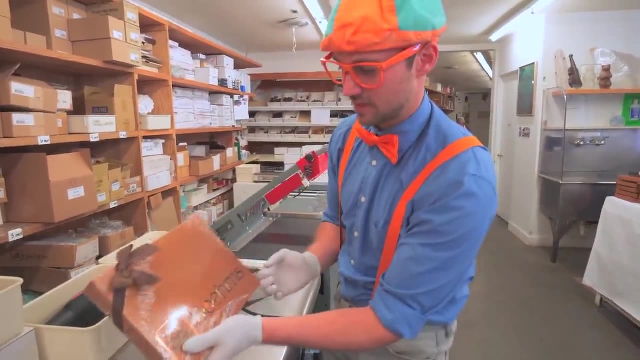 Let's flip it to the back And then, once it's nice and warm and tight, then you put on a bow. Yep, Just on the top, Then on the bottom And voila See, You got a beautiful box. 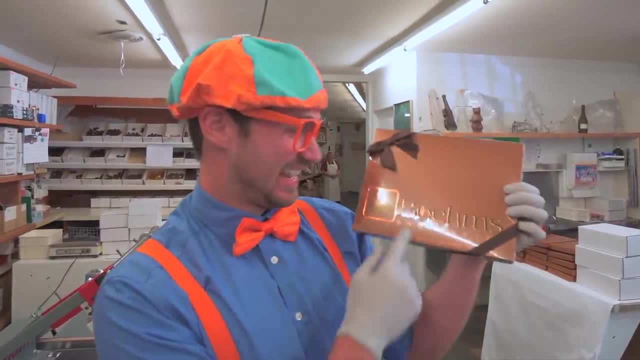 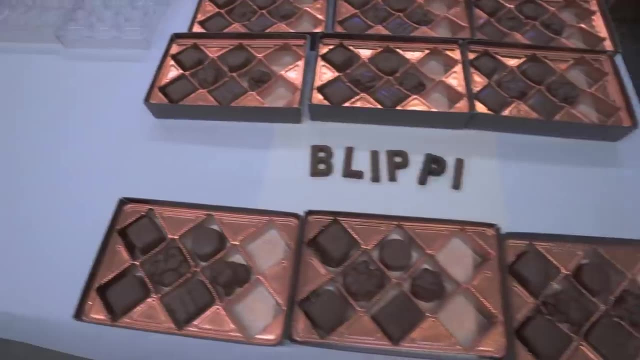 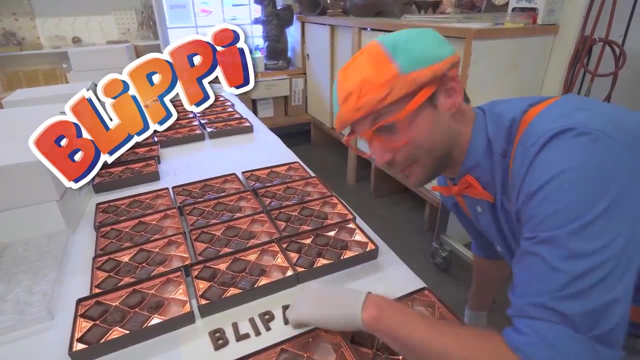 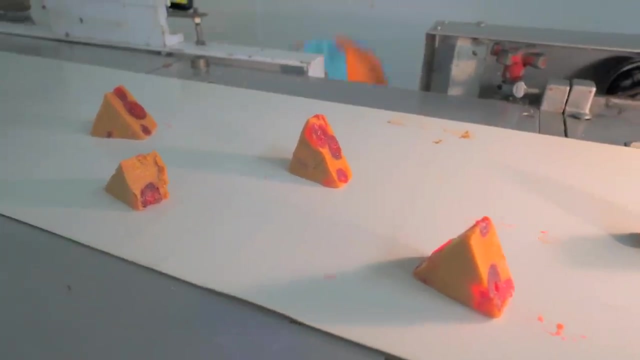 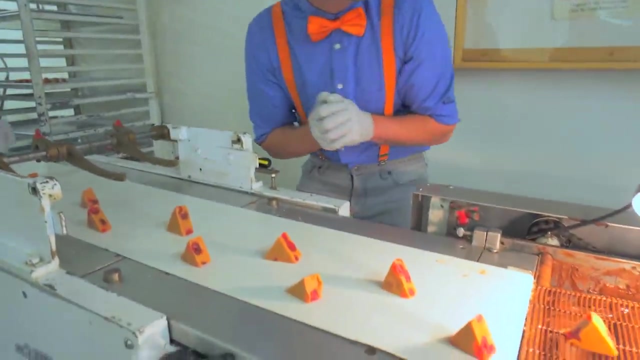 Beautiful and box Start with the letter B, And Bones does too. Now I can take it home. Woo, Ooh, B-L-I-P-P-I, Blippi Woo, This candy looks so tasty. Oh, It's on a really long conveyor belt. 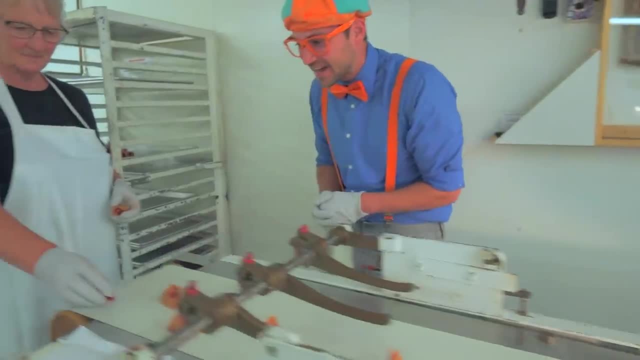 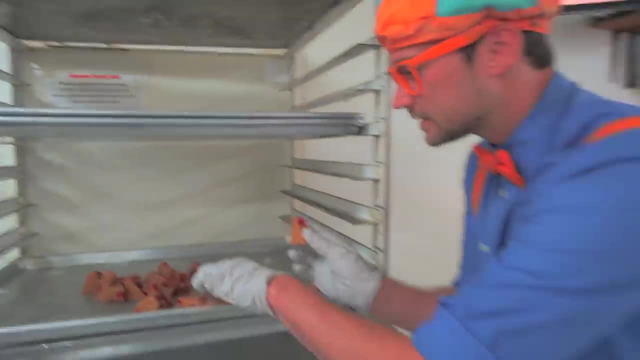 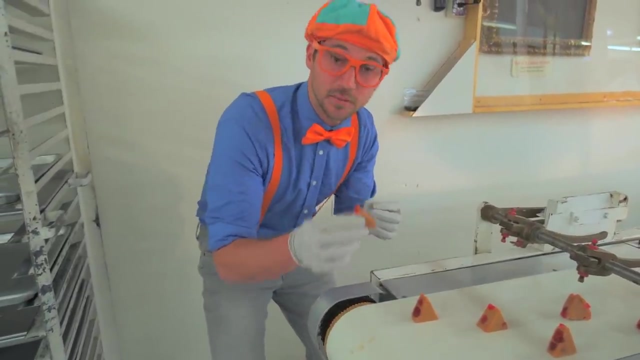 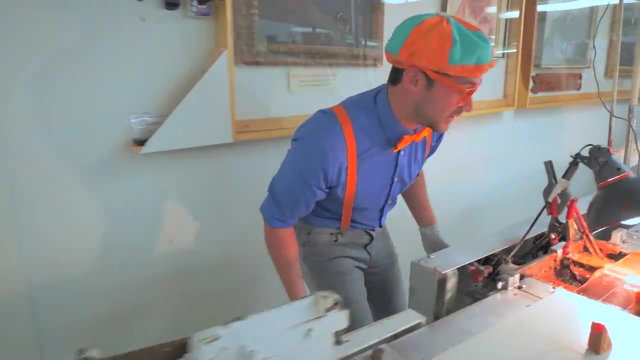 I wonder how it works. Oh, Can I try? Sure, Look over here. Let's take two pieces, Let's put one piece there And let's put the second piece right there, And then it goes down this really long conveyor belt. 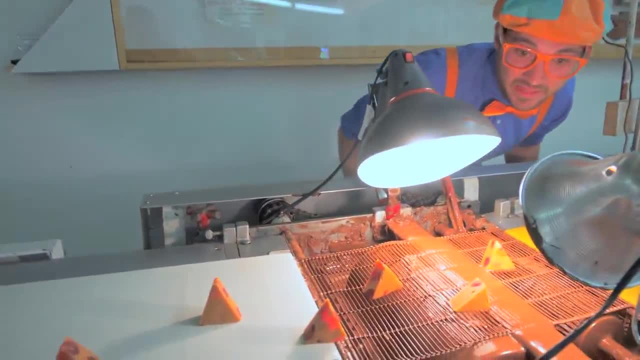 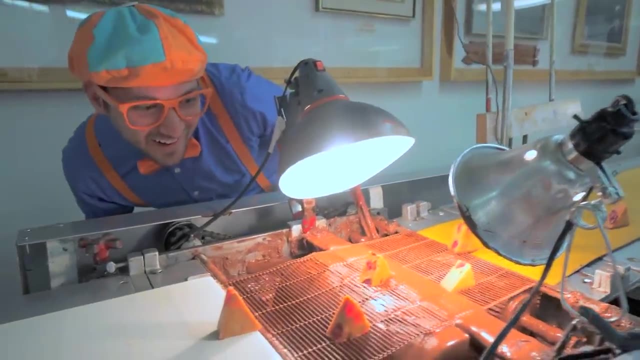 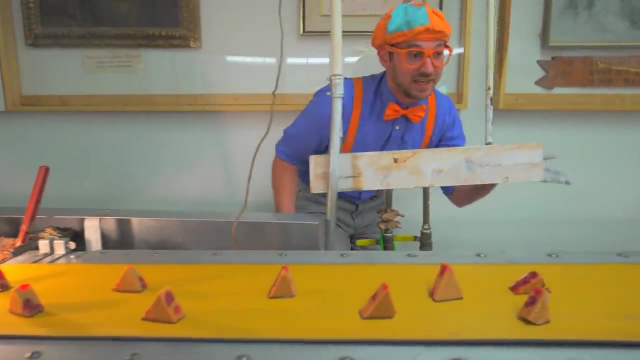 Oh, And this adds chocolate to the bottom. Wow, That's cool looking. Ooh, And then it dries a little right here And it goes really slow. Do you see how slow it's moving? Oh, hey look. 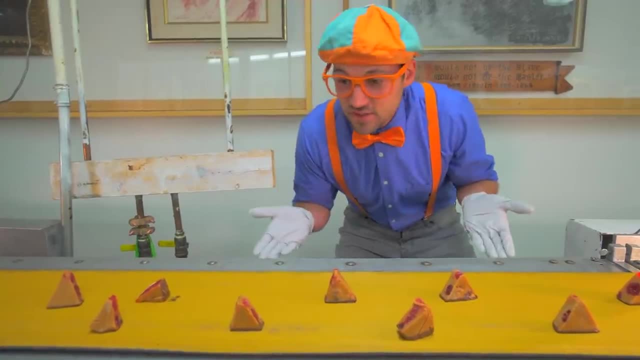 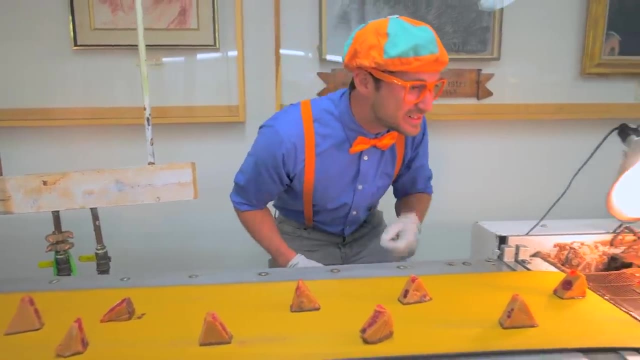 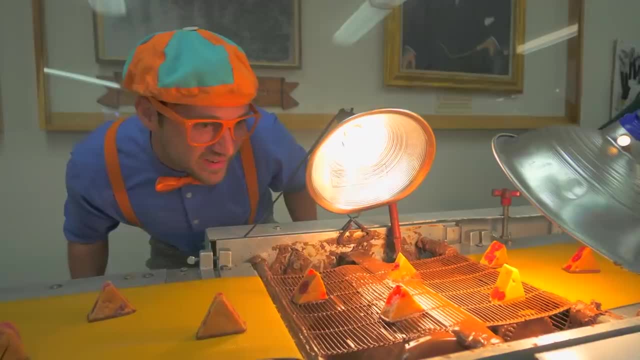 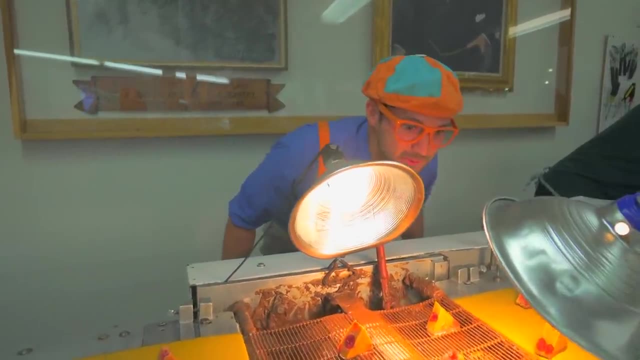 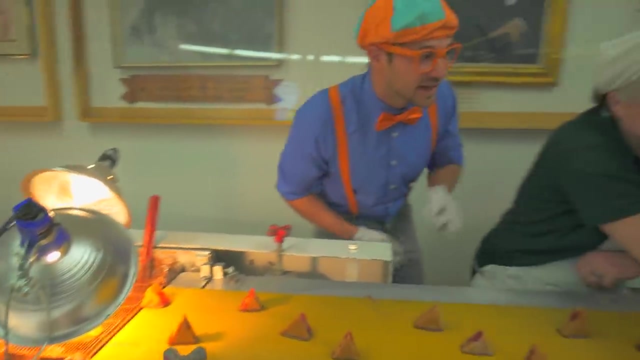 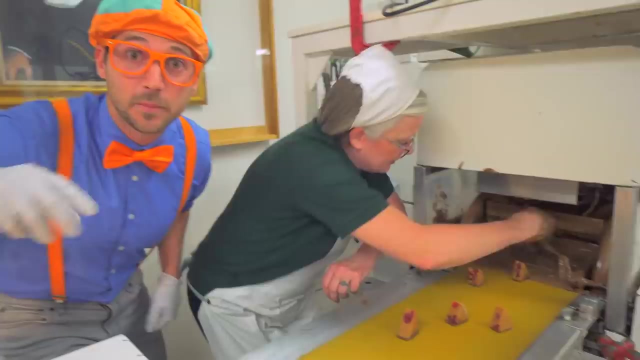 Wow, That's really fascinating to watch. Now that there's two layers on the bottom, the next part is right here. What are you doing? I'm covering the mountaineers with a lot of chocolate, so there's no holes, So they're putting a lot of chocolate up top. 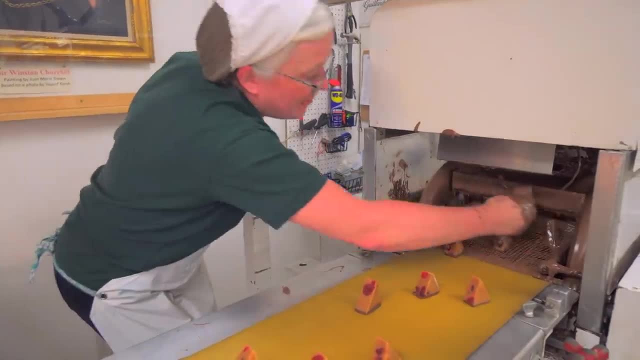 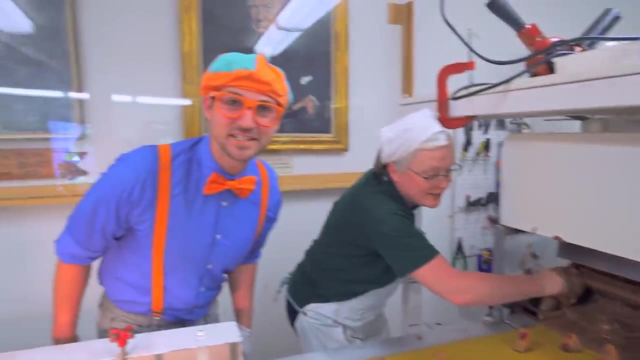 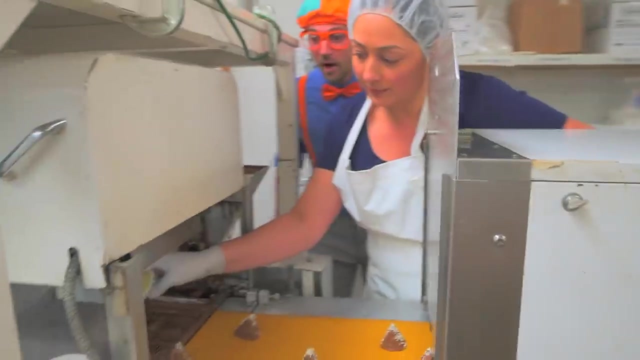 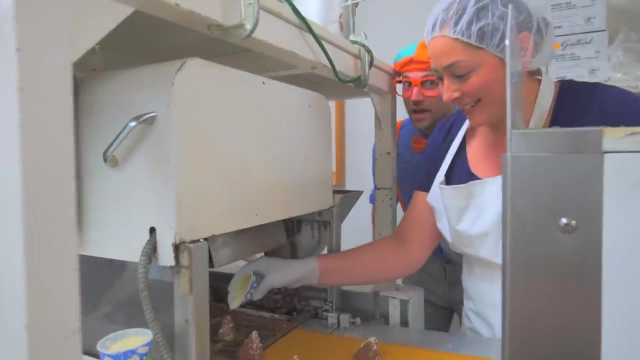 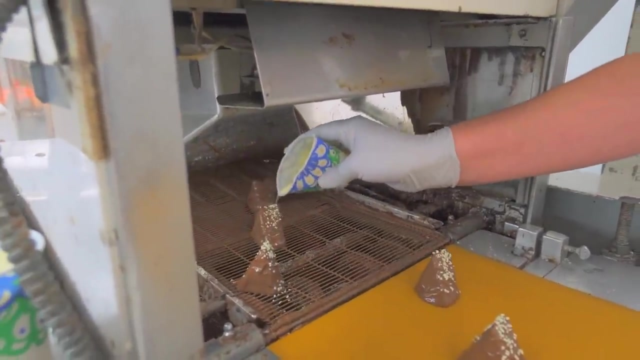 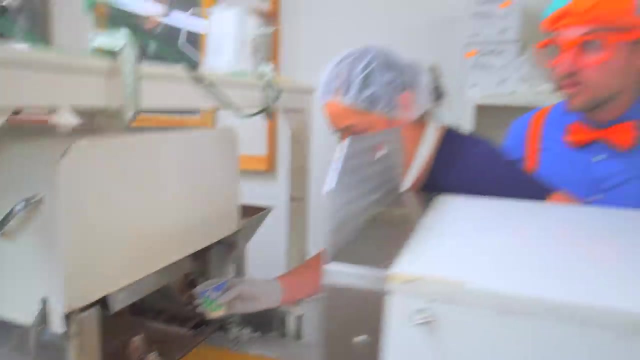 Whoa, look, That looks tasty. Meet me on the other side. Whoa, What are you doing? I'm adding white chocolate snow to the Mount Rainier. Ooh, check it out. White chocolate snow. Whoa, Whoa, it's looking tastier and tastier. 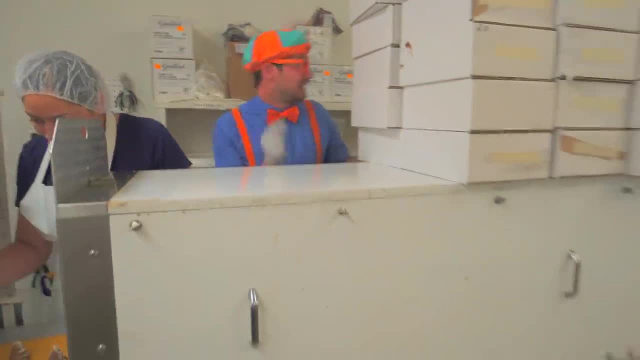 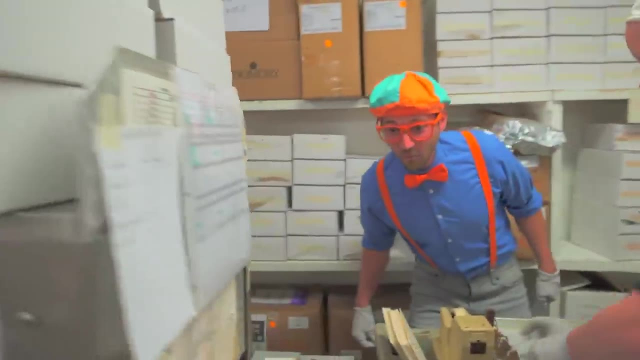 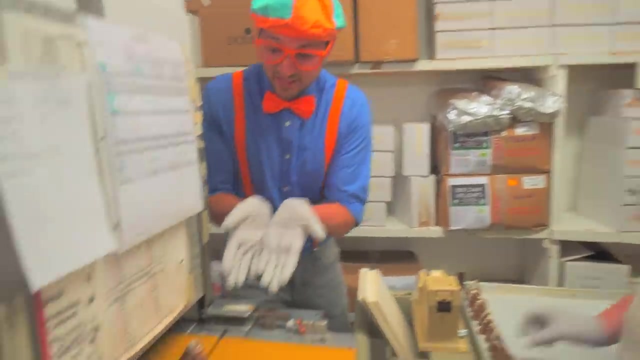 And then, right here, it cools down And then meet me over here. Ooh, What are you doing? Putting these on, putting these chocolates on the tray? Ooh, These chocolates that are complete now go on the tray. 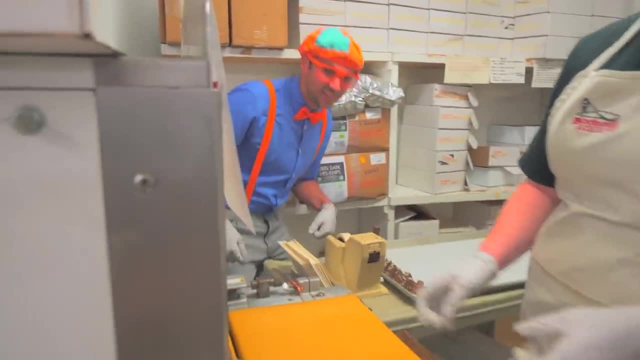 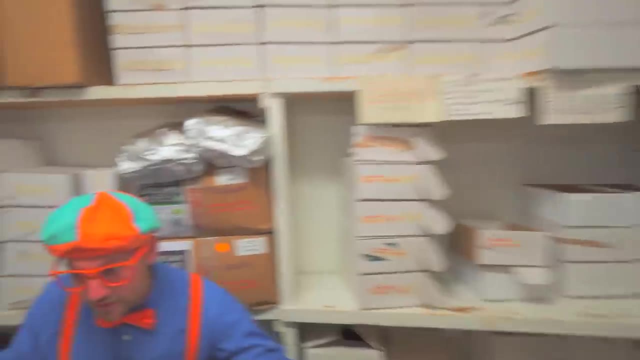 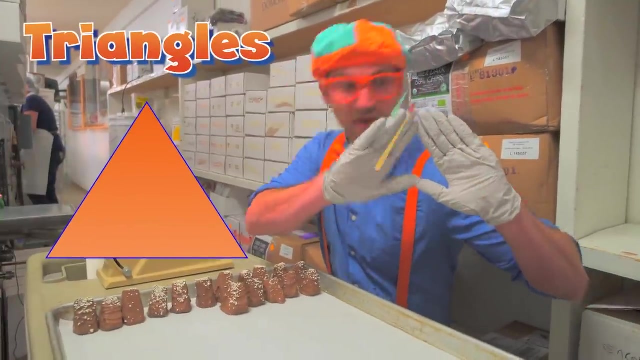 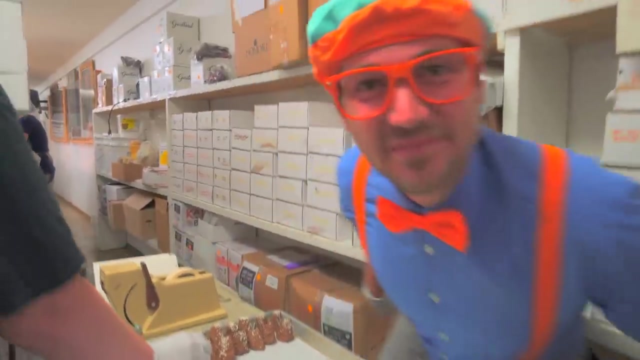 Watch Whoa, Wow, Check them out, Yum, Look at them. They're like little triangles with some snow on top, Just like Mount Rainier. Wow, Yum, Ooh. look, I have some chocolate in this plastic tube. 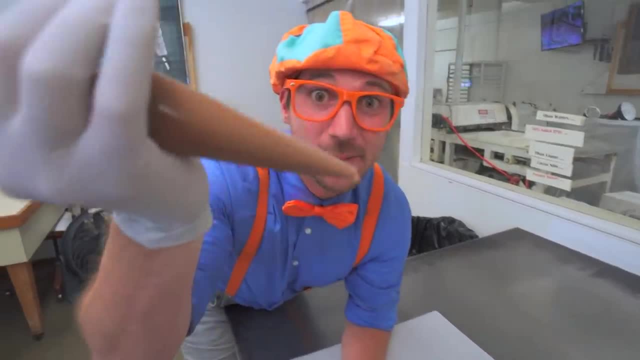 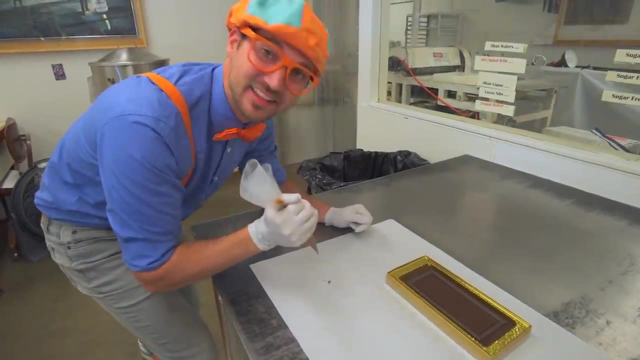 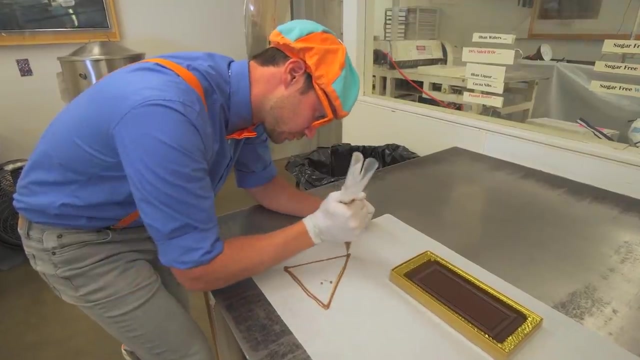 I cut the bottom off And now I can make a masterpiece Ready. Um whoa, It's coming out. Okay, let's draw a triangle. Oh, There we go. Good job. Now how about a rectangle? 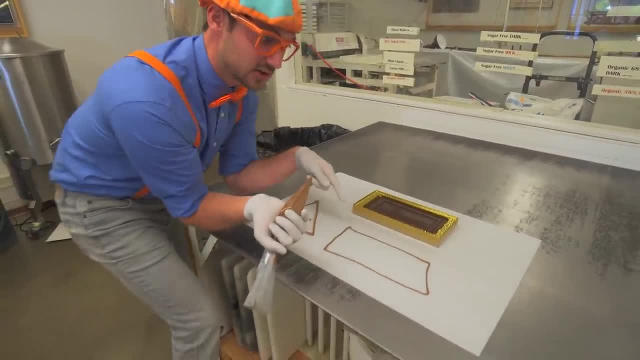 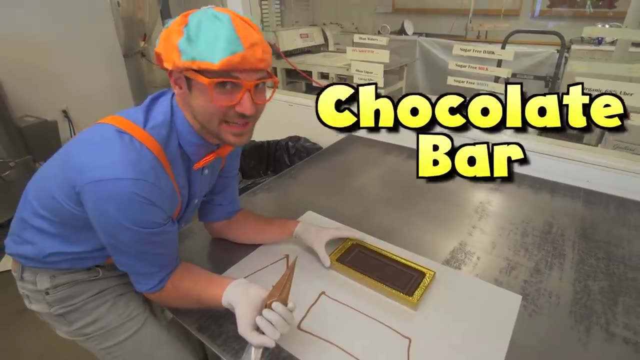 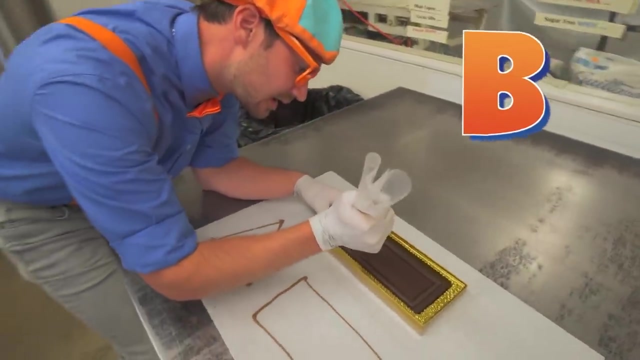 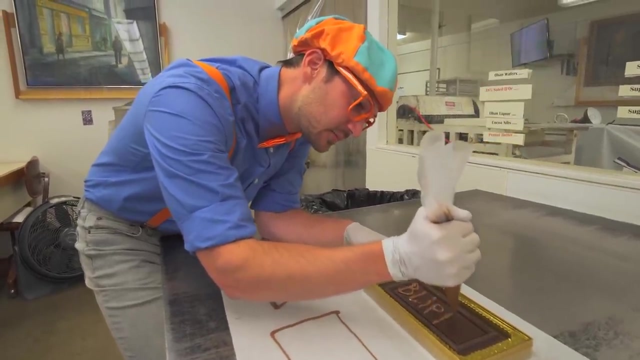 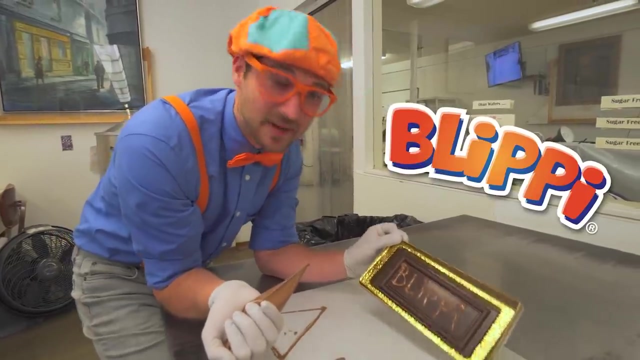 Ooh, That rectangle kinda looks like a chocolate bar. Hey, Here's a chocolate bar. Let's spell my name together: Ready B, L, I, P, I, P, I. Yeah, Look, Blippi, That looks tasty. What else can we draw? 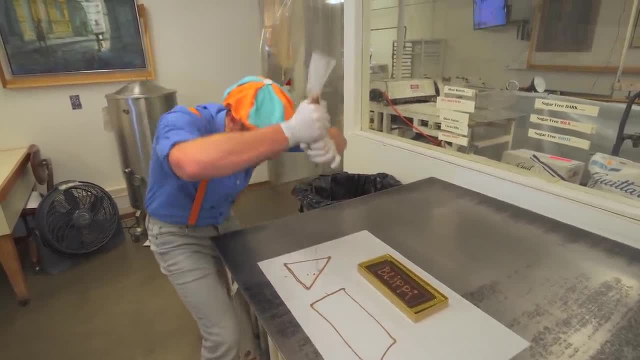 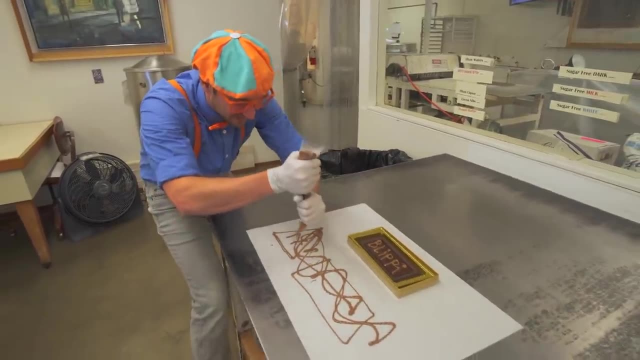 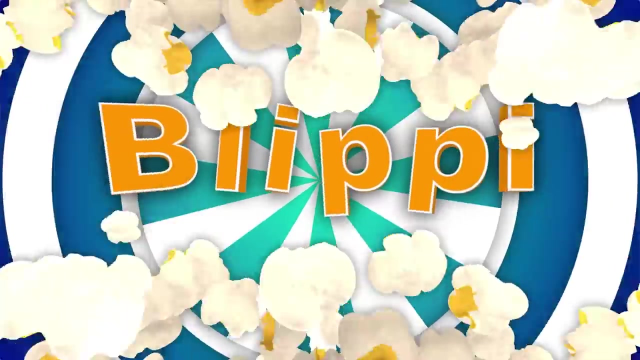 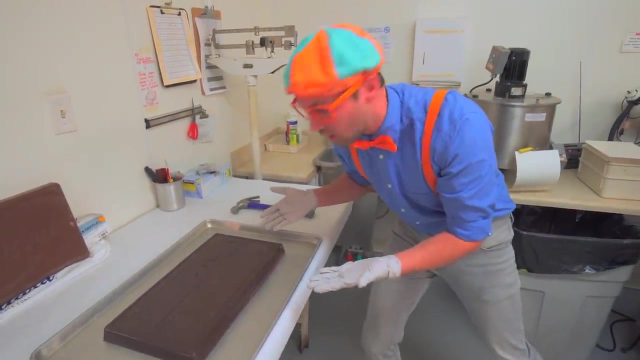 I know A bunch of squiggly lines: Whoa, Whee, Whoa. There we go. When that dries it's gonna be super tasty. Whoa Whoa. Look at this, This is a giant bar of chocolate. 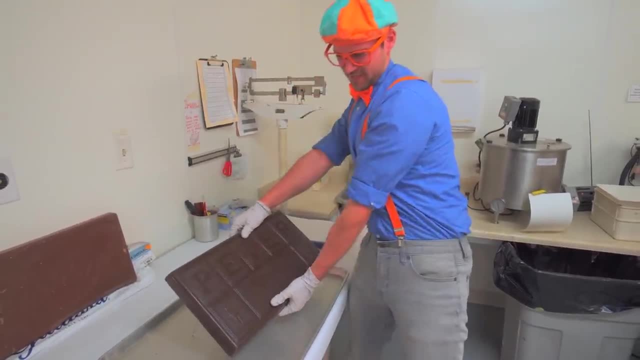 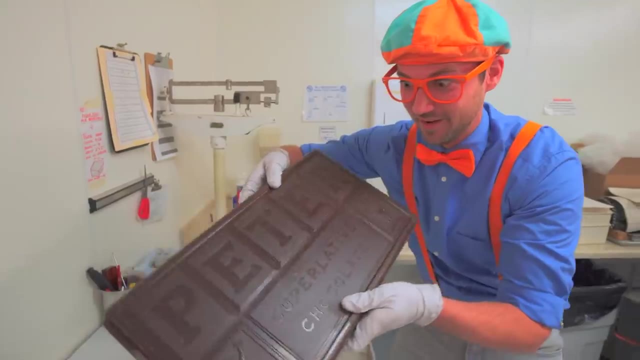 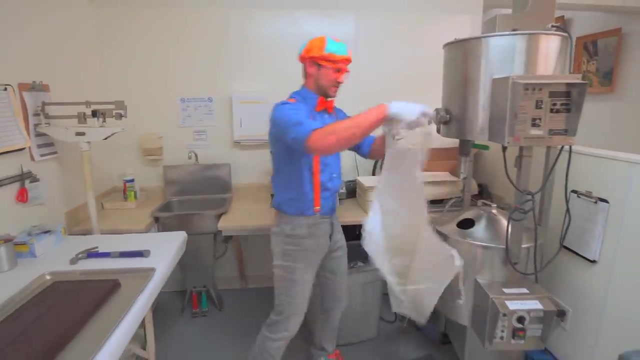 Whoa, It's really heavy. Whoa Jeez, Have you ever seen a bar of chocolate this big? I sure haven't. Okay, what I'm about to do is gonna get really messy, So the first thing we have to do is wear an apron. 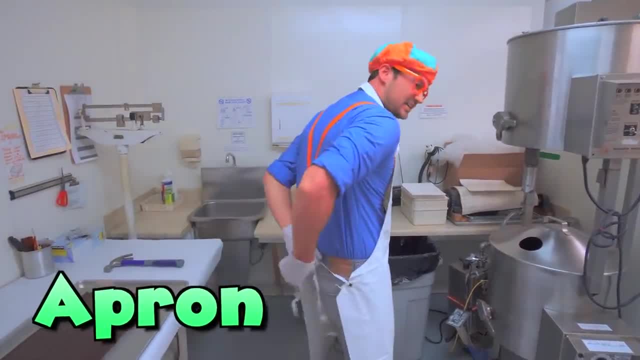 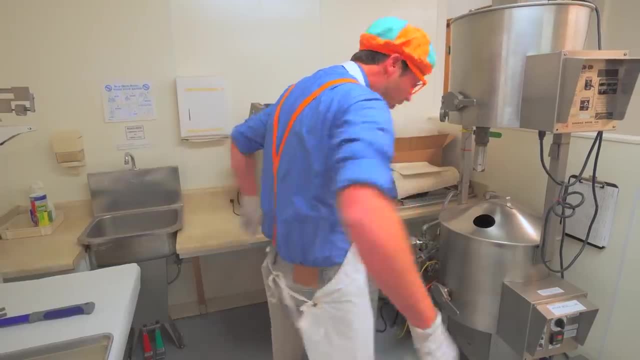 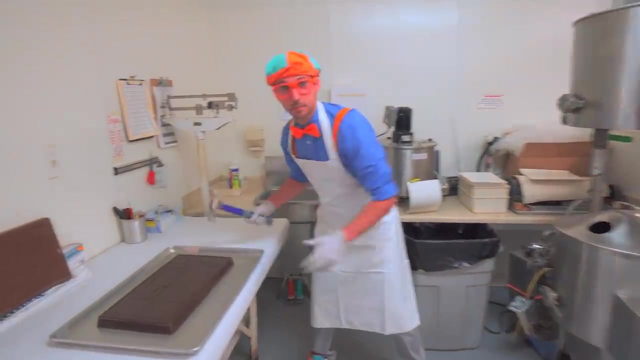 Perfect, Let's tie it on the back. Ooh, Now that I have an apron on woohoo, We can smash this bar of chocolate. But hey, this looks like a hammer, right, But this isn't a normal hammer. 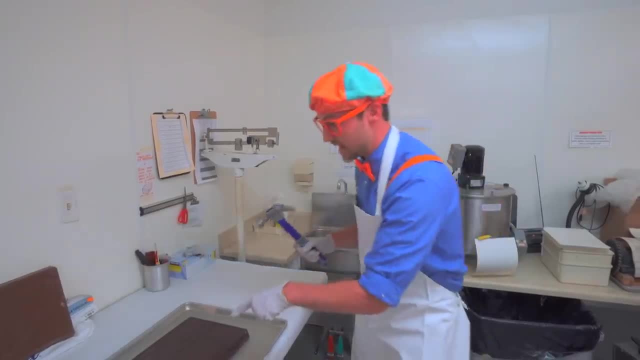 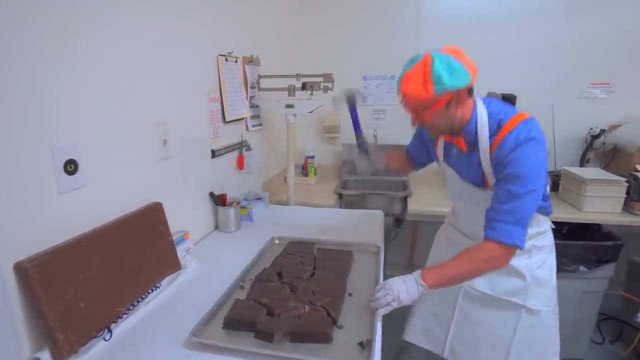 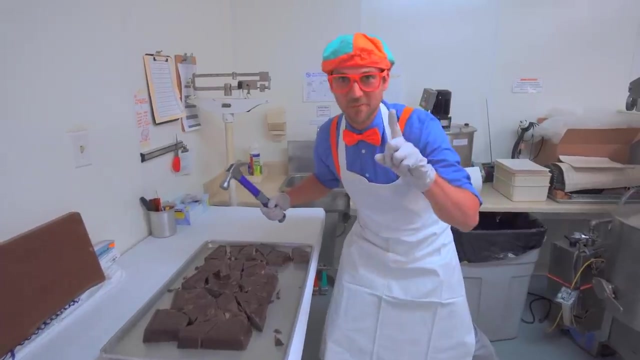 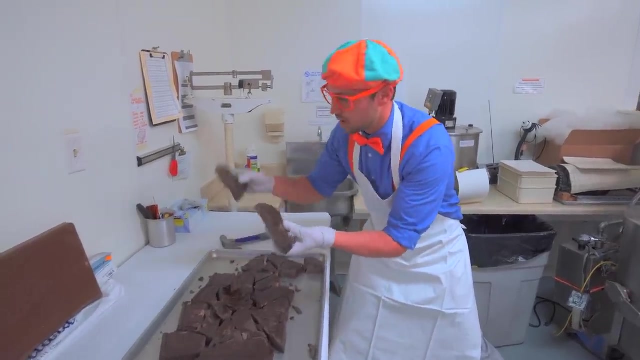 This hammer is only used to smash this big bar of chocolate. Ready, Ready, Yeah, Yeah, That was awesome. One more, Another one. There we go Now. it's in a lot smaller pieces, But still really big, So let's take this over to the heater. 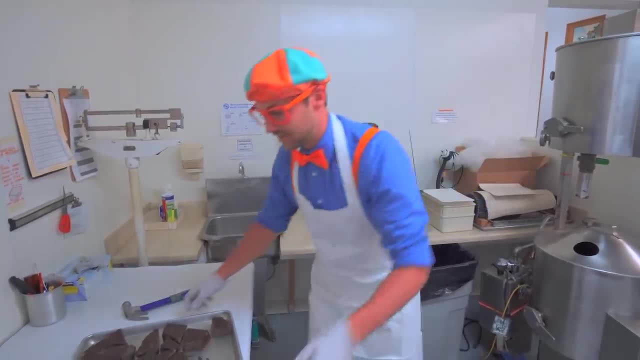 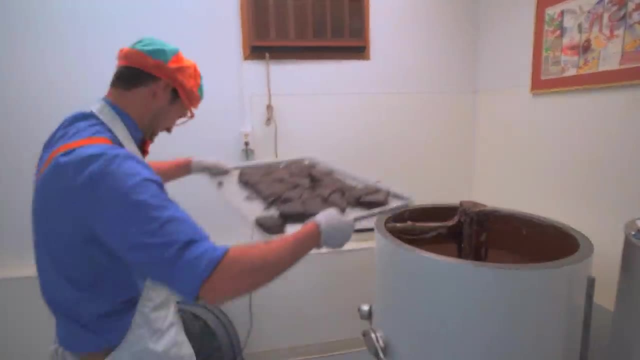 But first we need to take the cover off of the heater And then, Oh look, They did it for me. Thank you, Ooh, Check out, Check it out. Look, Whoa, That looks like some tasty chocolate. 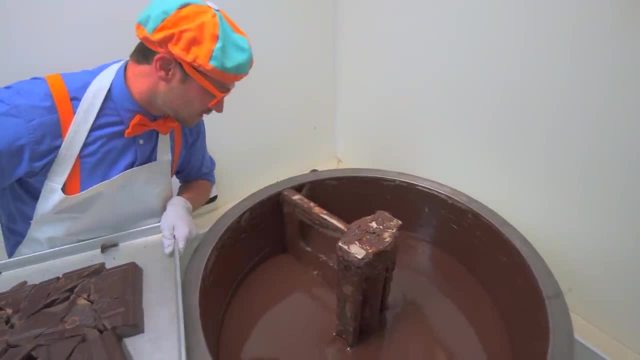 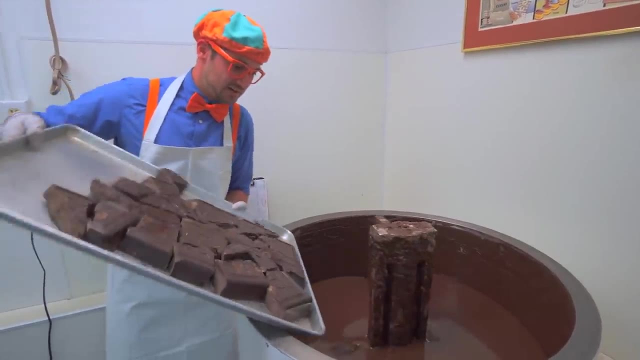 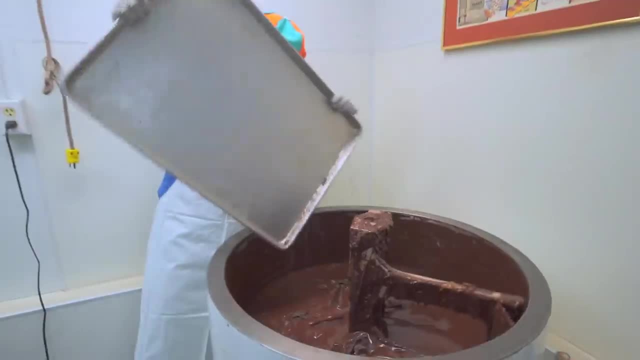 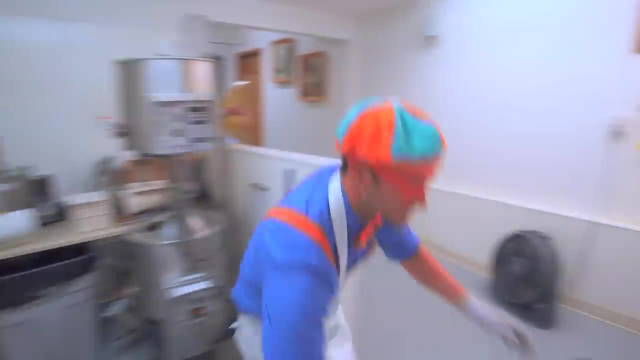 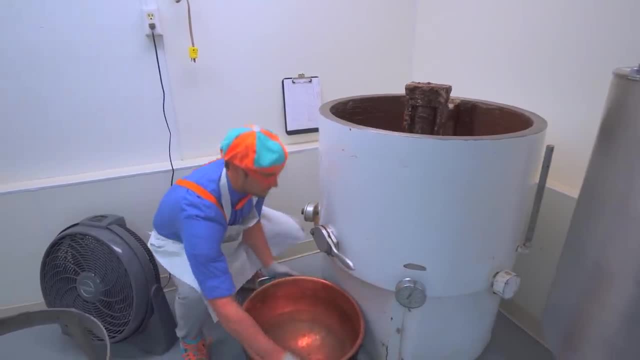 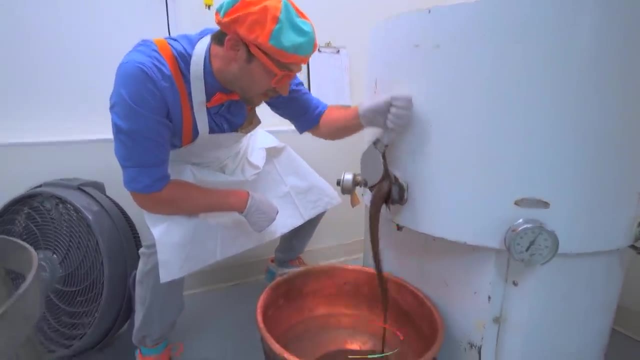 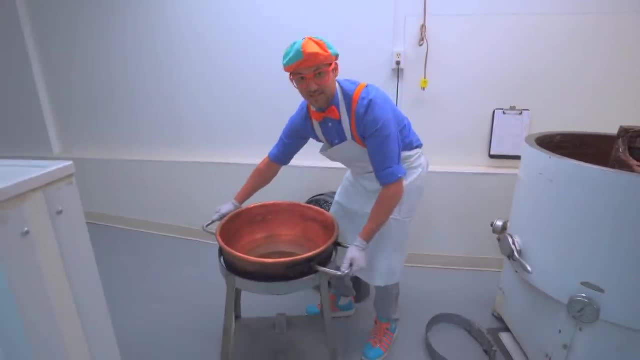 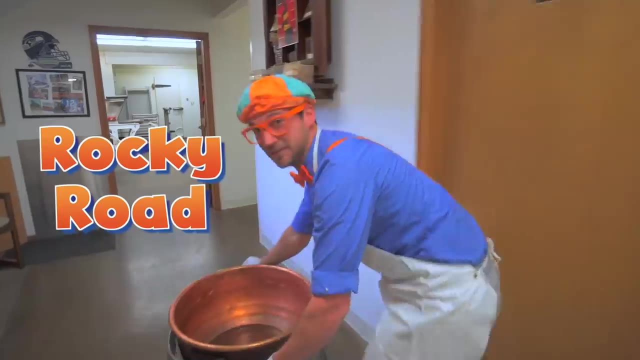 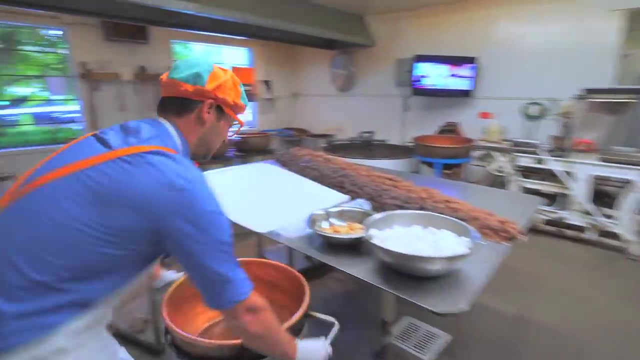 It's melting. Oh, it's really heavy. Okay, let's take the chocolate up here And what we're gonna do is make some rocky road. Do you know what? rocky road is Really tasty, All right. so, since that chocolate was really warm, 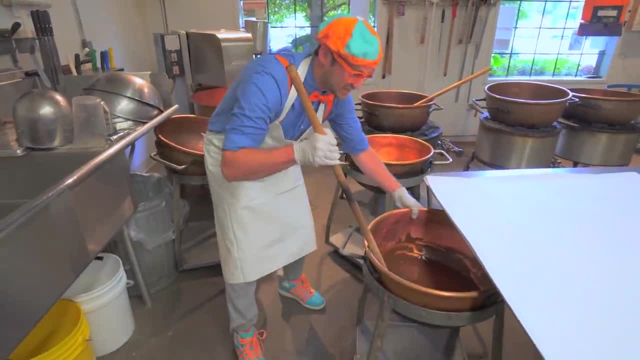 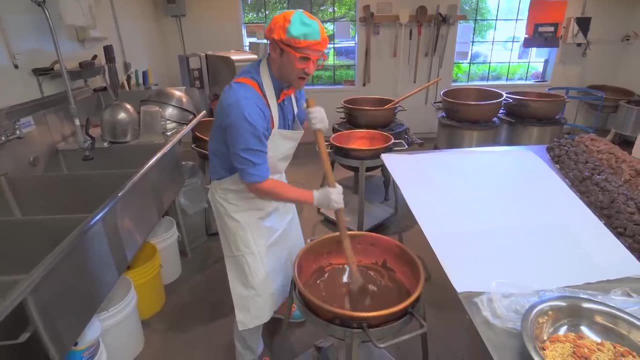 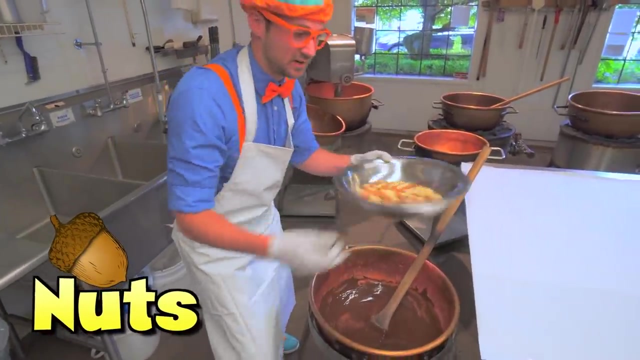 we let this cool down just for a little bit. See, here's some tasty chocolate That's just slightly cooler. All right, so we have some chocolate and then we take some nuts- looks pretty good. And then we also take some marshmallows. 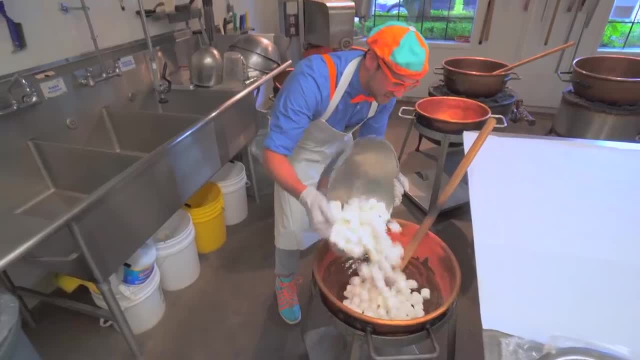 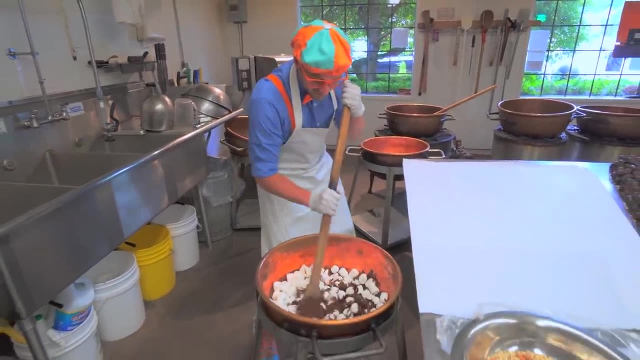 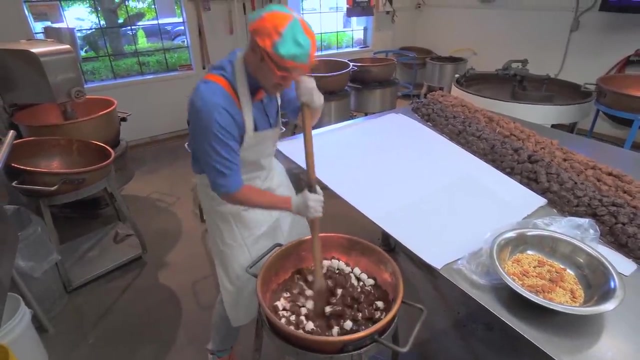 Let's put the marshmallows in first And we mix them all up together. Whoa, okay, here we go. Whoa look, Whoa, yep, You have to mix the chocolate and the marshmallows really good together. 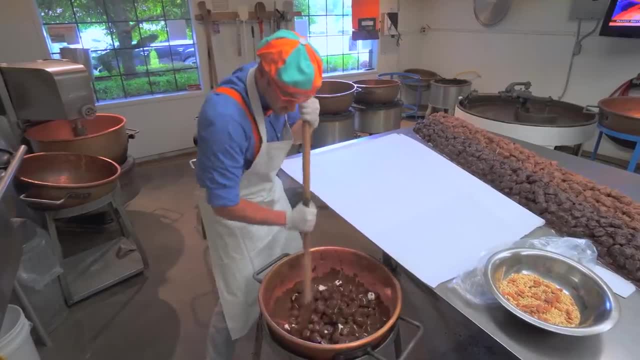 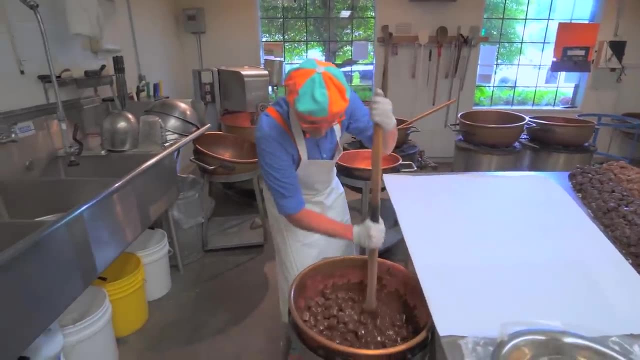 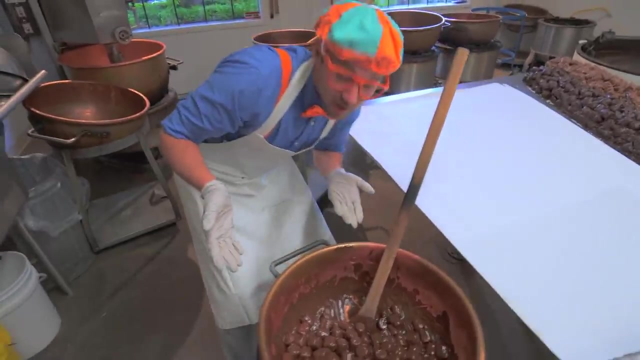 So then you see no white, You only see chocolate. We're almost there. Ooh, all right, looks pretty well mixed, Do you see that Looks like chocolate covered marshmallows. All right, now we need to put the nuts in there. 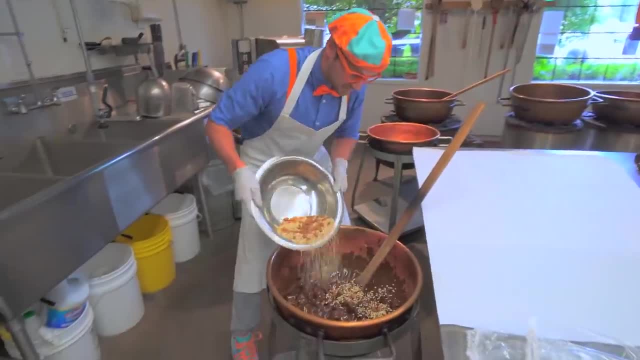 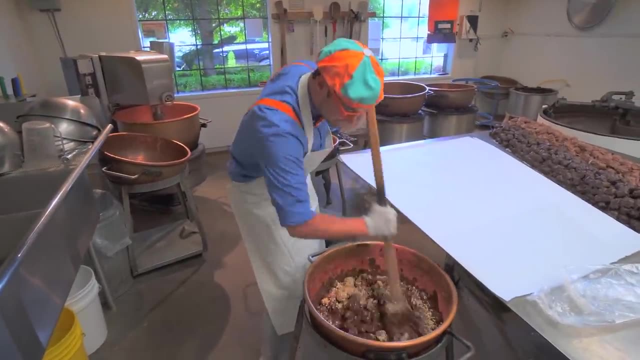 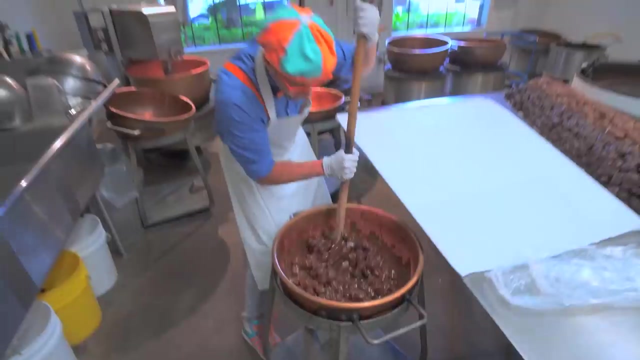 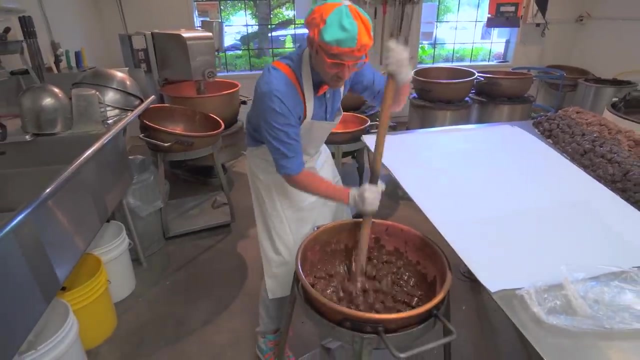 So let's sprinkle them in, Stir it up. Okay, here we go, Let's stir it up. Ooh, now that looks tasty, All right. so the next thing we have to do is take it out and put it on the table. 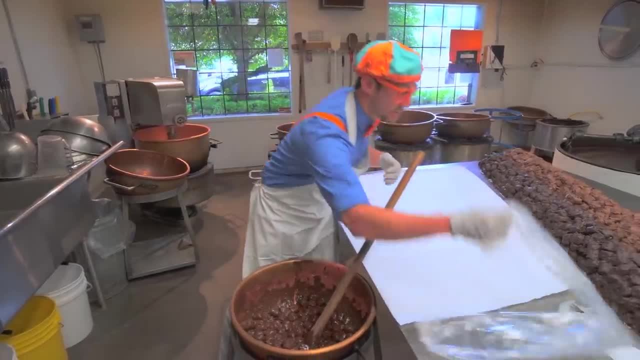 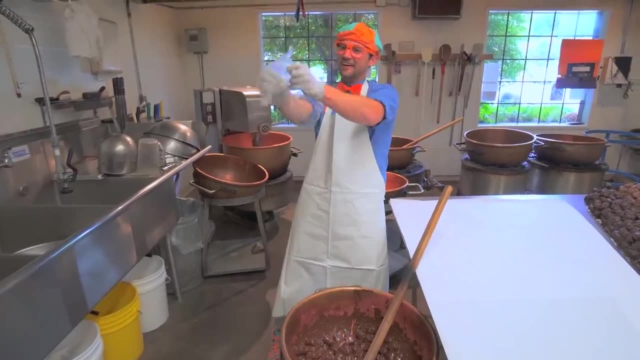 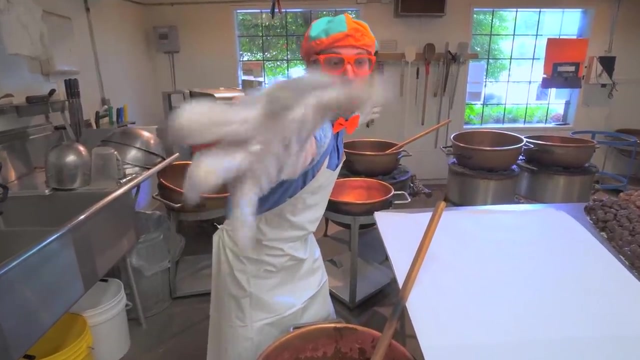 It's gonna get really messy. So the first thing we should do is put on these really big gloves. Whee, Look how big these gloves are. They go all the way up my arm. Whoa. And then let's put on this other one. 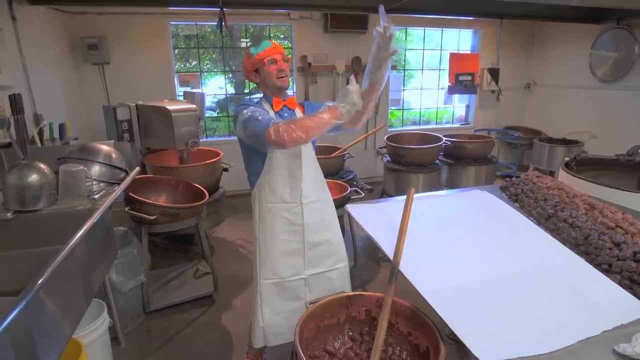 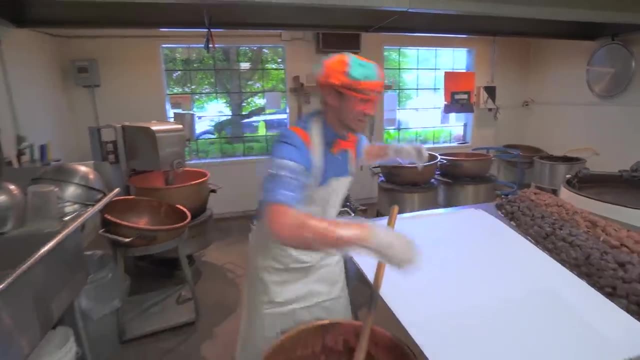 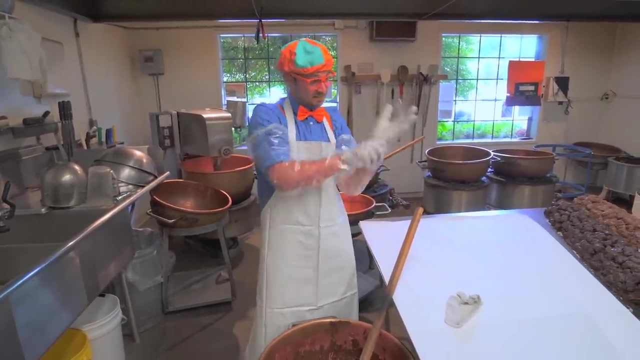 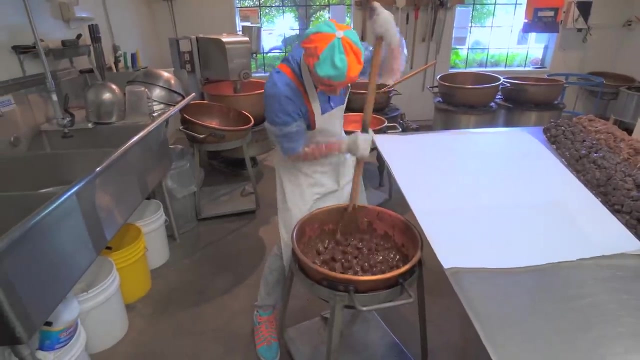 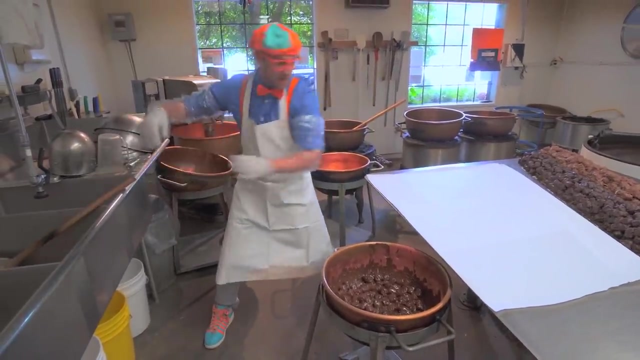 Okay, whoa, I have two giant gloves on One. two, Whoa. And then let's put another set of these small gloves on. Now we are ready. Let's give it one last stir. Okay, Let's put the mixing spoon over there. 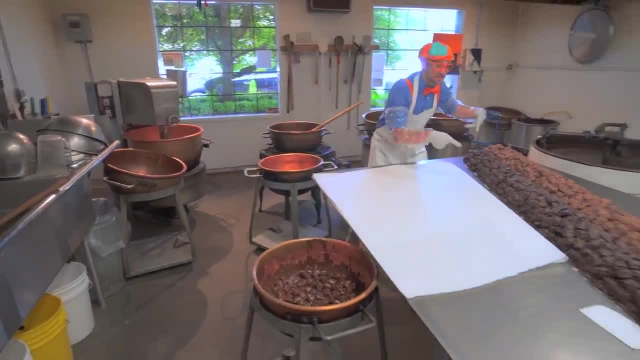 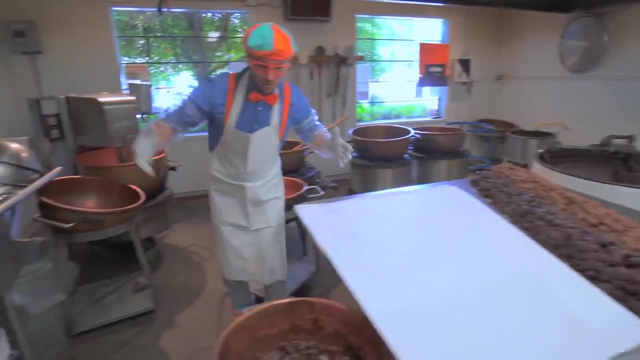 And what we're trying to make are really big logs that look like this. Do you see this? Whoa, That looks tasty. So let's take this, put it on the table, make it into a really long mound Ready. 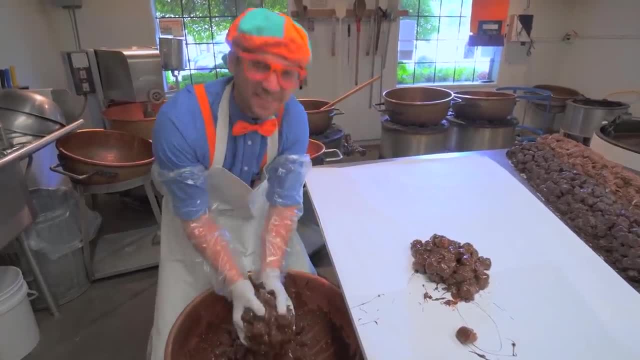 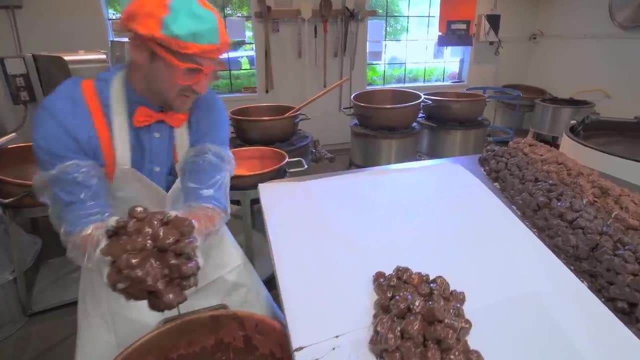 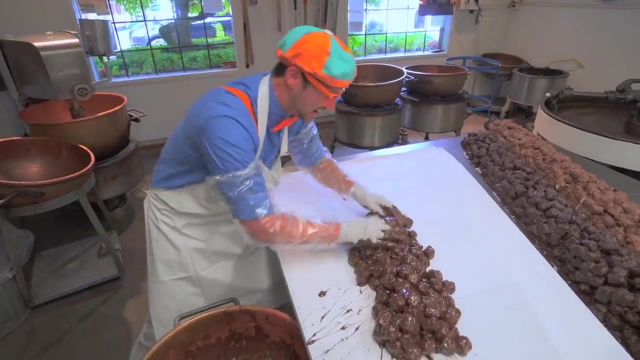 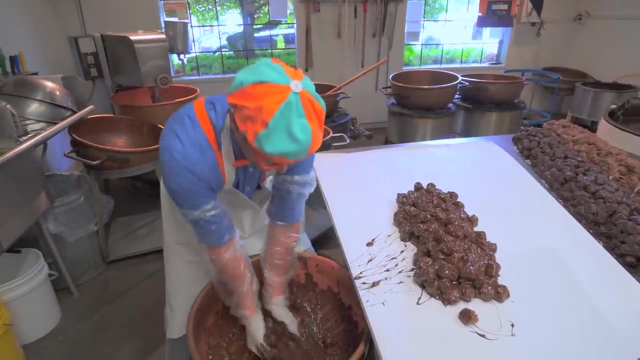 Whoa. It feels so mushy And it smells so tasty. Whoop, whoop, There we go. Oh, Oh, this is so much fun. Okay, there's a little bit more. Okay, this is a bowl that I sure want to lick. 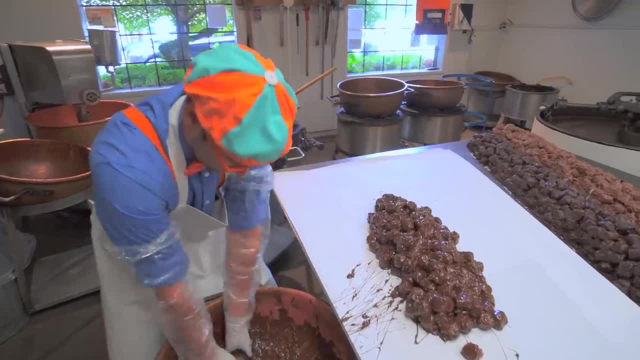 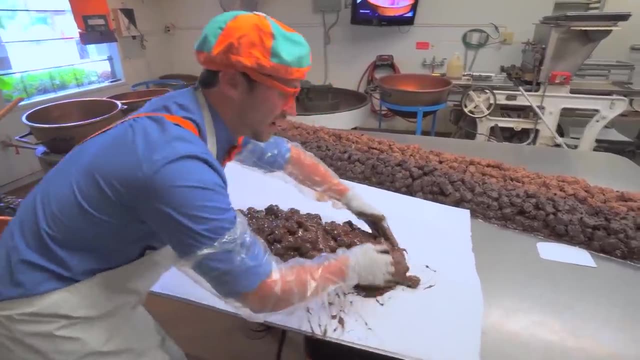 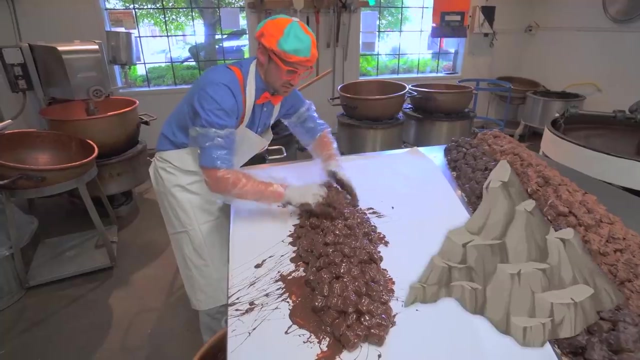 Okay, a little bit more. All right, I think that's all of it. So put that right there. Now I'm going to shape it into a really long mountain type of shape. Okay, There we go, There we go. 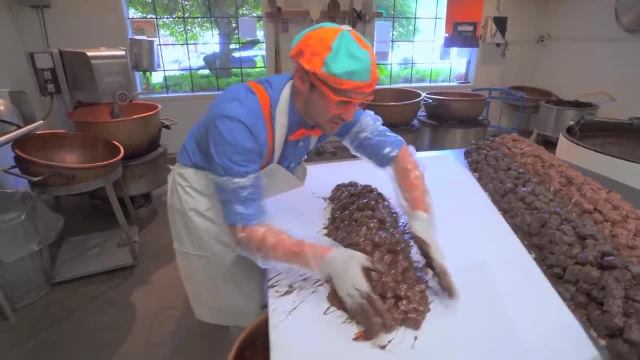 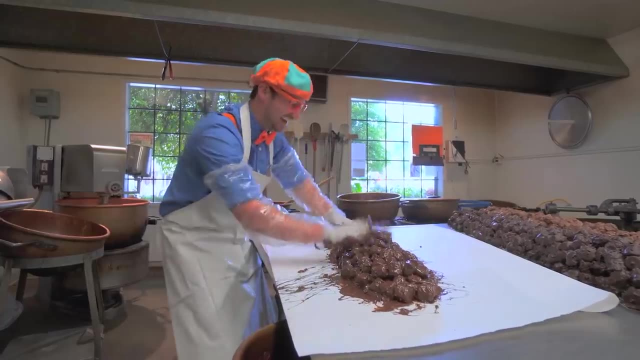 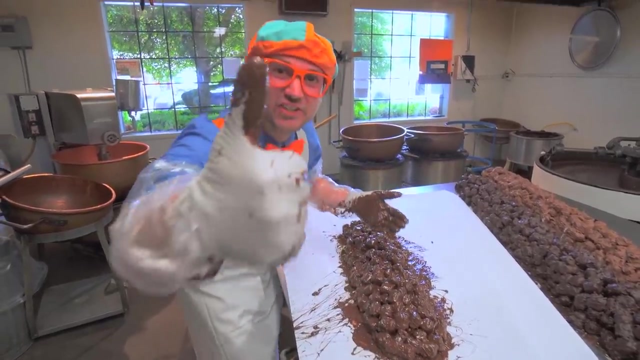 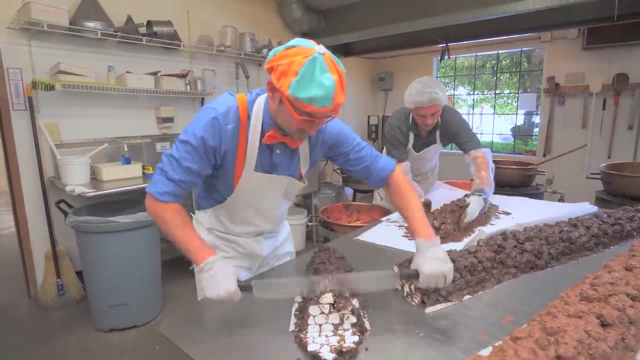 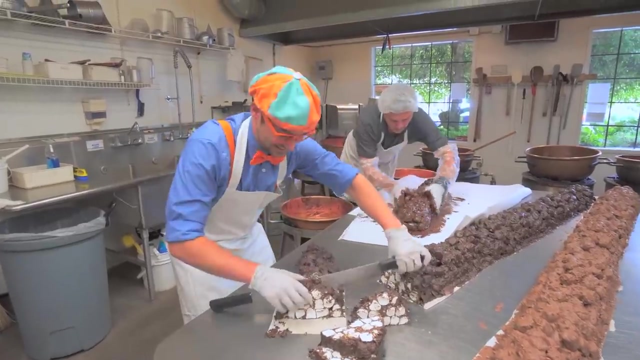 So this is a really long mountain type of shape that has a mound. Oh, Does that look good? Or does that look good? All right, So now what we do is let it dry and then we enjoy. Good job, Check it out. 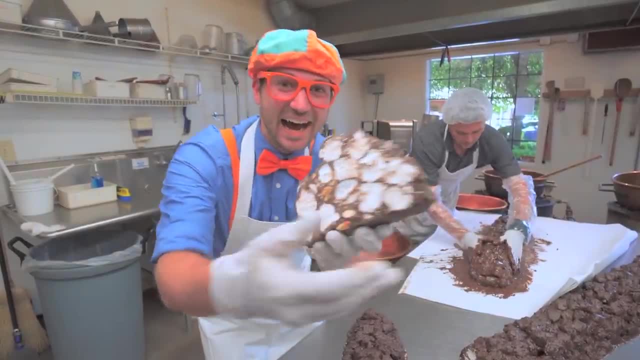 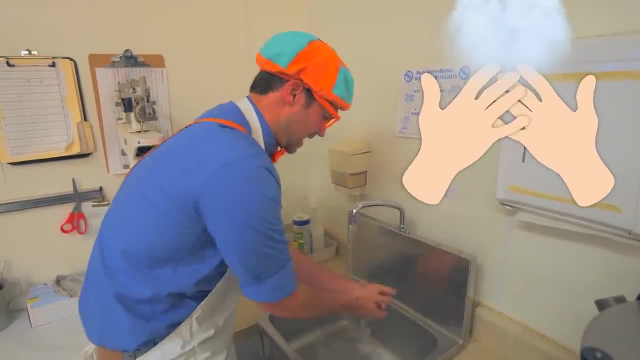 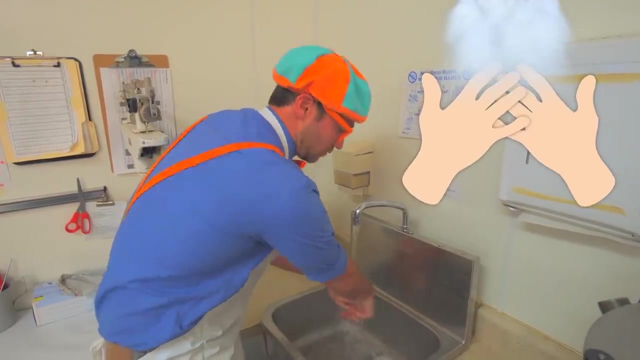 Now that's what I call rocky road. Ooh, Do you see what I'm doing? I am washing my hands, and I'm washing them really good, because what I'm about to do requires me to use my hands. All right, Let's dry them off real quick. 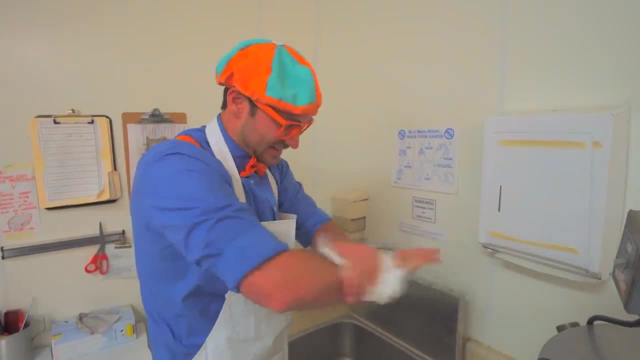 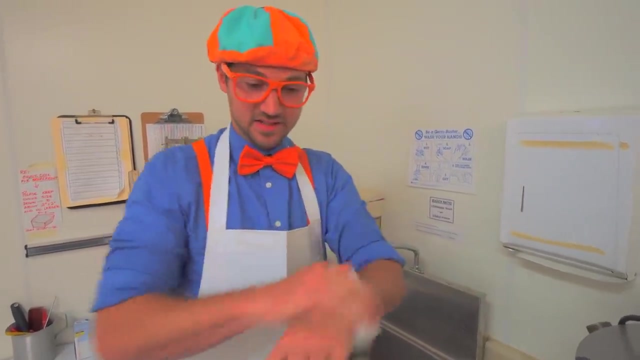 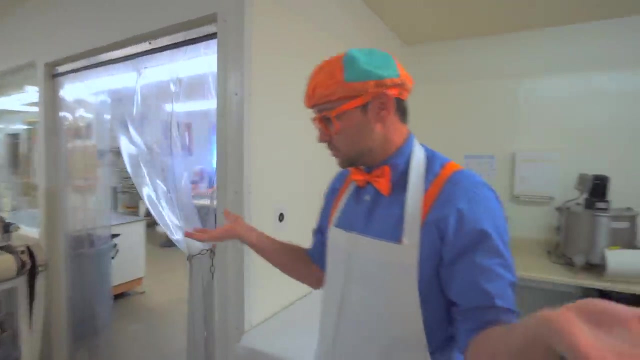 Oh, This is going to be fun. Oh, All right. Now my hands are really clean, So I'm going to use my hands as thermometers. Do you know what thermometers are? Thermometers help you check the temperature. Come through here. 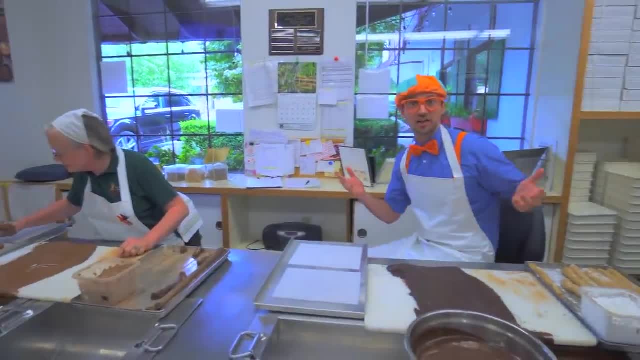 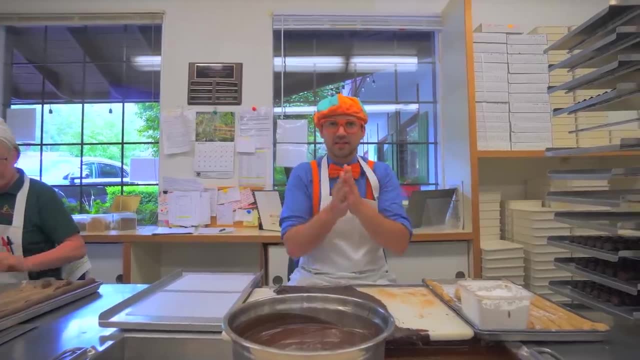 Whoa, And the temperature of this chocolate that I'm going to use is really important, And that's why I'm not using any gloves, So I can touch the chocolate and make sure the temperature is perfect. Do you see this chocolate right here? 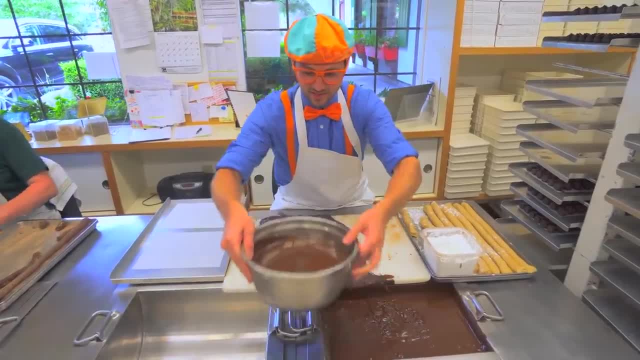 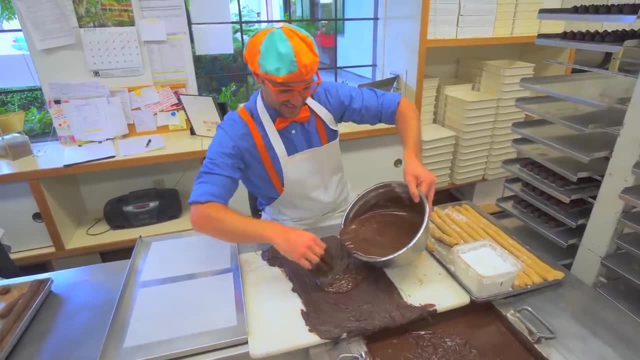 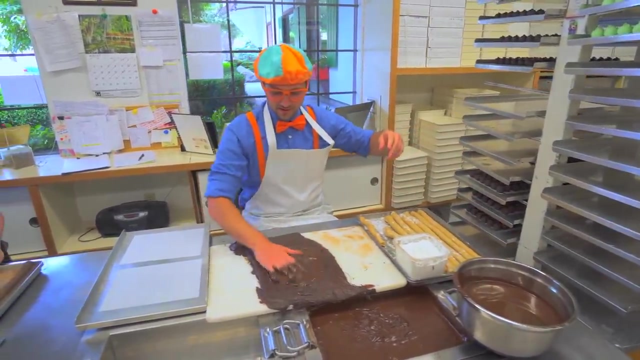 It's really warm, So let's take some and put it on the table. Yeah, Just like that. Perfect, I'll put that right there, And then you spread it around, just like this, And what we're doing right here is making truffles. 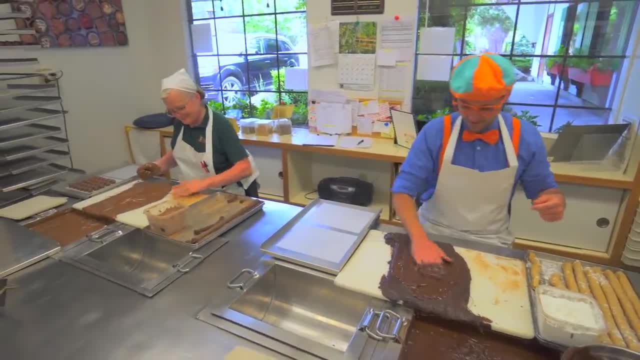 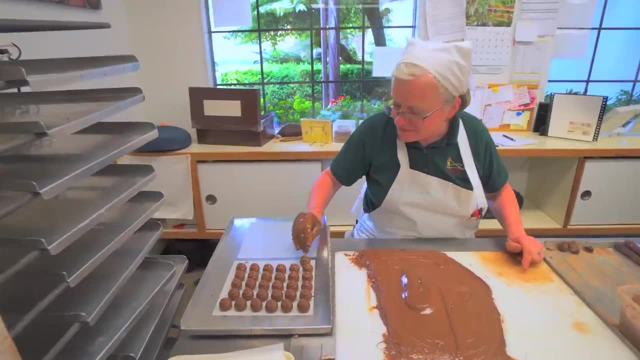 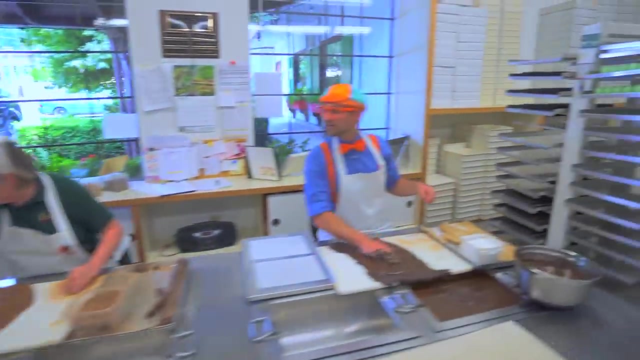 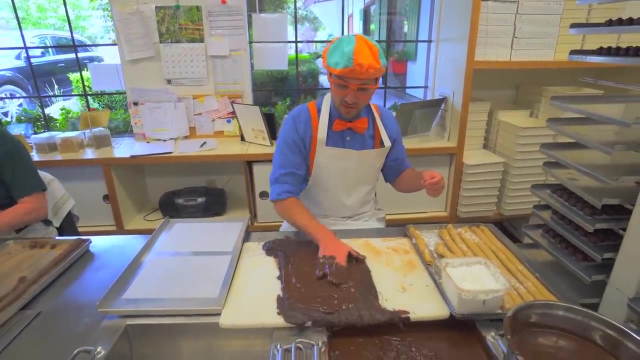 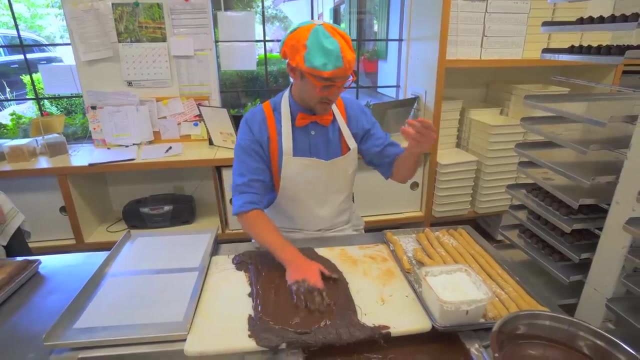 Oh, She's really good. Go look. Wow, That's fascinating. See, I'm moving my hand around the chocolate Here. Make sure it's the perfect temperature. All right, feels pretty perfect to me. So then, with my left hand, I'm going to grab some of this peanut butter. 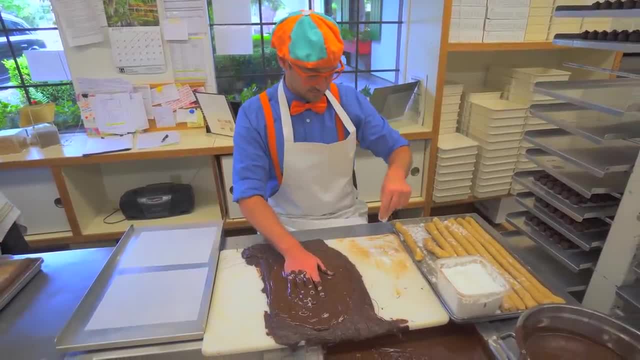 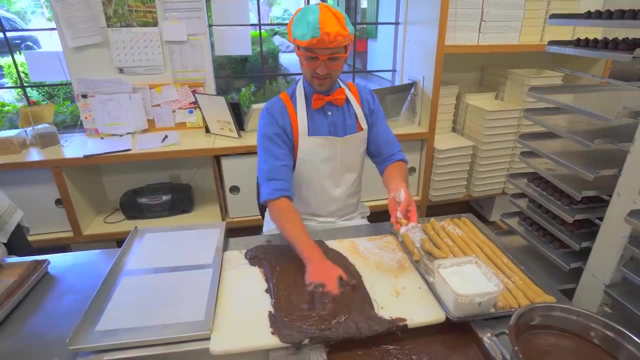 and I'm gonna take some of this white stuff, Put it right there, spread it around. Oh, I have to keep moving my right hand. It's pretty tricky. It's kind of like rubbing your belly and patting your head at the same time. Hey. 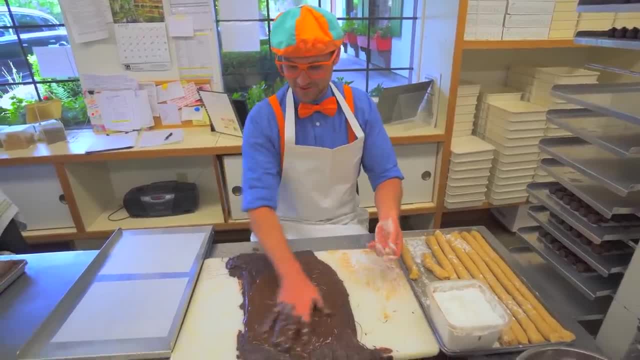 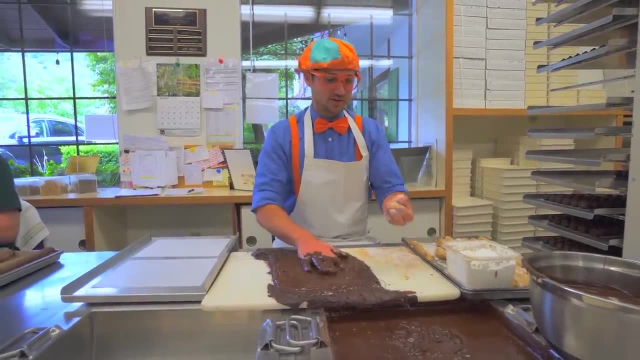 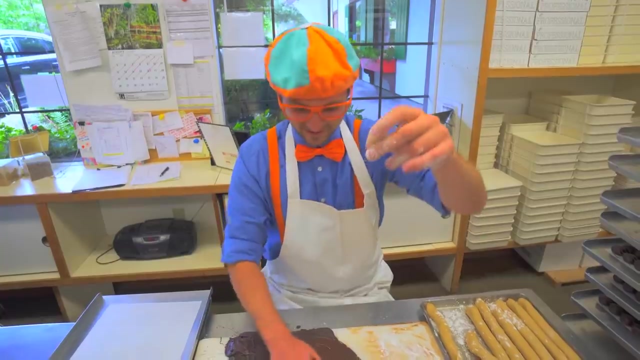 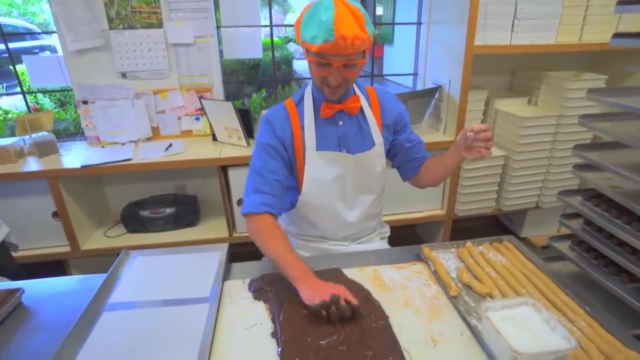 It's really hard and it feels so smooth. okay, That's gonna be Closest I can get to it. See, Kind of looks like a perfectly round circle ball. Okay, let's put it in my hand. Oh, Okay, and then looks like I put it on this tray. 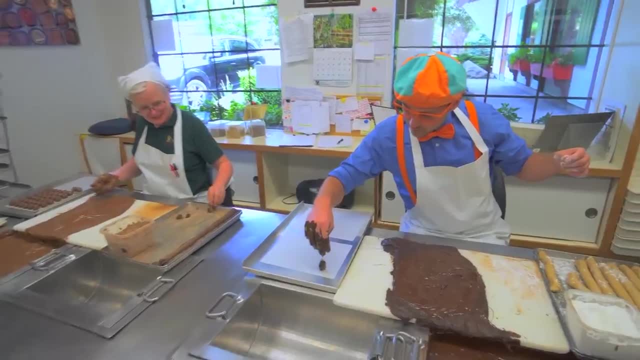 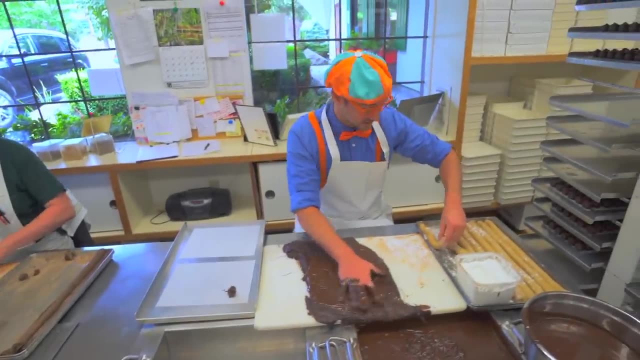 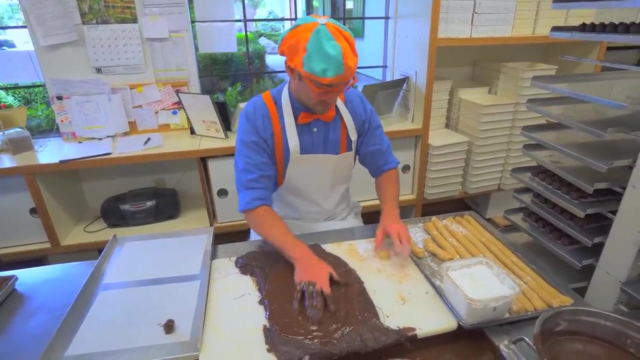 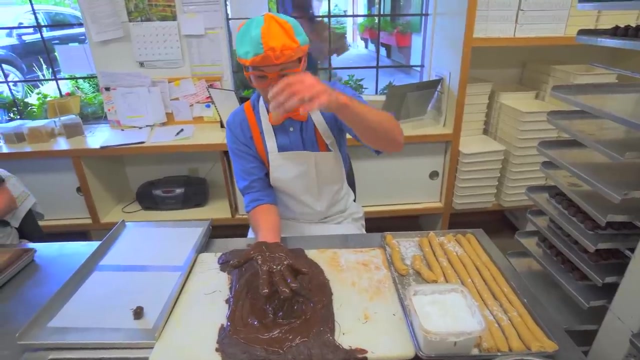 Just like what she's doing: Do a little swirl. That looks pretty good. let's make the next one a little bit bigger. I'm not very good, but practice makes perfect. Okay, here we go. All right, throw it in my hand again. Oh. 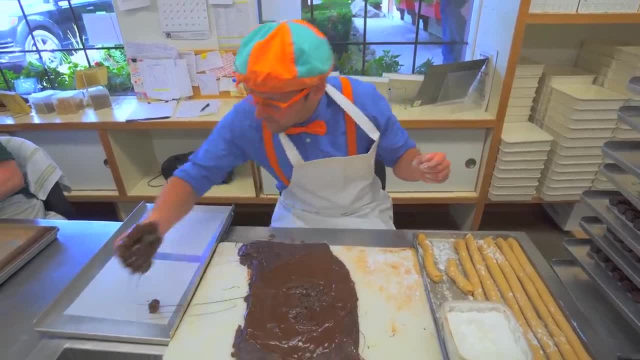 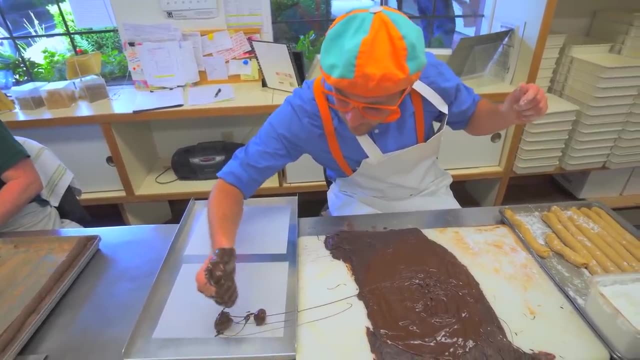 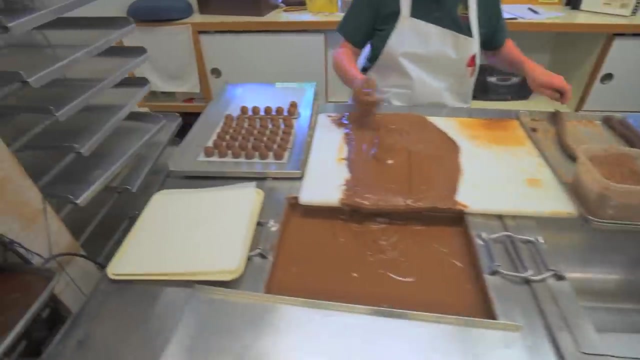 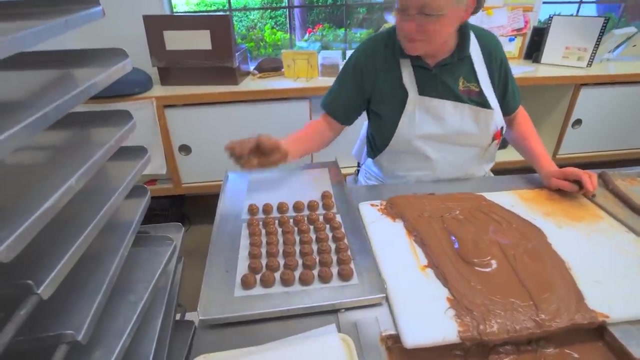 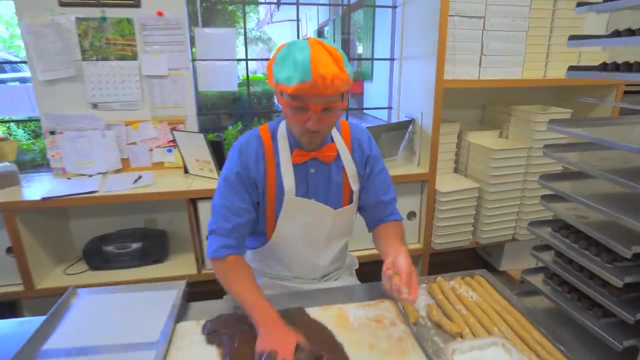 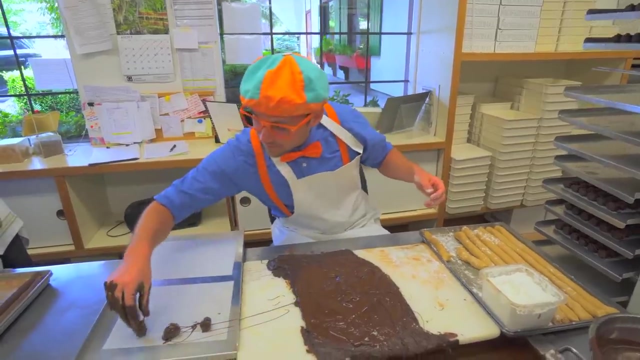 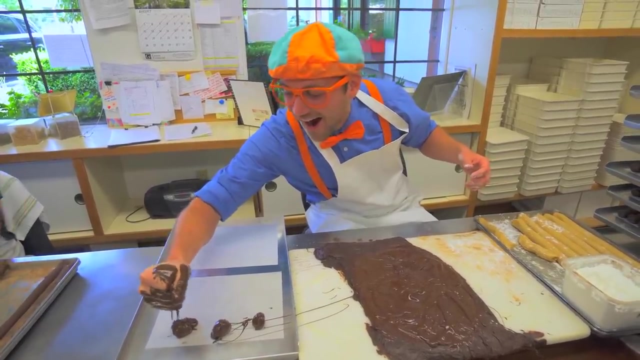 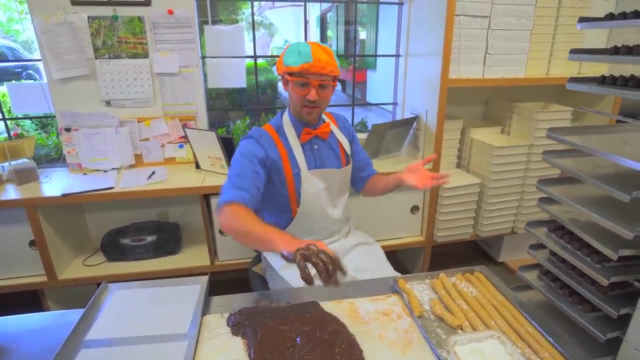 All right, Go. Whoa. no one has a lot of chocolate. Here we go. oh go, watch her again. All right, I'll make one last one. Swirl it around, Swirl it around. We're right there. Let's squeeze some chocolate on top. That looks like a tasty truffle. all right, now that I'm all done, let's go wash my hands again. 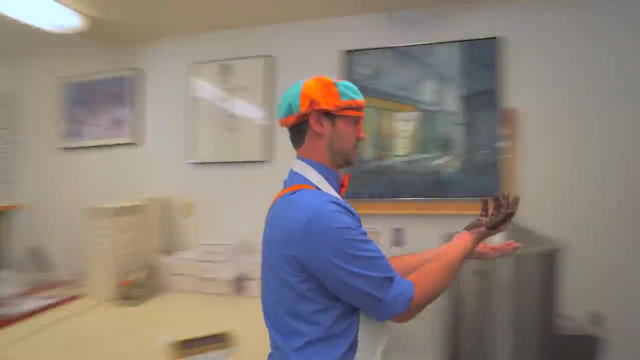 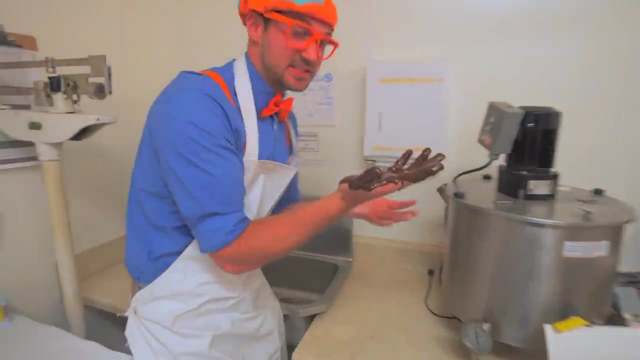 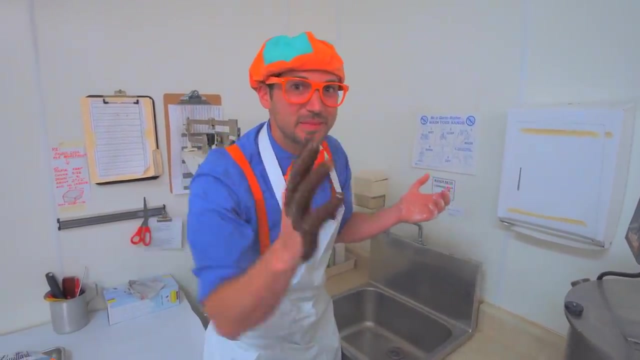 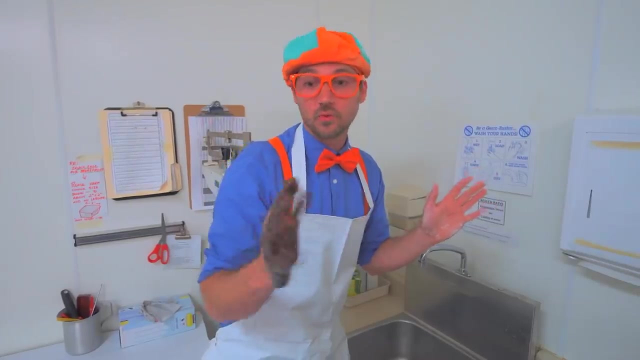 Let's go over here, Okay, Whoa, Oh, All right, Like I said, I'm all done and those chocolates are gonna be so tasty. You know what other chocolate might be tasty? Yeah, I'm gonna lick the chocolate off my hands because I'm all done with the production of the truffles, and then I'll wash my hands. 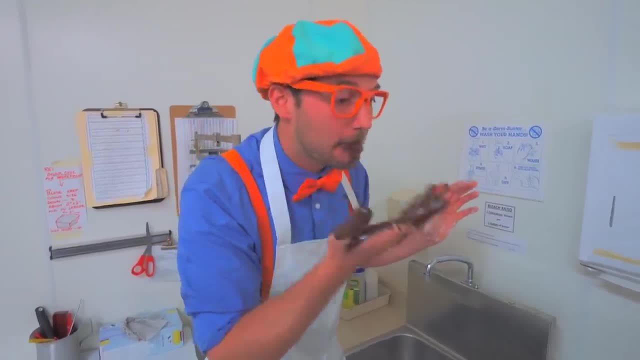 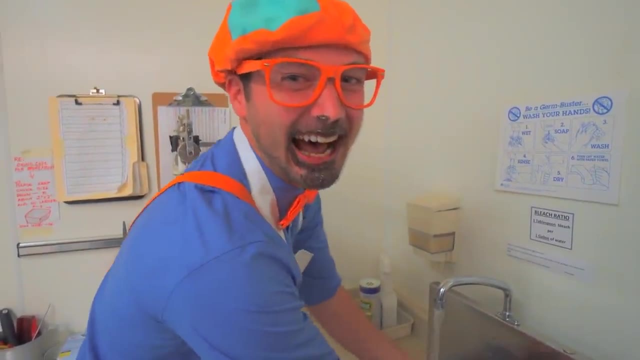 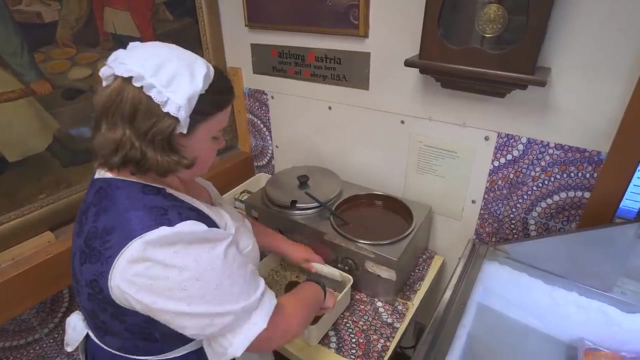 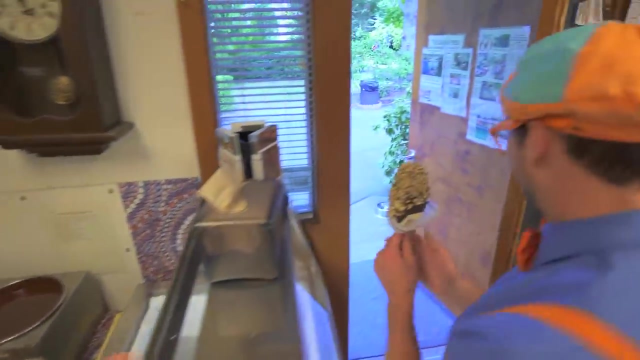 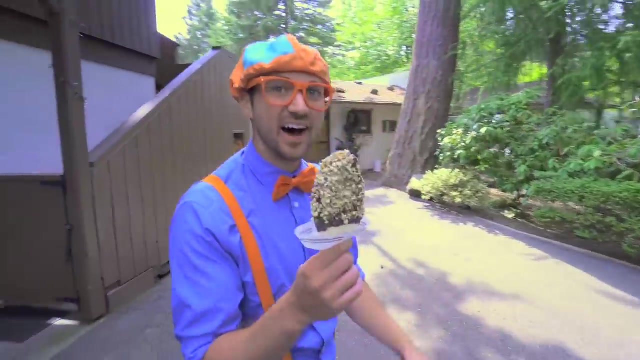 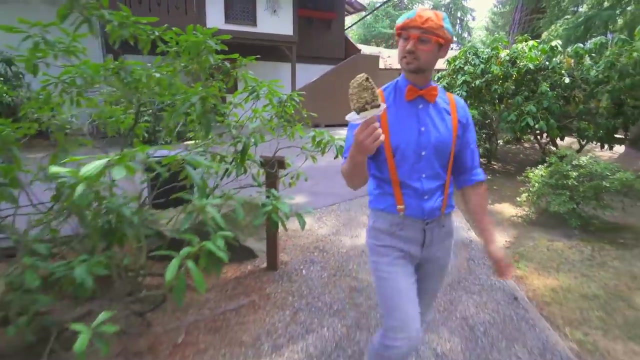 immediately after. That was super tasty. There you go, Thank you, Have a great day. Yum, I am so excited to eat this. Doesn't it look tasty? Whoa, Wasn't that fun learning about all those tasty treats Like this- This chocolate dipped ice cream cone. 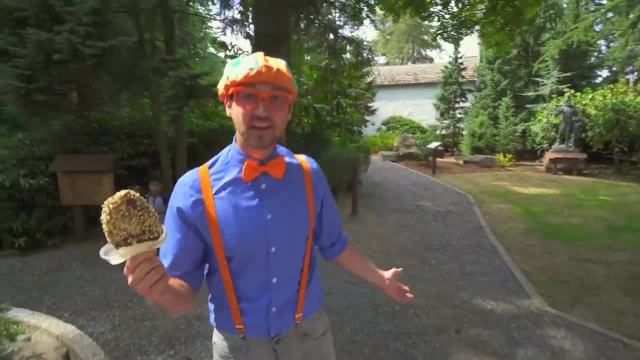 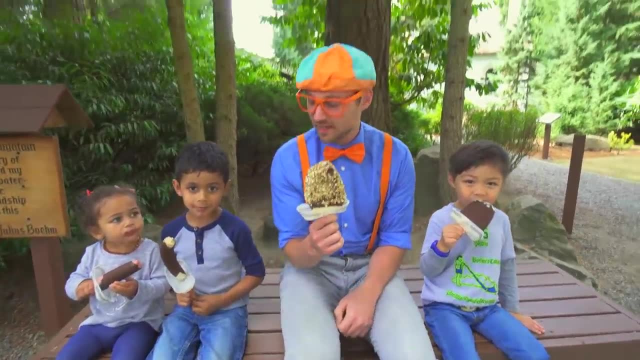 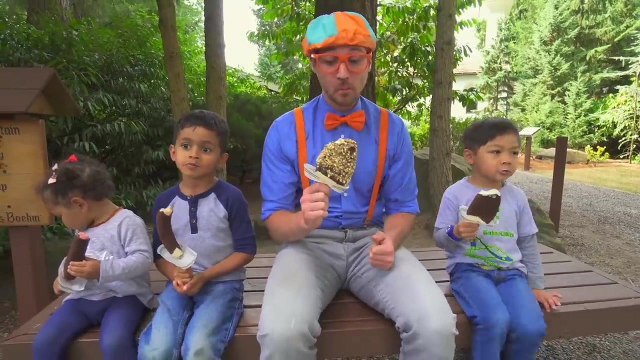 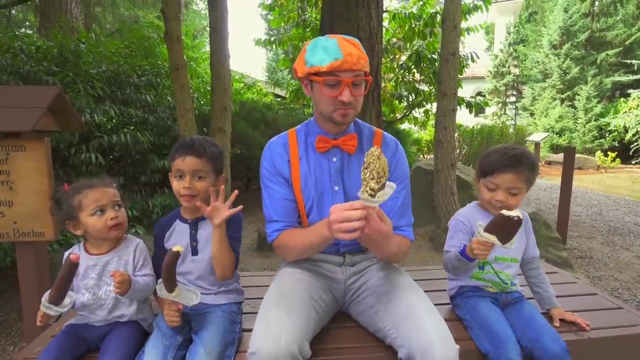 This is gonna be so good. We saw the conveyor belt. We made some truffles. Oh hey, some friends, Whoa, Let's try some. How's the sweet treats, kids? Mmm, Mmm, Mmm, Real good, Real good. Well, that was so good. 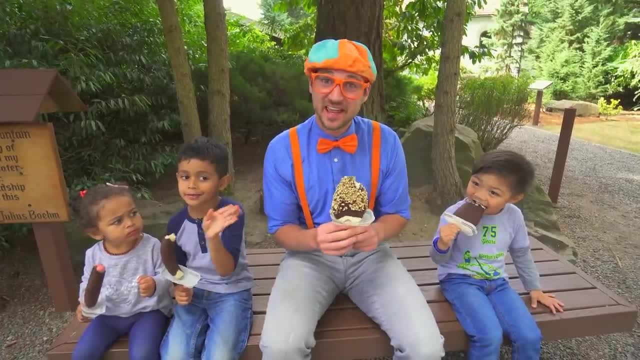 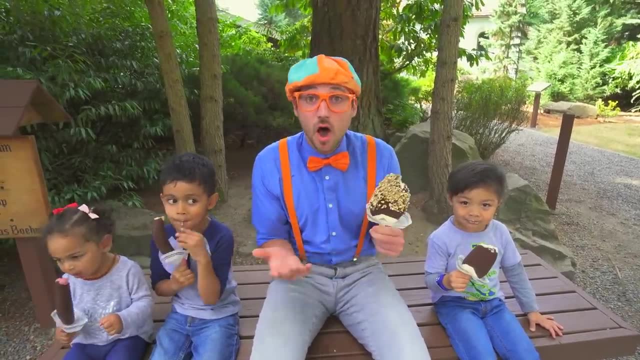 Well, that was so much fun learning what we learned today at Boehm's Candy Shop. Well, this is the end of this video, But if you want to watch more of my videos, all you have to do is search for my name. Will you spell my name with me? 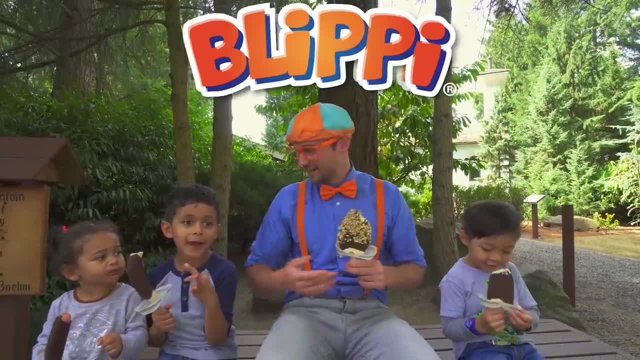 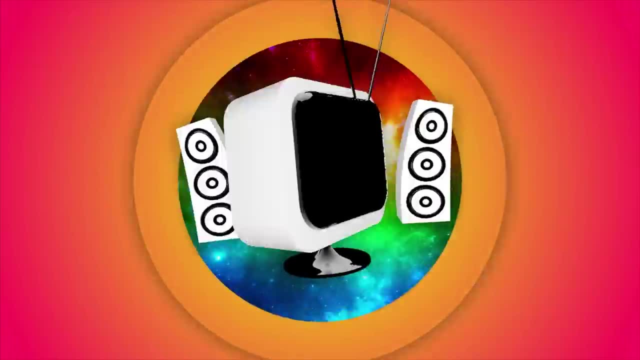 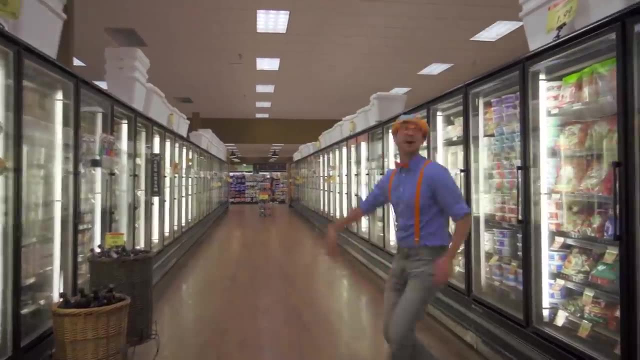 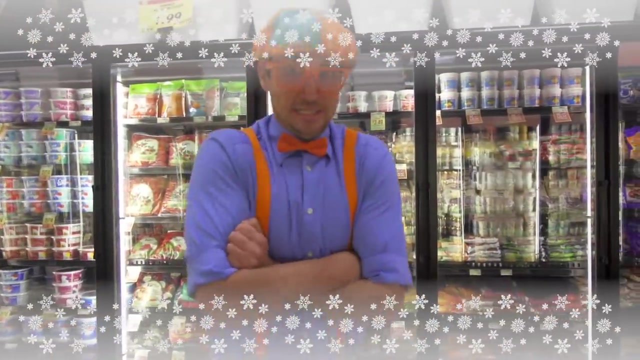 B-L-I-P-P-I. Good job, All right, see you soon. Bye-bye, Bye, Blippi. Wow, Look at where we are. We're in the frozen food aisle in the grocery store. But look at what it is. 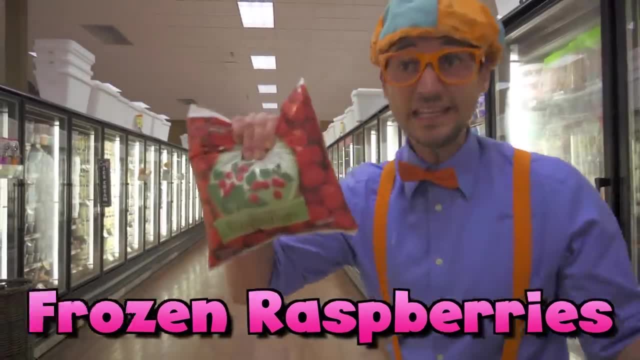 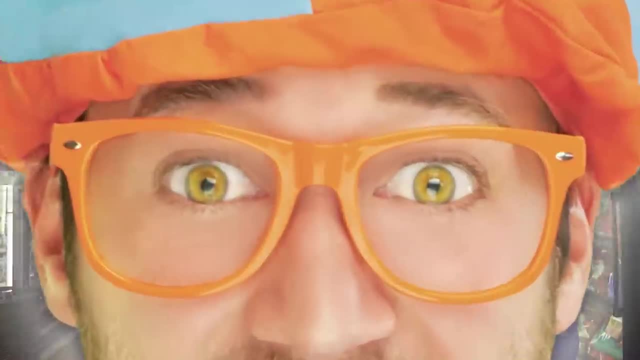 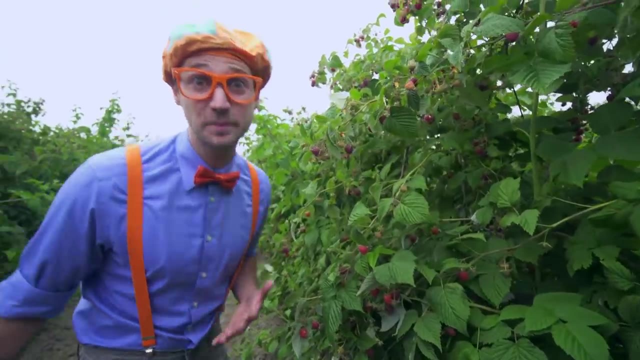 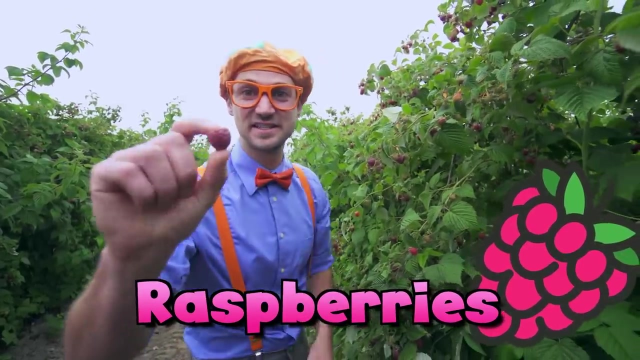 Yeah, Frozen raspberries. They're so sweet and high in vitamin C I wonder how these raspberries got here. Wow, Look at all of these raspberry bushes, And all of these raspberry bushes have raspberries on them, And this is the color: raspberry red. 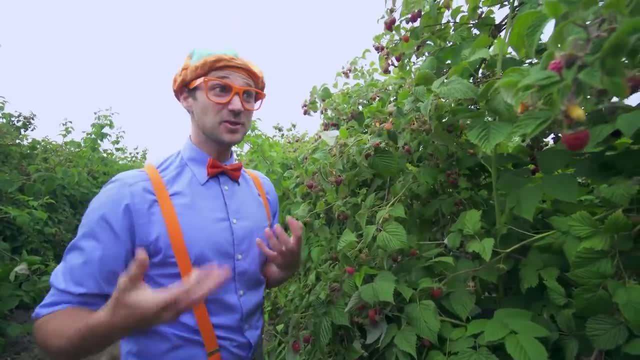 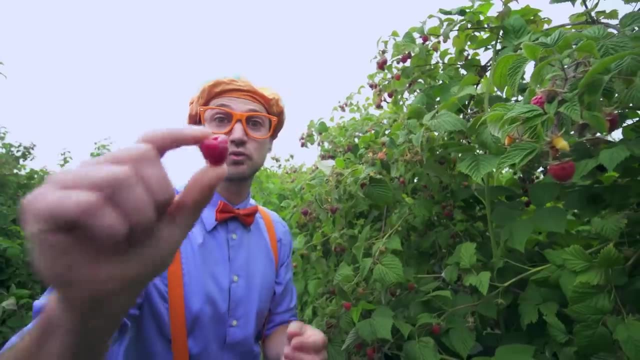 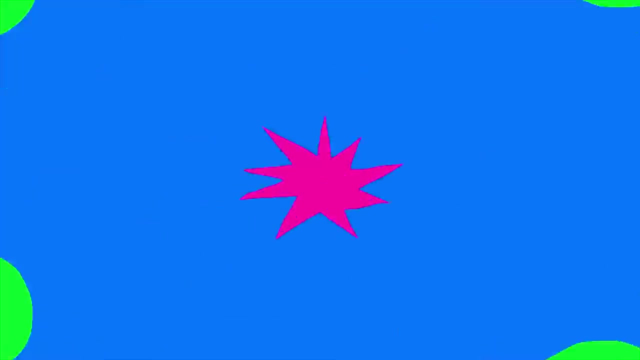 Mmm, Mmm, And it's so tasty. Well, since we're picking these to be frozen, We pick them at the perfect ripeness And actually we don't pick them. We shake them off with the harvester. Wow, We're in front of the harvester. 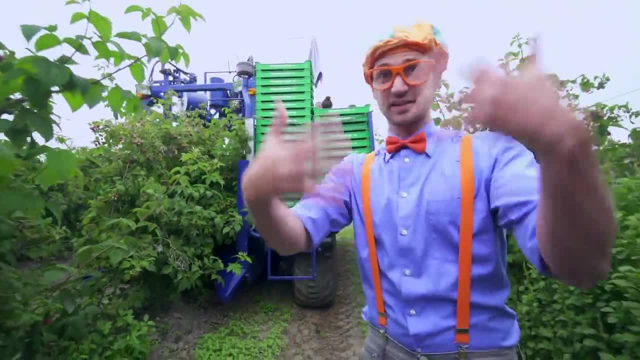 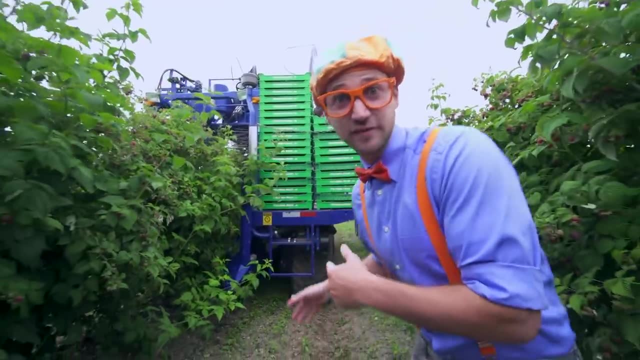 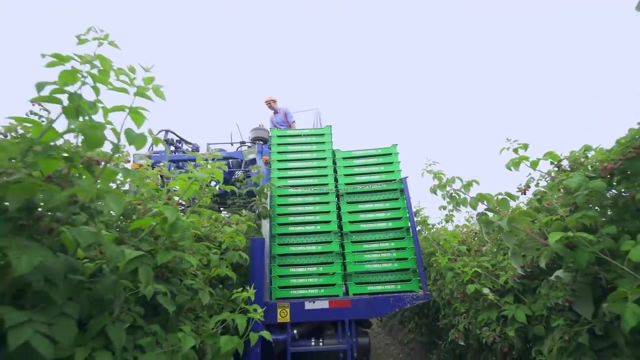 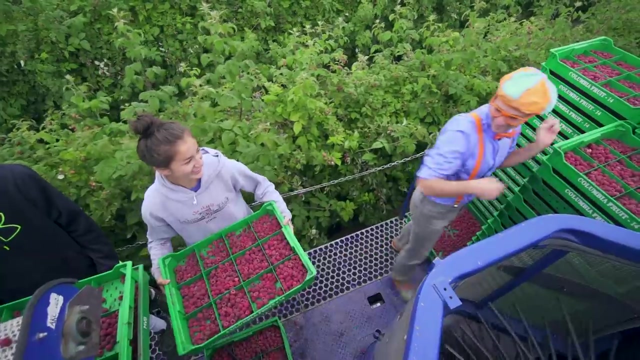 See, And deep in there it's shaking these bars like this: Da-da-da-da-da-da-da-da-da-da-da. And so then the really ripe raspberries fall off into the harvester. Look, So now we're on the harvester. 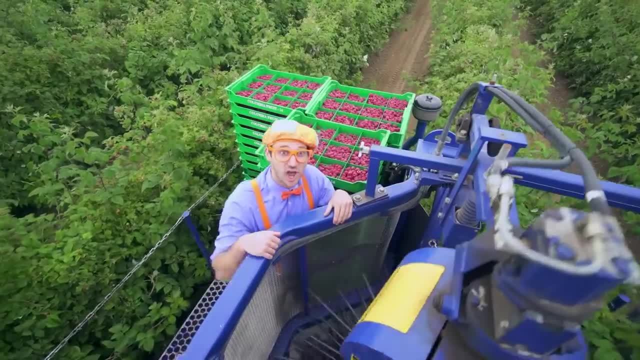 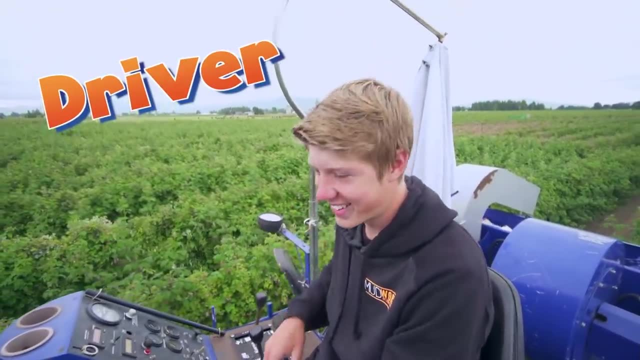 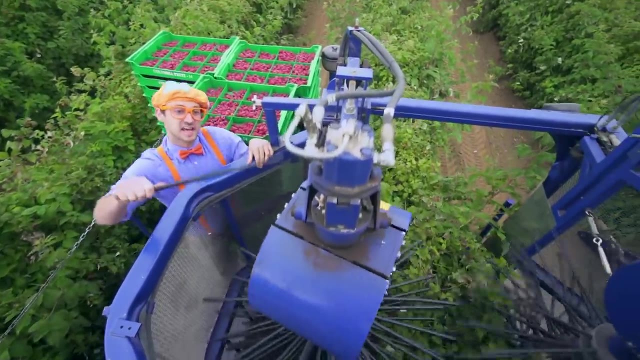 This is the machine that gives the raspberries off in the bush. And look at the driver. Hey guys, I'm the driver, See, And the driver operates the harvester And these things- yeah, They're plastic bars that go up and down real quick. 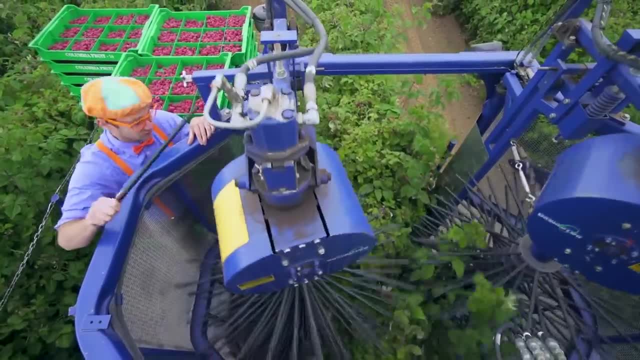 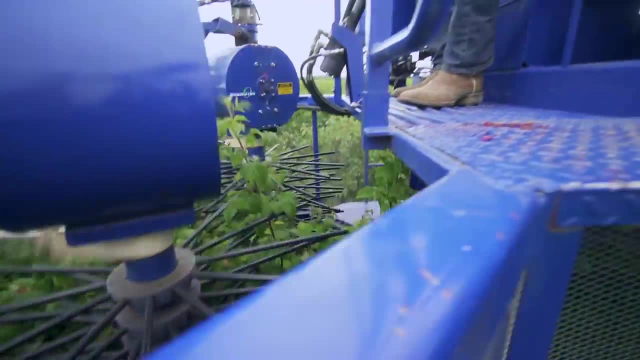 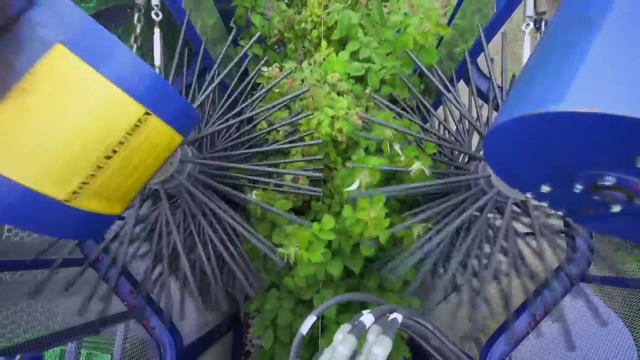 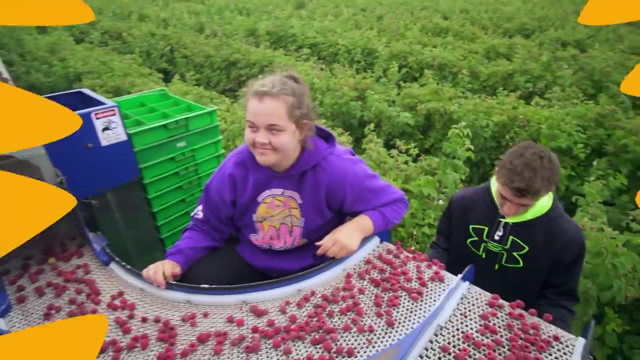 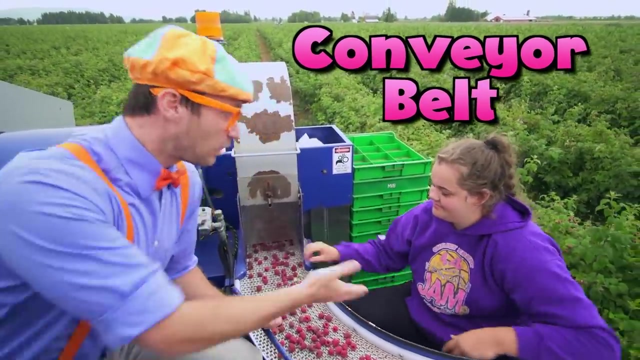 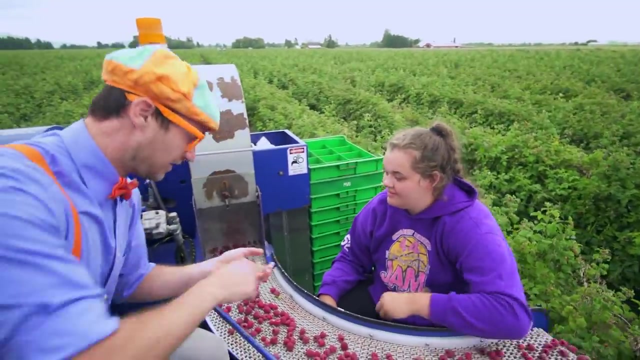 And shakes the raspberries off in the bush Music. After the raspberries get shaken off the bushes, They arrive on these conveyor belts. So what do you do? I would get all the raspberries and pick off the bad ones. Whoa Like, Oh, Like this one right. 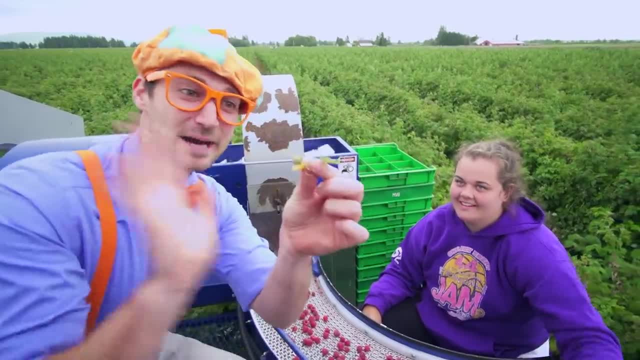 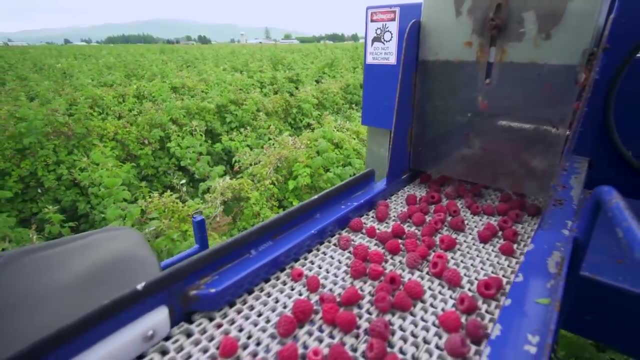 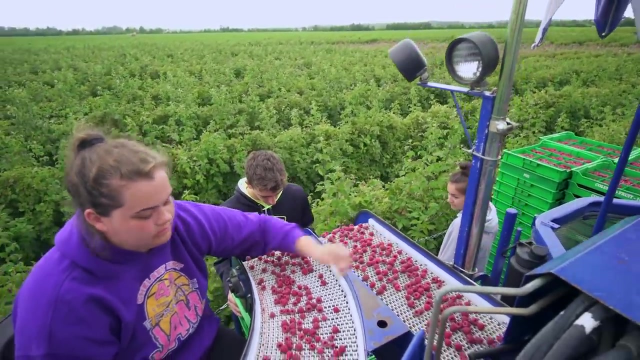 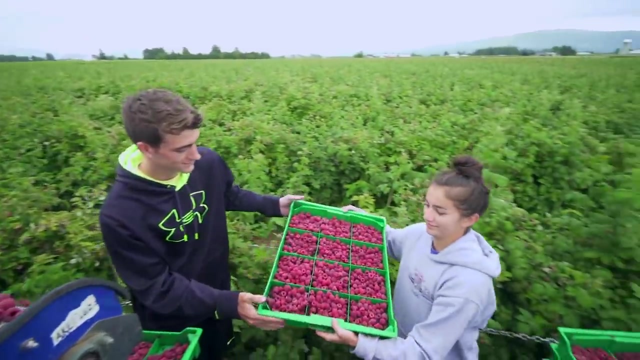 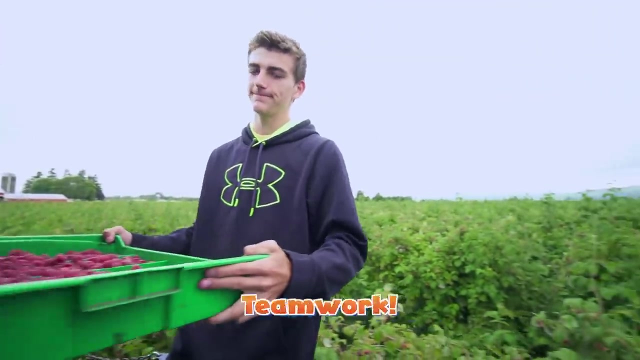 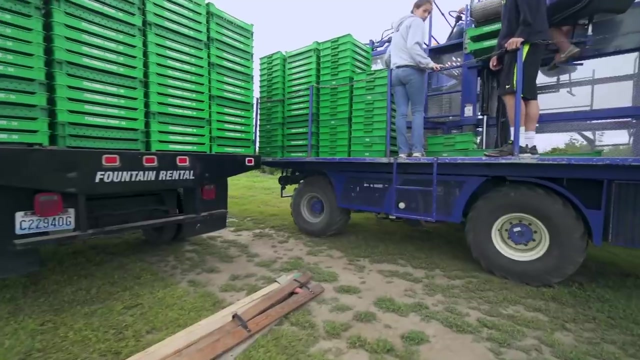 Perfect. Okay, put that there And say goodbye to this. Bye-bye. There she goes, Picking off all the bad ones. Wow, Look at him and his tray. He passes it to the girl And then she stacks them up. Good teamwork Now that the harvester is really full. 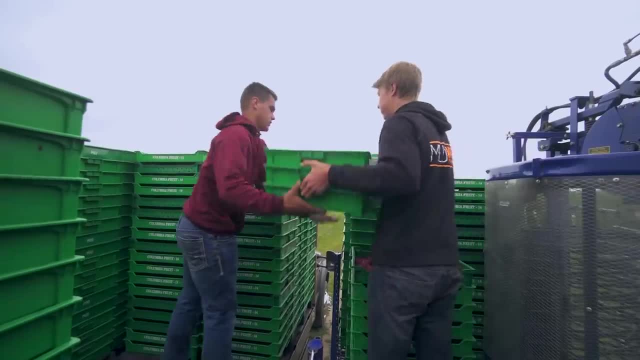 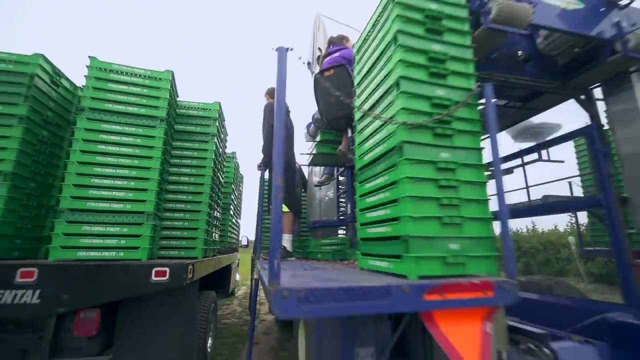 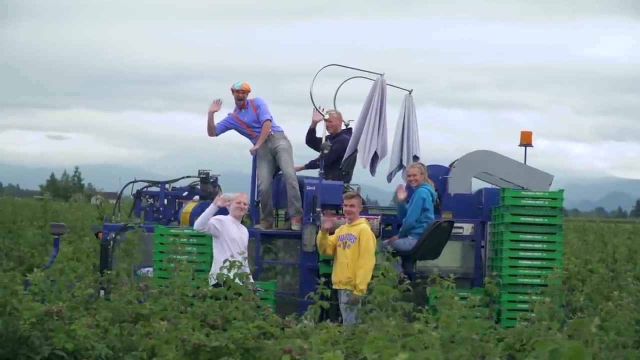 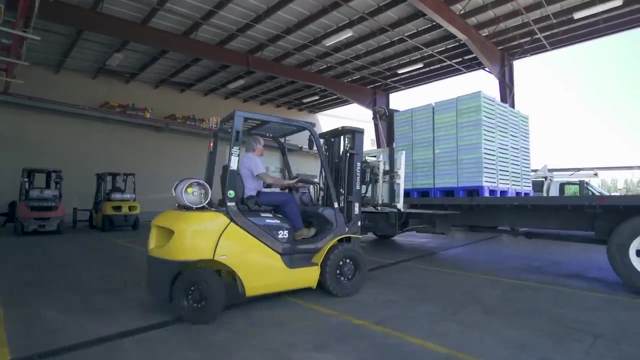 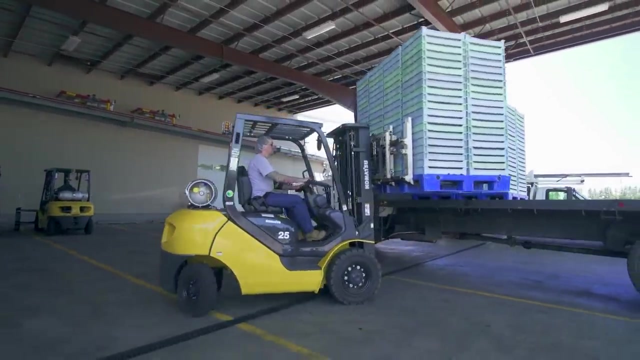 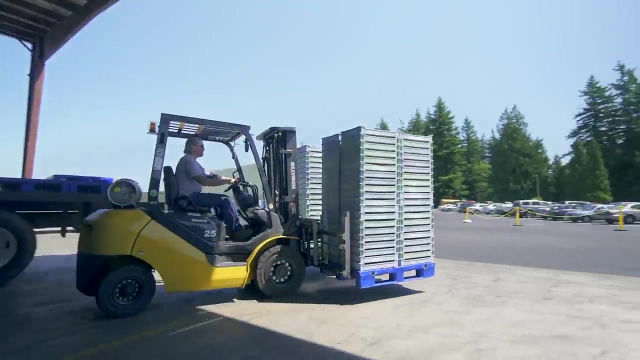 They have to pull up next to the truck And unload all of the raspberries Music. Now the truck arrives to the facility And then the raspberries get taken off the truck With a forklift. Music Whoa, That forklift can carry a lot of raspberries. 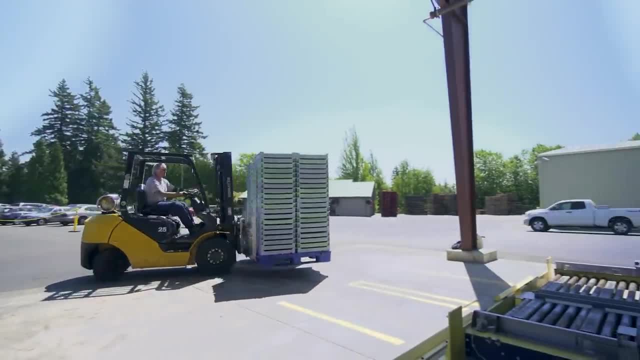 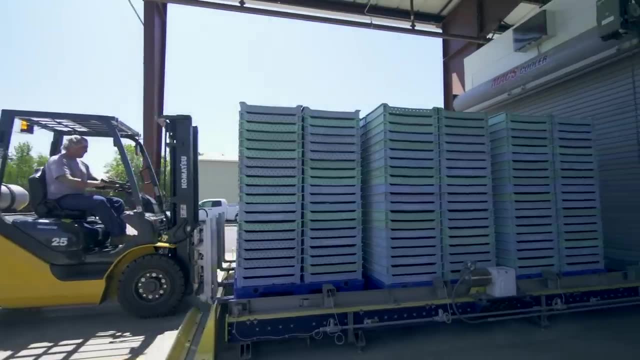 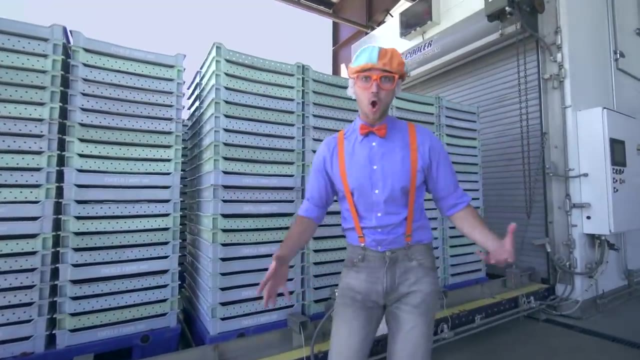 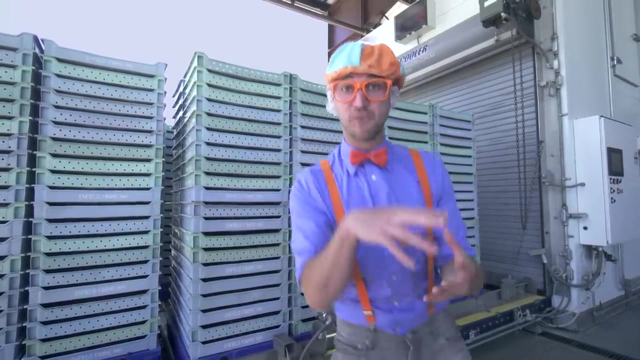 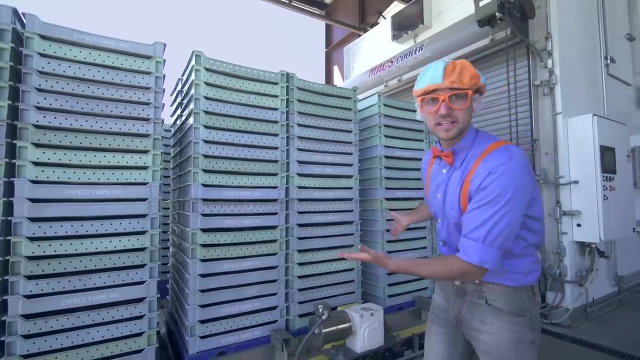 Music, Music. Okay, so the raspberries came from the farm And got transported from a truck, And then a forklift pulled it off of the truck And loaded it up right here, And so now all of these raspberries Are going to go into this cooler. 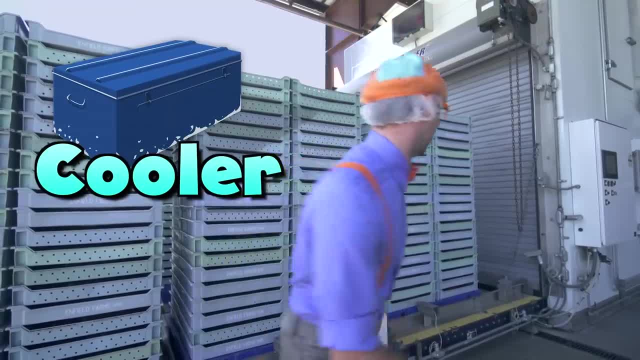 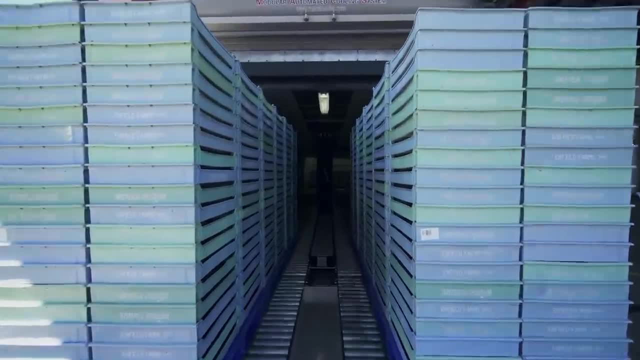 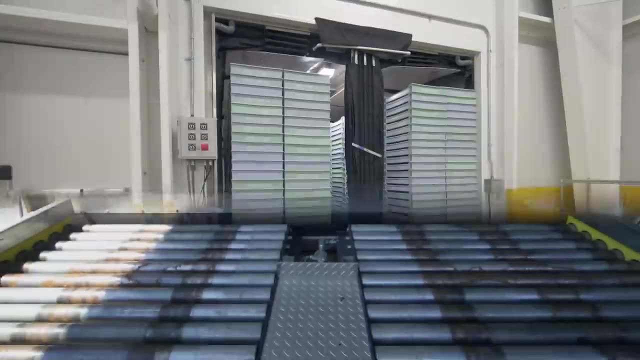 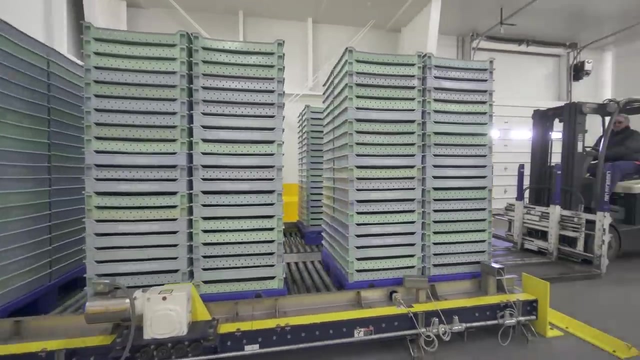 Watch this Music. There they go into the cooler Music: Wee Bye-bye Music. Oh hello. Now this is basically a giant refrigerator Music. So then the raspberries get nice and cold, Super quick Music. Look, he's wearing nice warm clothes. 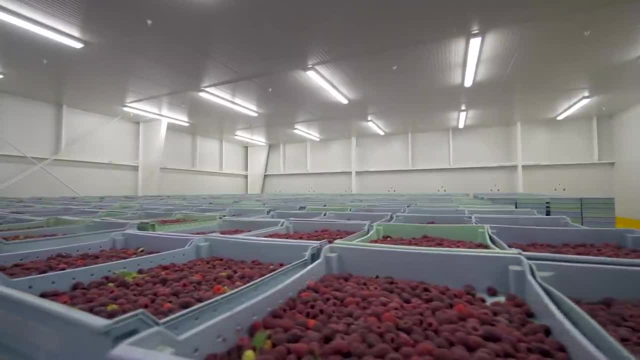 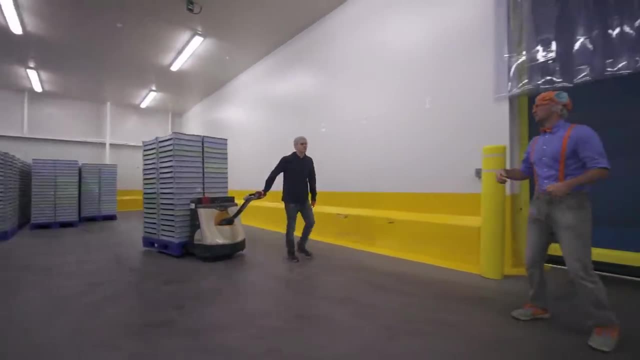 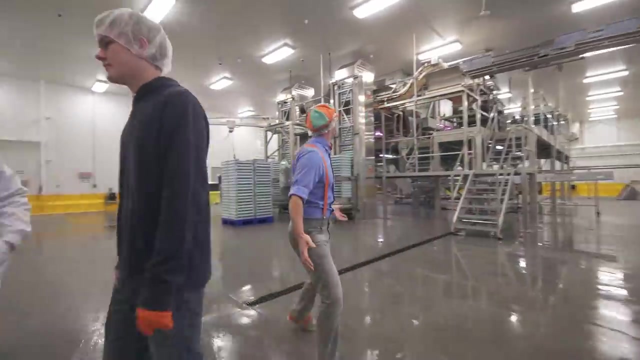 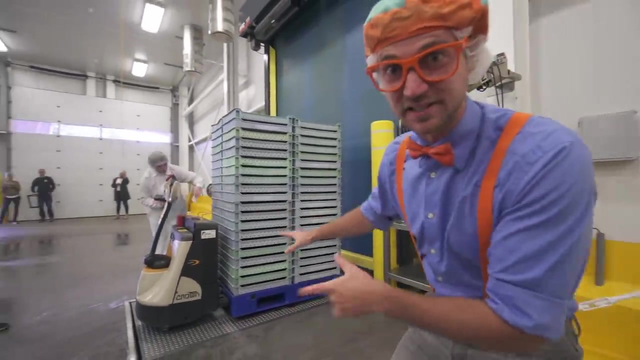 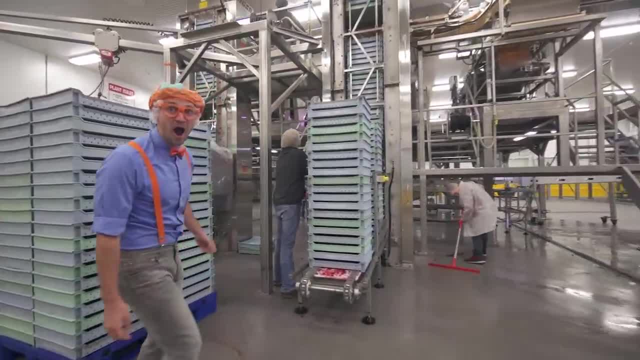 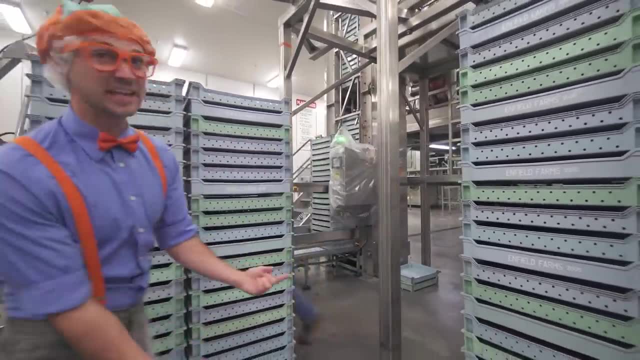 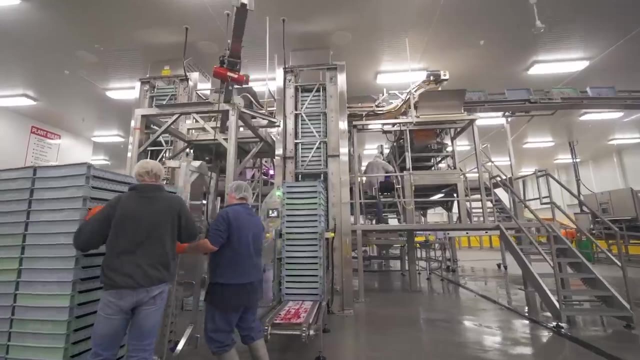 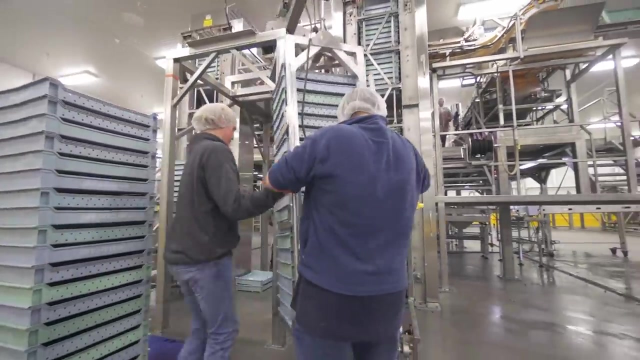 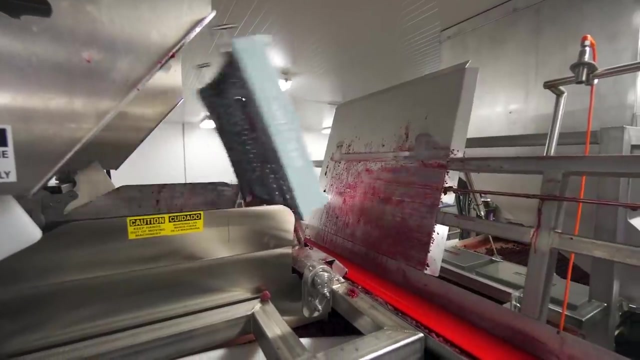 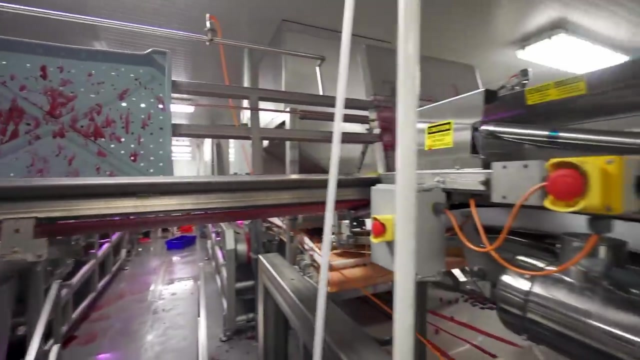 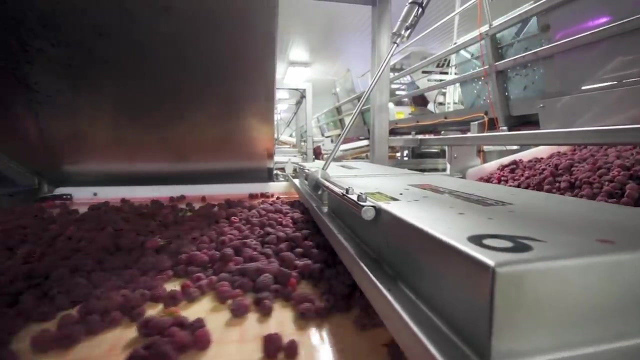 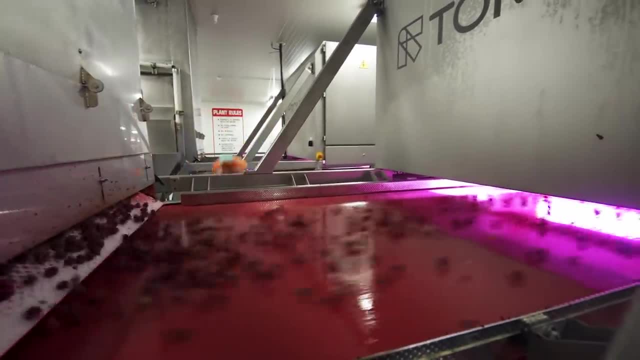 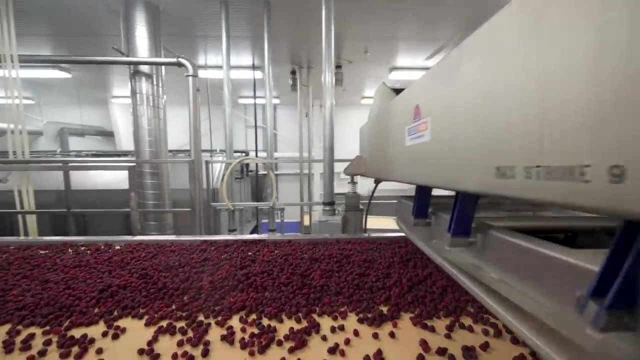 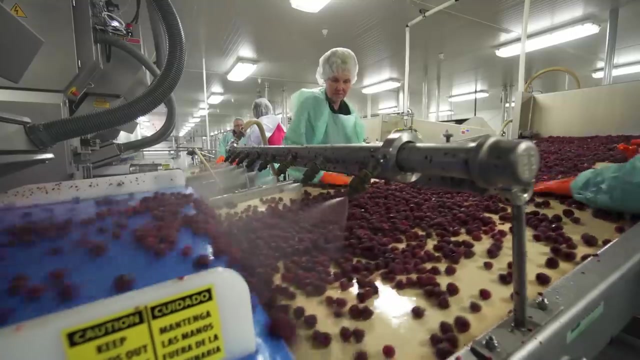 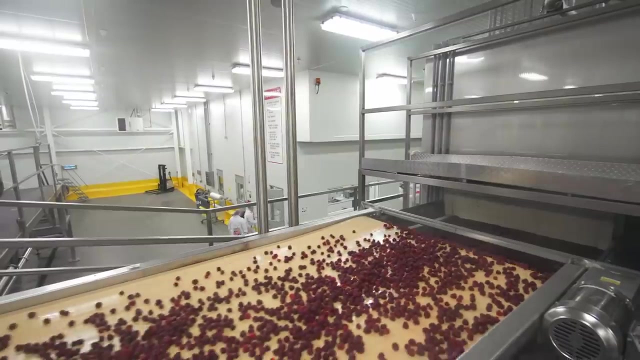 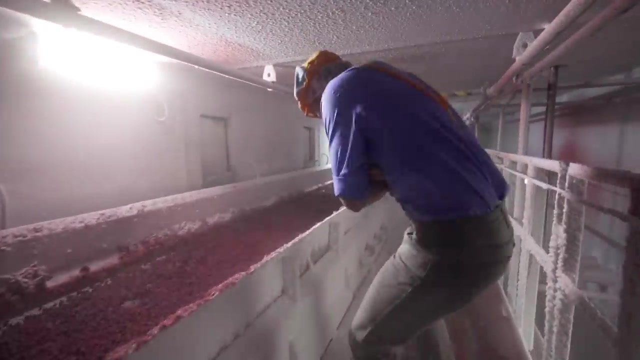 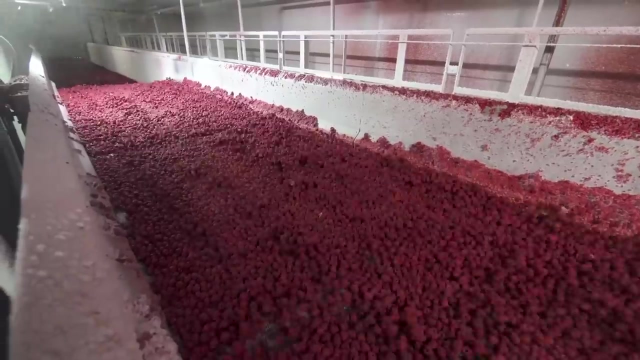 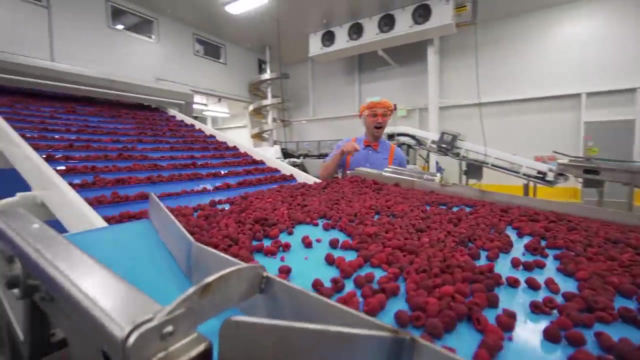 Music, Music. So many conveyor belts- Wow, those look so tasty. Hello, ladies, You're doing a mighty fine job. Now this room is where the raspberries get frozen. It is so cold in here. Look at them Now. all the raspberries are frozen. 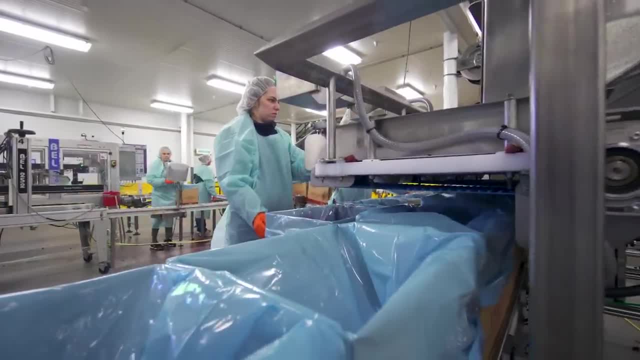 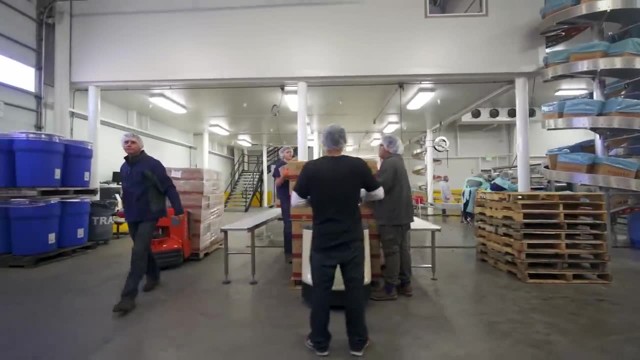 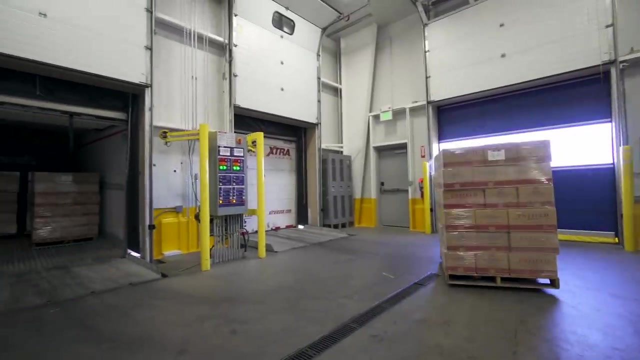 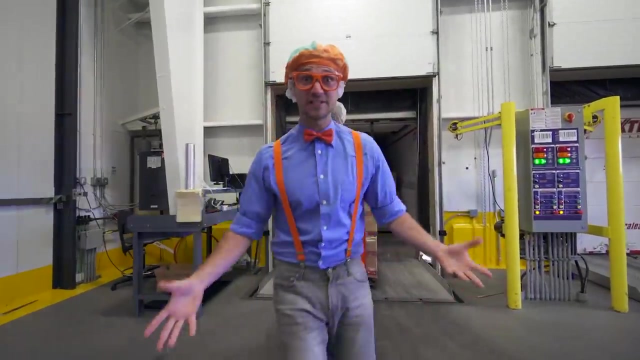 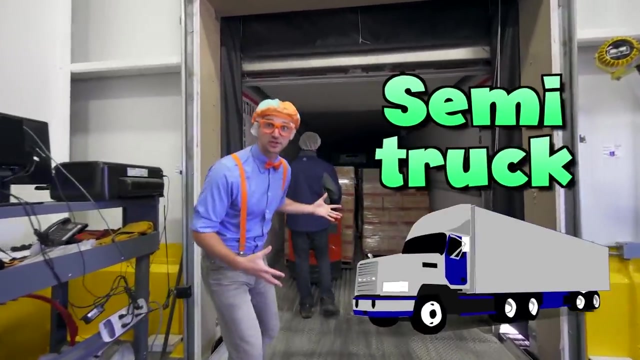 So we have to put them in boxes, All perfectly weighed out. Look at that, Oh, look at all those boxes of raspberries, Wow, Wow. So the raspberries just finished getting packed up into these boxes. So then what we're doing is loading them into the back of a semi-truck. 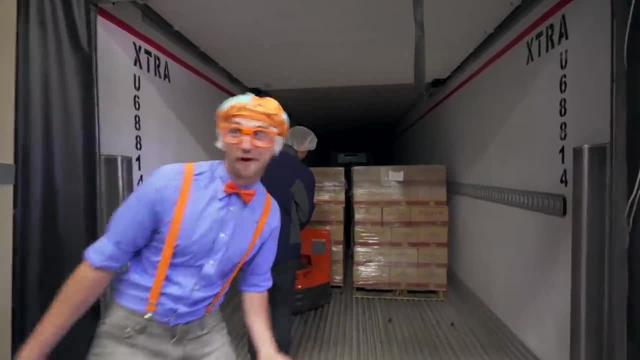 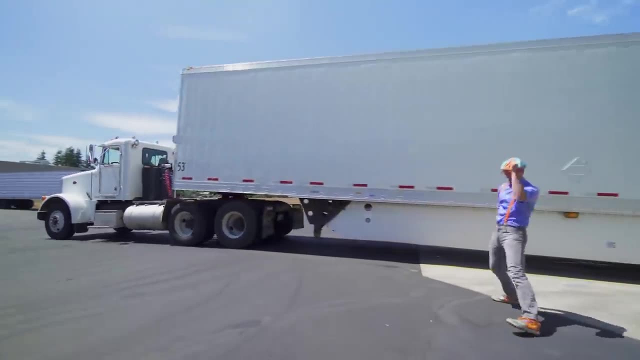 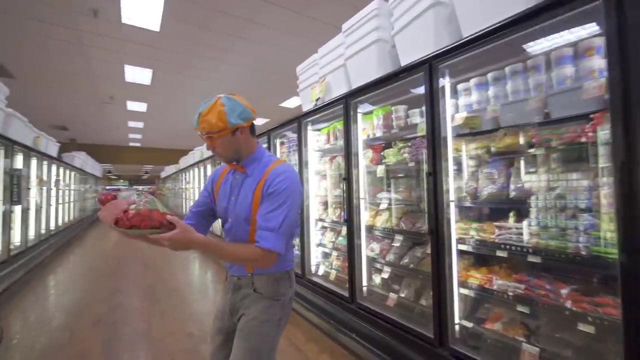 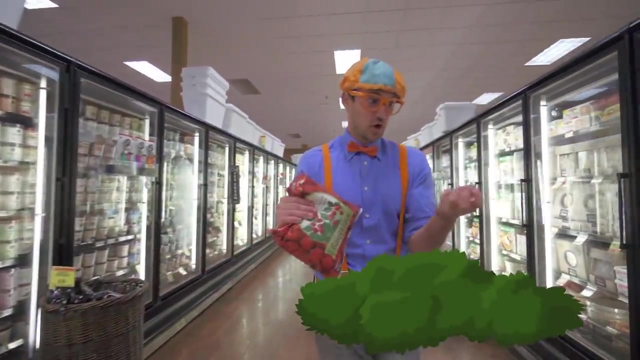 In the semi-truck. The semi-truck is going to deliver it to the grocery store. Oh, so that's how the frozen raspberries got all the way to the grocery store. They grew on the bushes, really big and red, And then the harvester drove down the aisles of bushes. 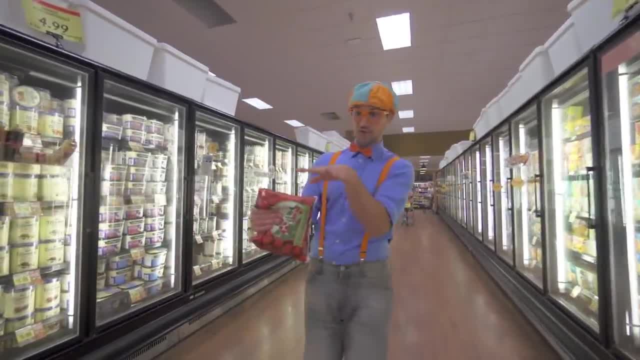 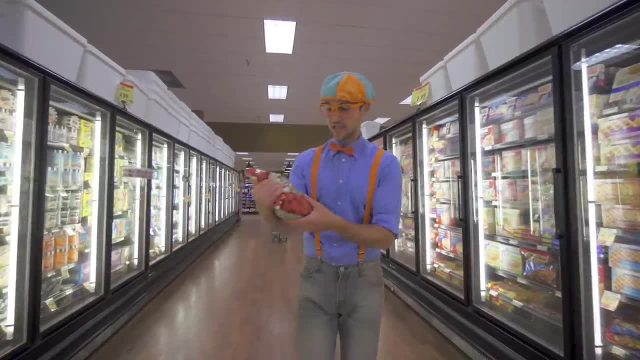 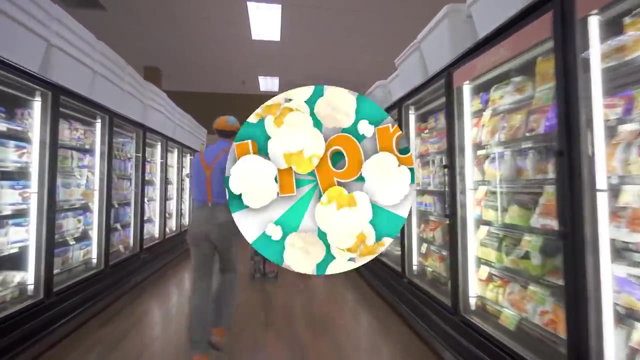 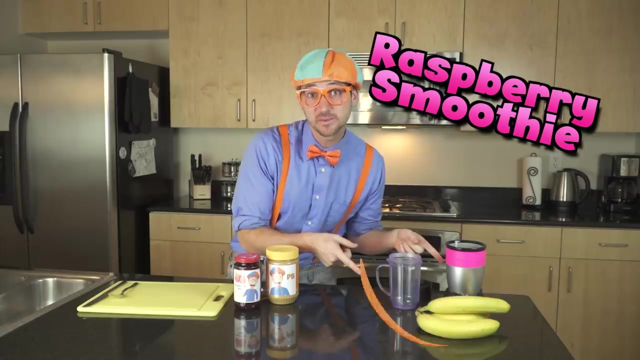 Oh right, And shook them off, And then they get packaged up in these plastic bags. And then they arrived here. Hey, I think we should go make a frozen raspberry smoothie together. Whoo, All right, Now it's time to make a raspberry smoothie and a raspberry sandwich. 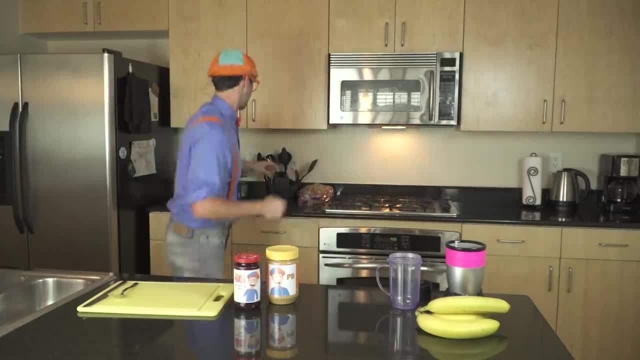 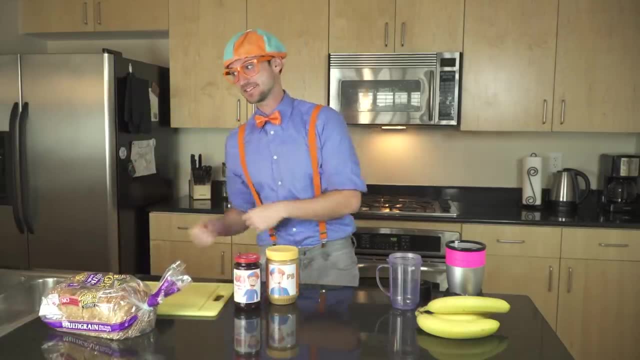 Yum, All right. so let's make a sandwich first, All right? Whoa, whoa, whoa. Before you touch food, you have to wash your hands. Let's go wash our hands. All right, here we go. 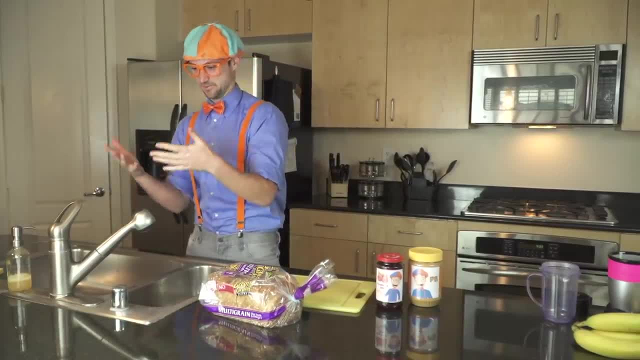 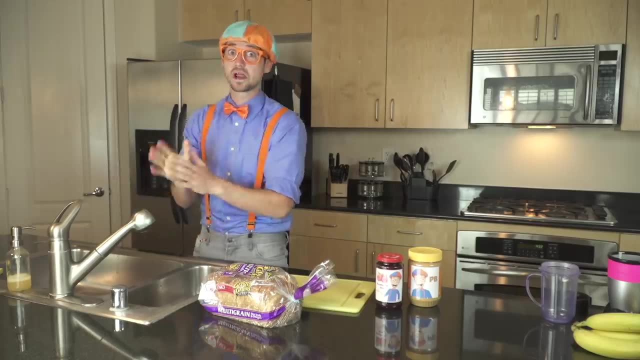 Get your hands nice and moist. Okay, whoa, Now you have to put soap on your hands And then you scrub-a-dub-dub, But I'll tell you the correct amount of time. all right, You have to say blippy. 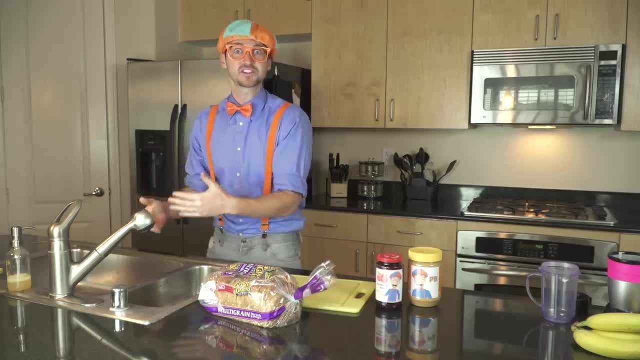 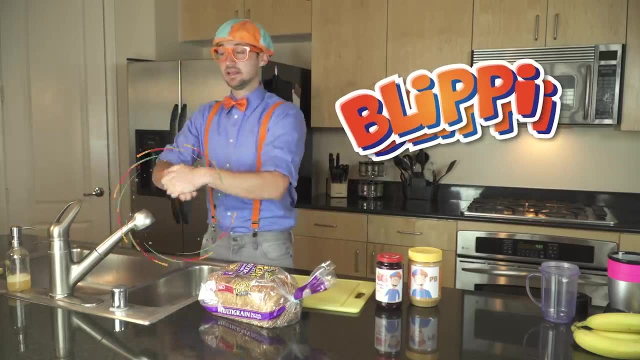 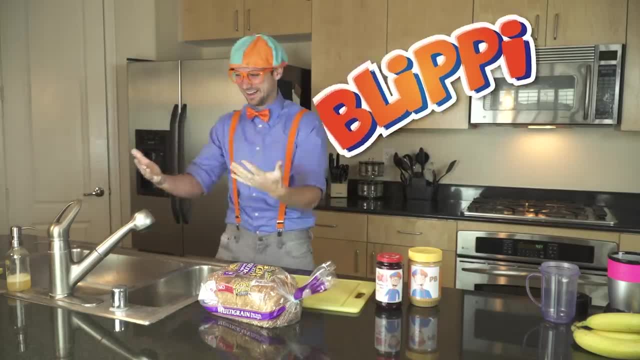 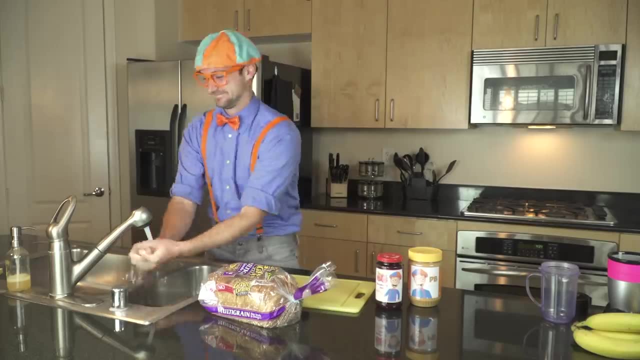 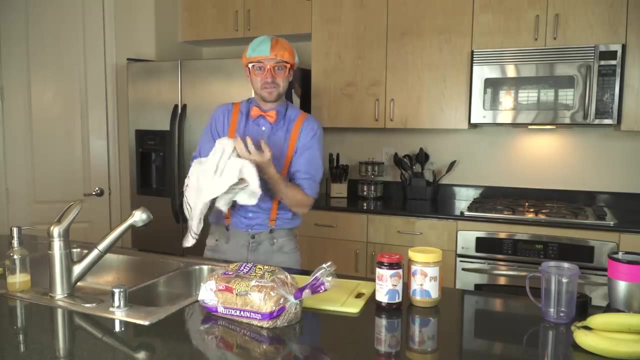 Blippy, Blippy, Blippy. All right, Whoa. Now you rinse the soap off your hands. All right, Dry off your hands, Dry off your hands. I am so excited for the food that we're going to make together. 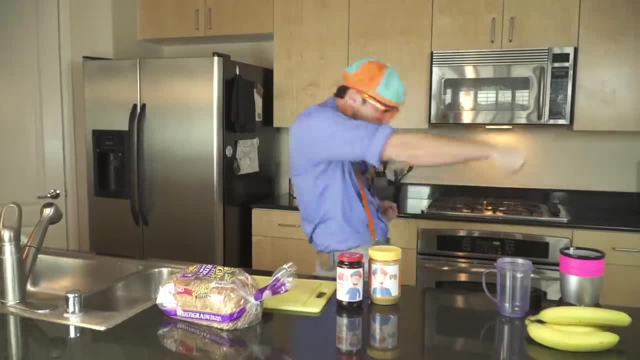 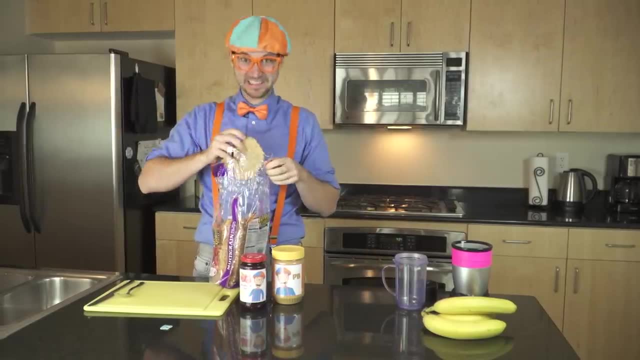 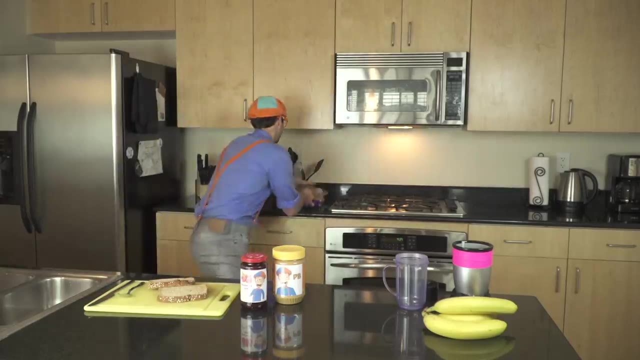 All right, here we go. Let's get some bread for our sandwich. Ooh the heel, Yum. I'll save that one for someone else, though. All right, There we go. One slice of bread, Two slices of bread. 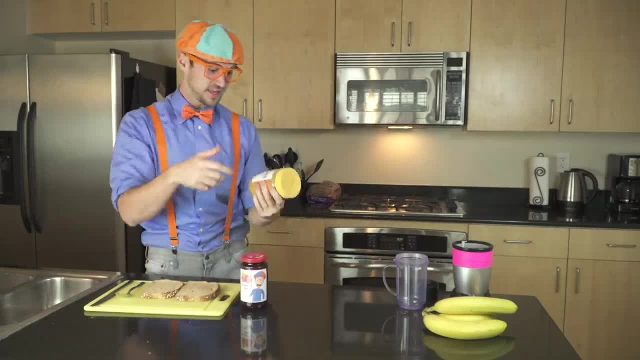 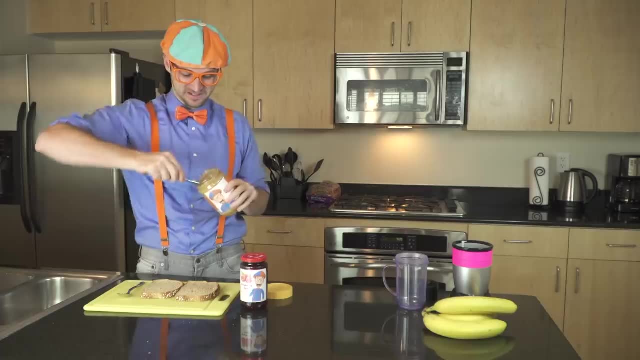 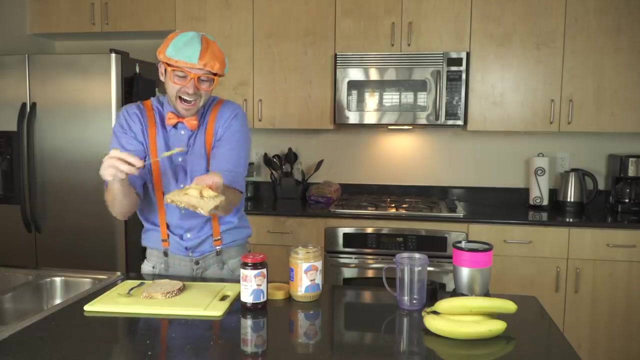 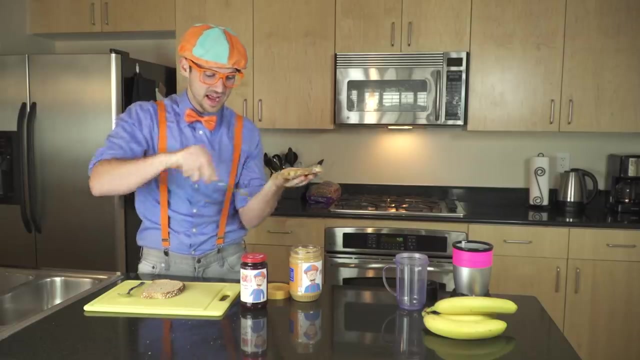 All right, There you go. All right, Let's start out with some peanut butter. Yum, Take a big scoop. I love peanut butter. Okay, Okay, Slop it around. Ooh, yeah, Look at that Yum. 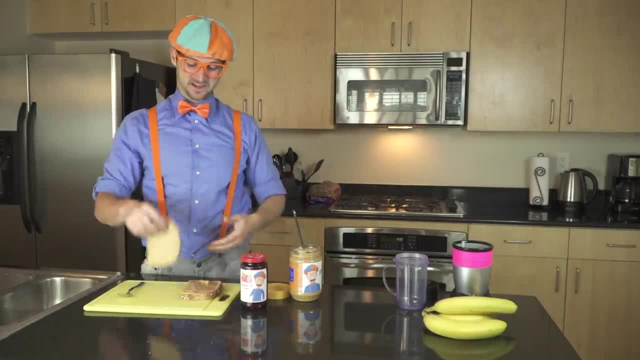 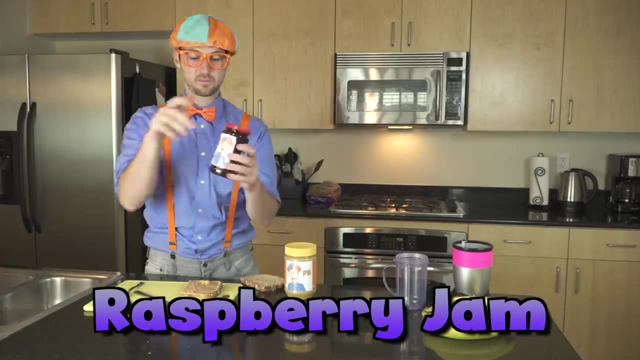 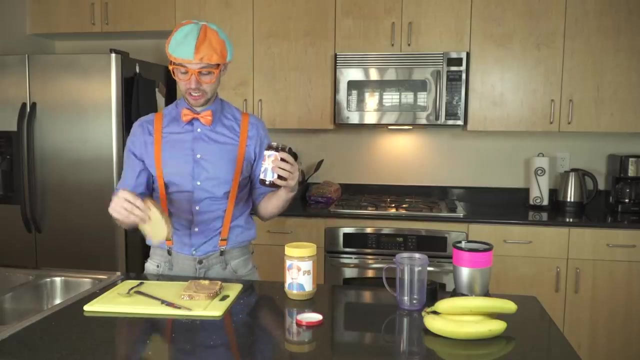 Yum, Yum, Yum. Okay, And on this other side we are going to put some raspberry jam. Mmm, this sandwich is going to taste so good. All right, Take a big scoop of raspberry jam, Plop it right there. 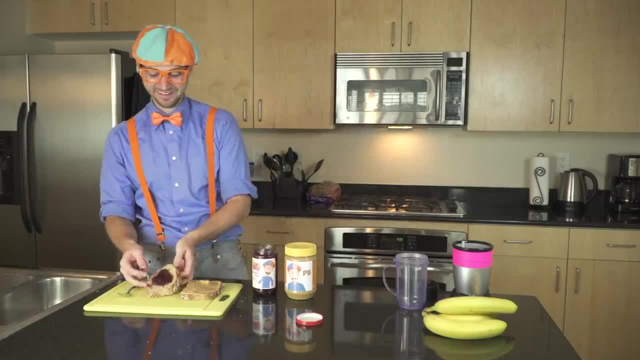 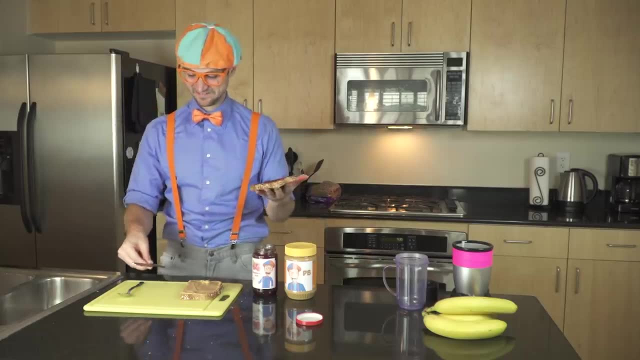 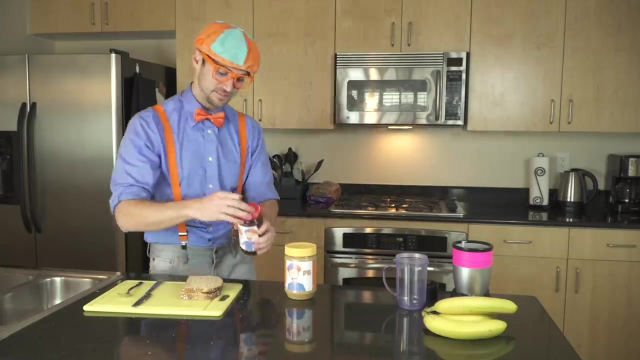 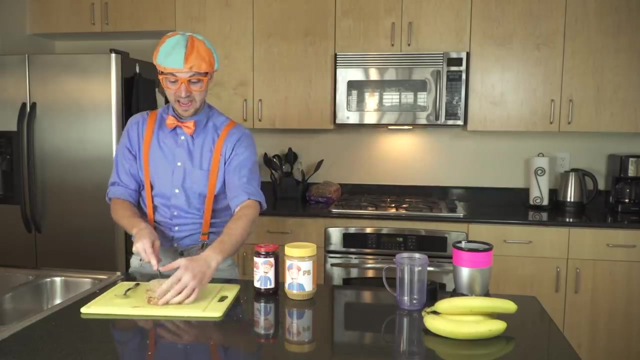 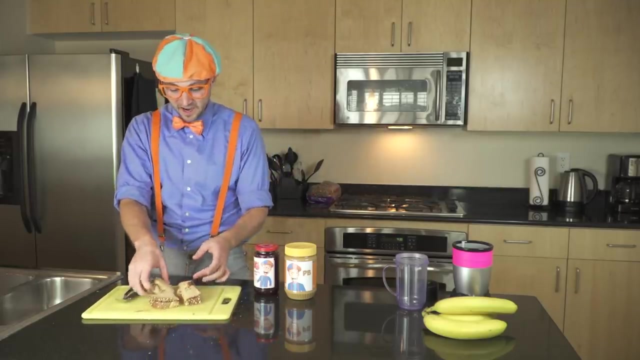 All right, Spread it around, Oh yum, Yum, All right, Put it down. Put the lid back on. All right, Here we go. Let's cut it in half, All right, And let's cut it into quarters. Yum, Look at that. Whoa All. 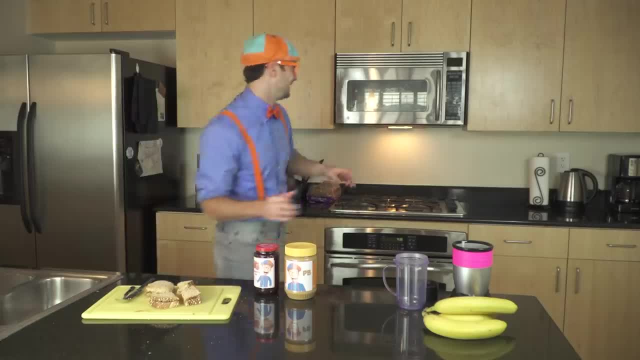 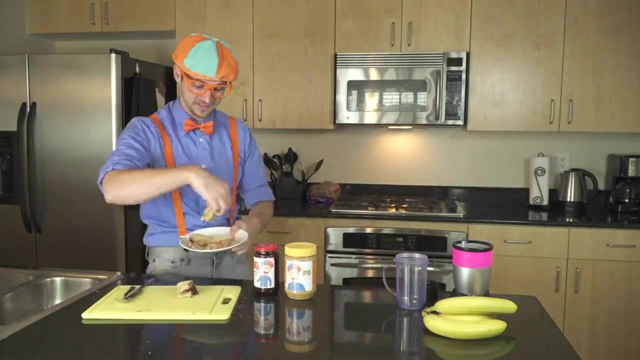 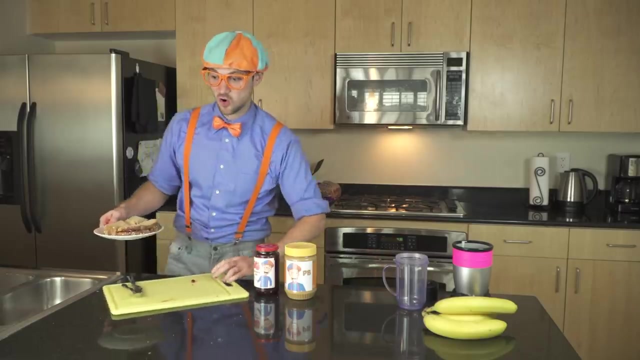 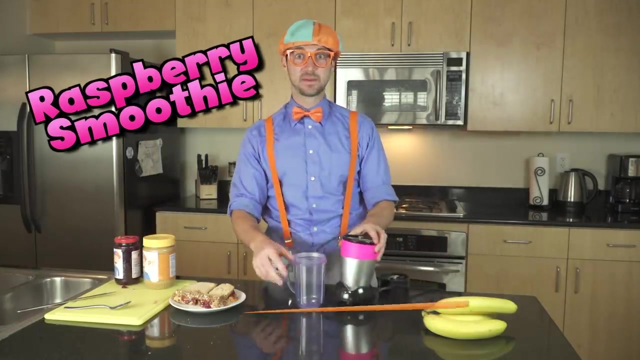 right, Let's put this on a plate. All right, One, two, three, four, Oh yum, All right. You know what Beverage would be so tasty with this raspberry sandwich? Yeah, A raspberry smoothie. Okay, I'm going to teach you how to make one. First, we need to go ahead and 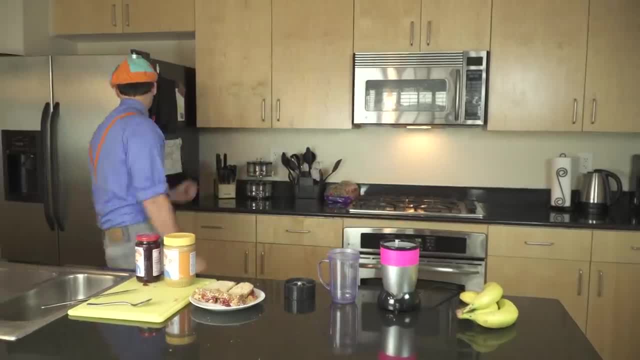 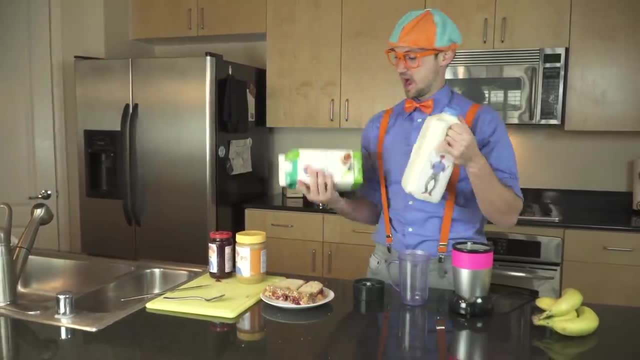 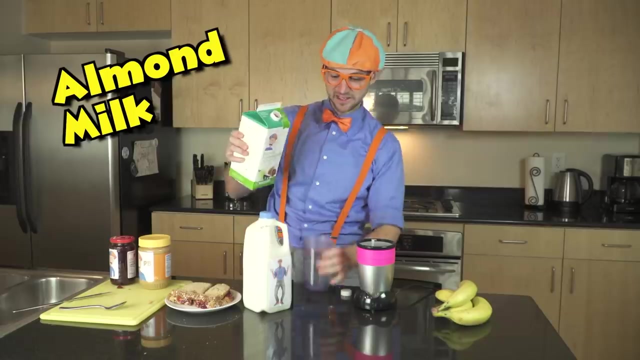 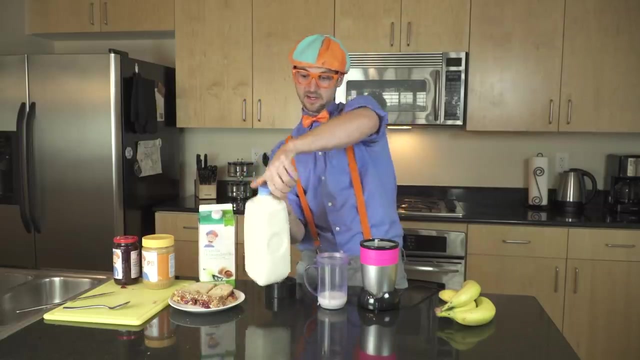 go get our milk. Hold on, Okay. So I have almond milk and normal milk, So let's put a little bit of almond milk in here. Perfect, That looks great. And let's put a little bit of normal milk in here. 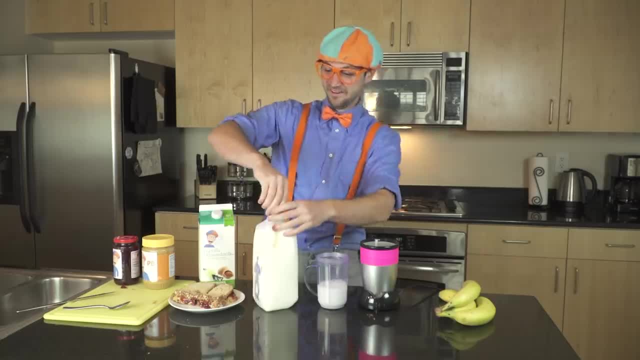 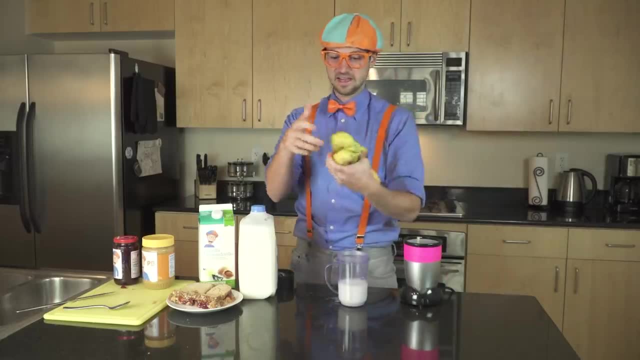 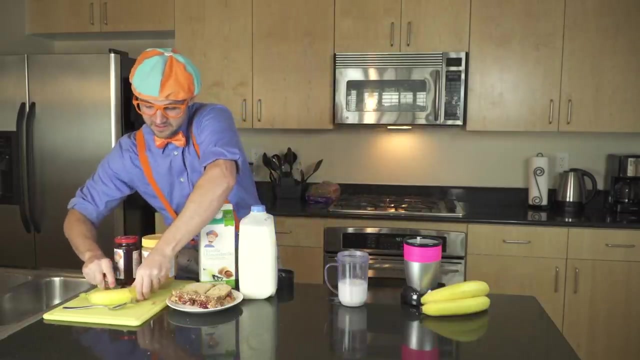 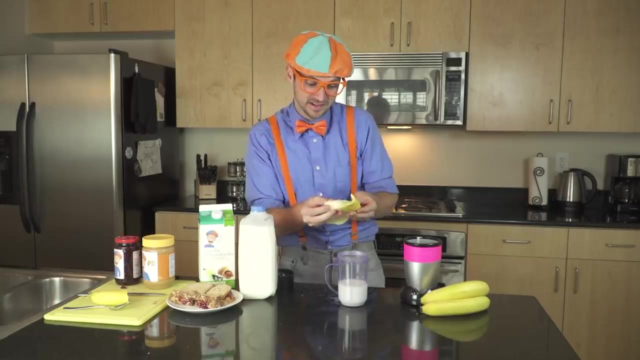 Okay, Perfect, I spilled a little. Look, That's okay, We'll clean it up after All. right, And let's take a banana. Let's actually cut it in half, because that's a lot of banana. I want more raspberries than banana, But I still do like banana. Bombs away, All right. 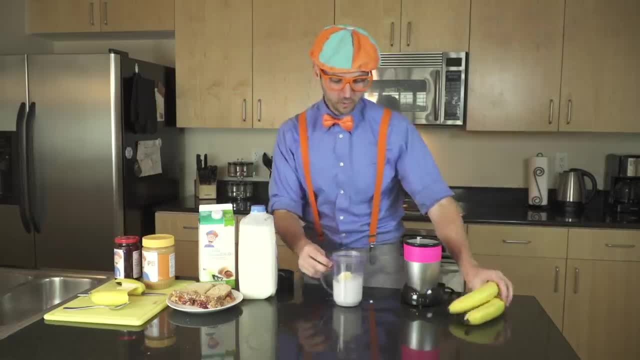 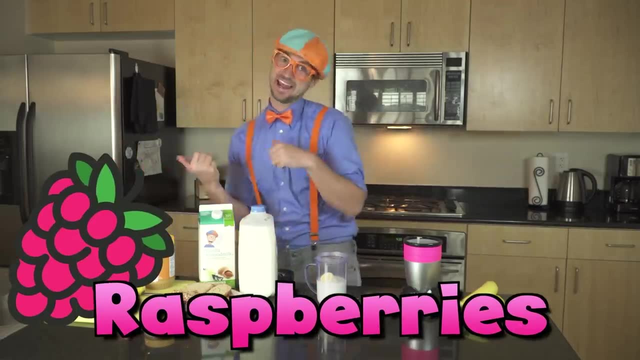 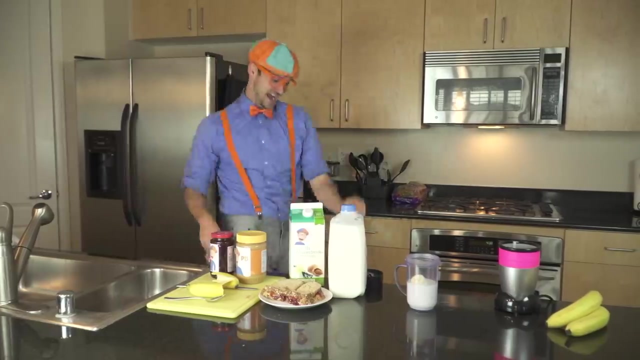 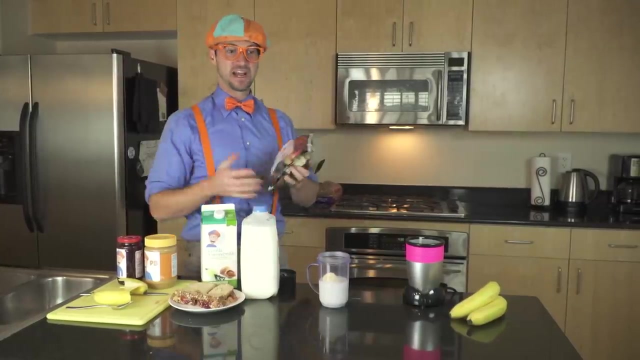 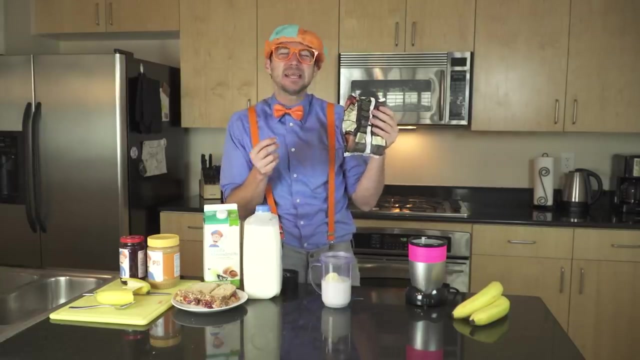 All right, Yum And wait. What are we missing here? Yeah, Raspberries. Okay, I need to go get them from the freezer. Yeah, Frozen raspberries. I use frozen raspberries because they're really good in here, because then it makes it nice and cold and then it feels like little ice. 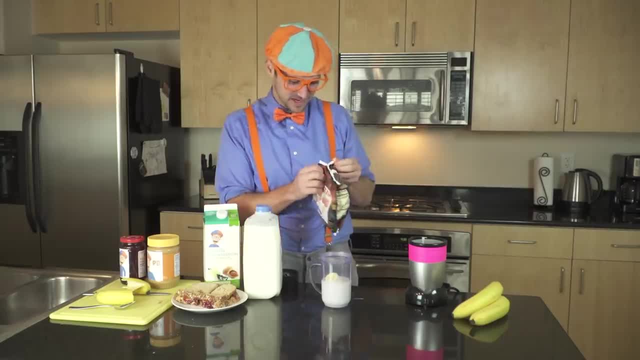 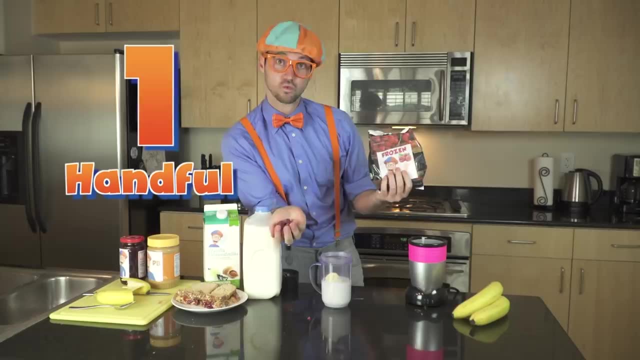 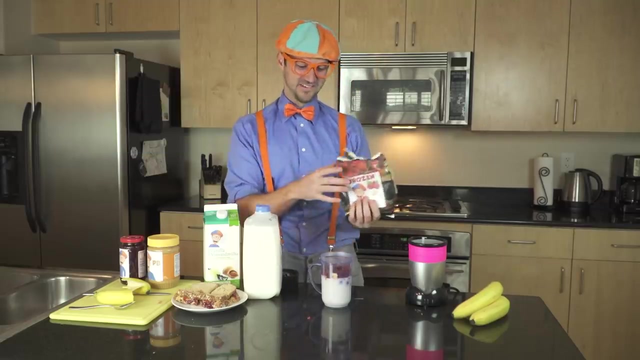 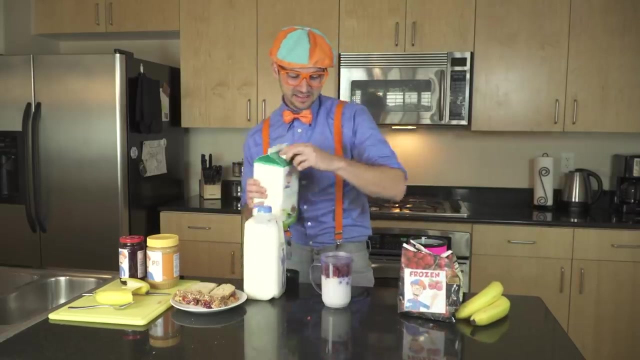 chunks. All right, How do we open this? There we go. All right, The correct amount is one handful. Nope, It's two handfuls. Yeah, There we go. Yeah, Okay, There we go, And let's add a little. 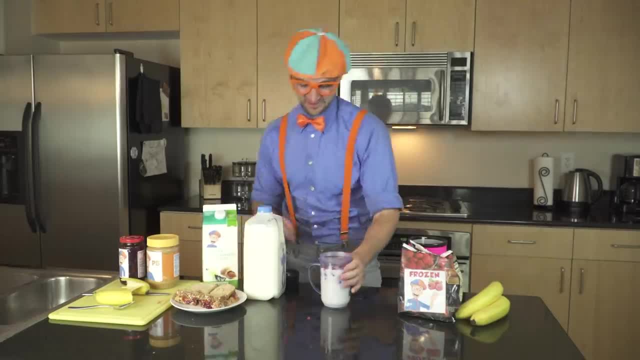 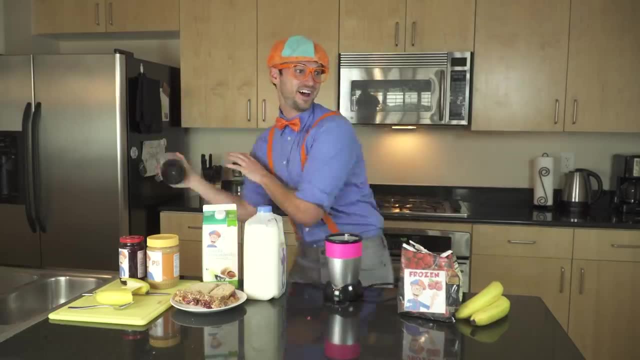 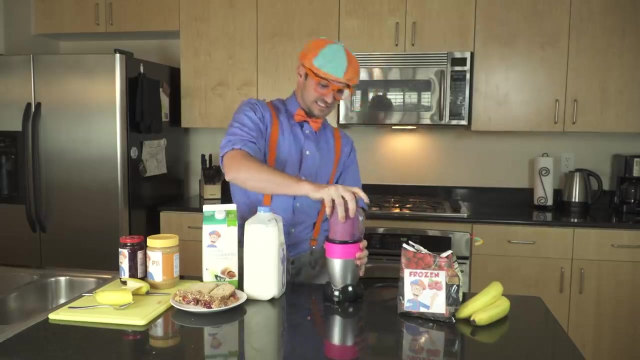 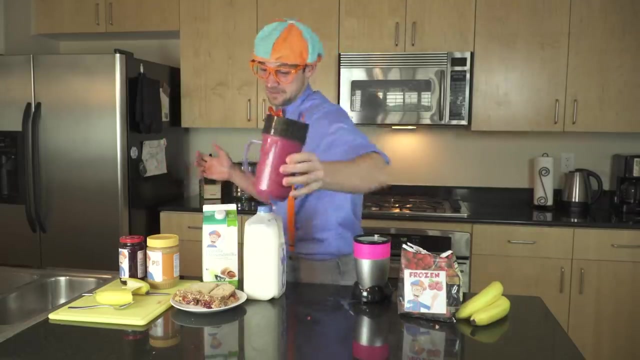 bit of extra almond milk, Perfect. All right, Let's put the lid on, Give it a little shake. Yeah, Now let's blend it on up. Wow, yum, That looks so tasty. Okay, I'm going to get a glass. 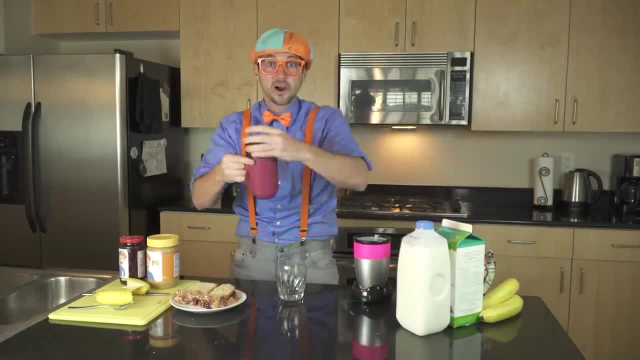 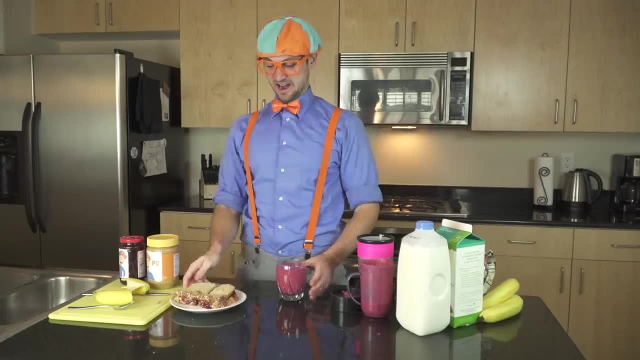 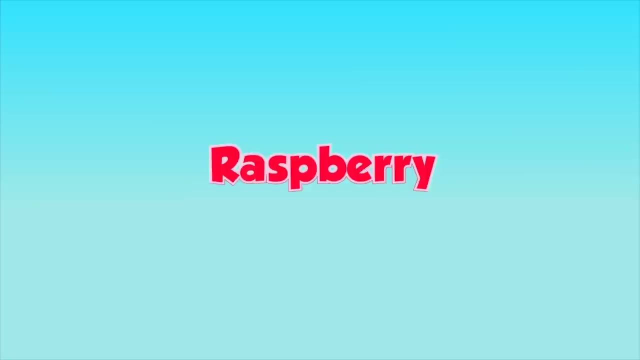 Perfect. Yum Alright, let's pour our smoothie. Yum, Alright. now it's time for the raspberry song: Raspberry- ras-ras-berry- Raspberry- ras-ras-berry- A tiny fruit. raspberry. Raspberry- ras-ras-berry- A tiny fruit raspberry. 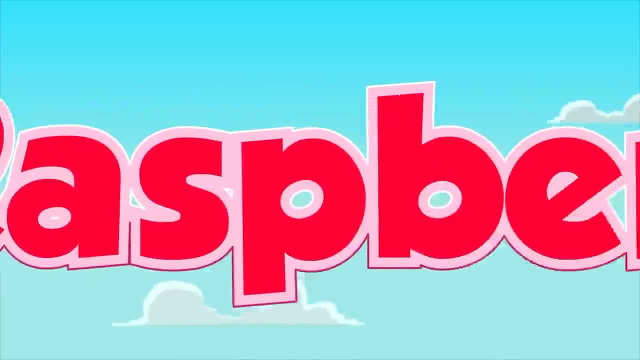 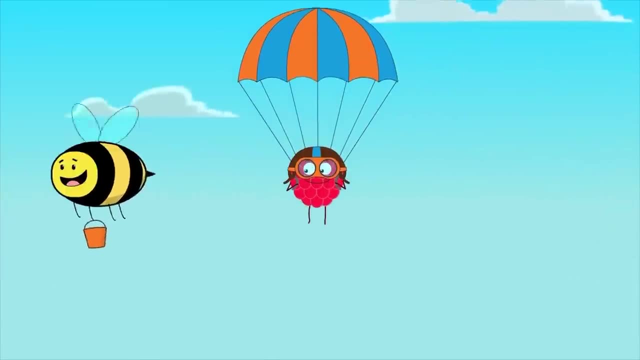 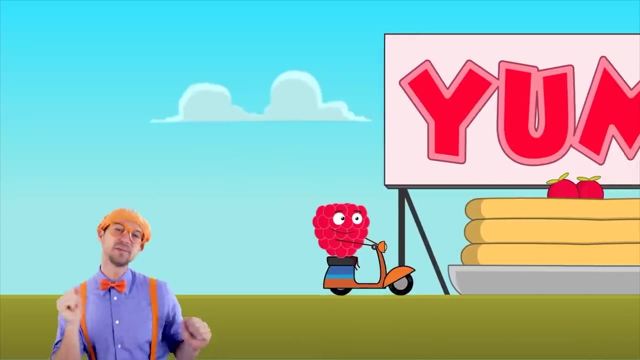 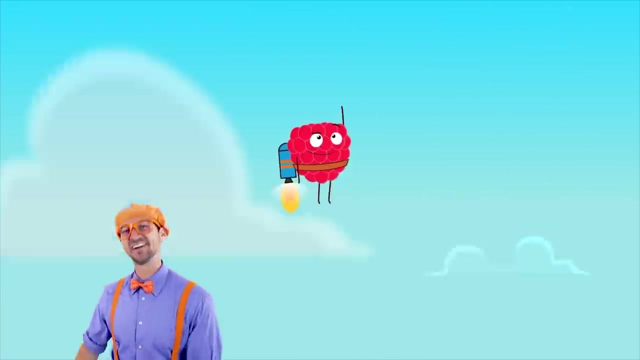 Red and sweet, called a raspberry. Raspberry ras-ras-berries Grows on a plant loved by honey bees. Raspberry ras-ras-berries Raspberries- I think they're very, very yum On waffles and in yogurt cups. Raspberries- I like them very, very much And I just can't get enough. 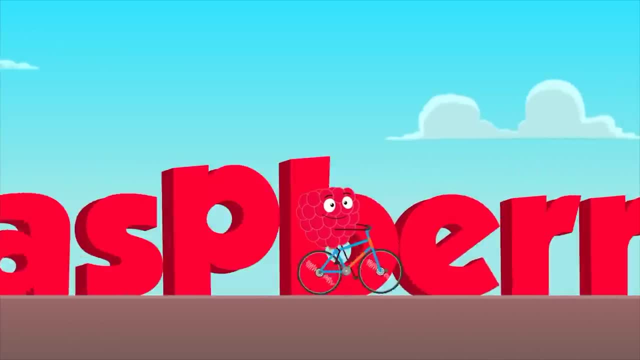 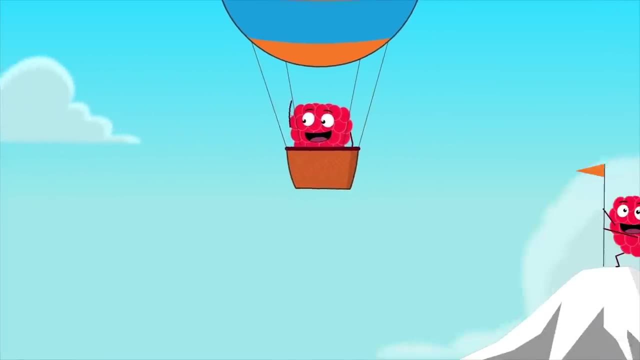 A wonderful jam, juice and pie filling: Raspberry ras-ras-berries, A frozen treat on top of your ice cream: Raspberry ras-ras-berries. And they're full of vitamin C. Raspberry ras-ras-berries, Raspberries- I think they're very, very yum. Raspberry ras-ras-berries. 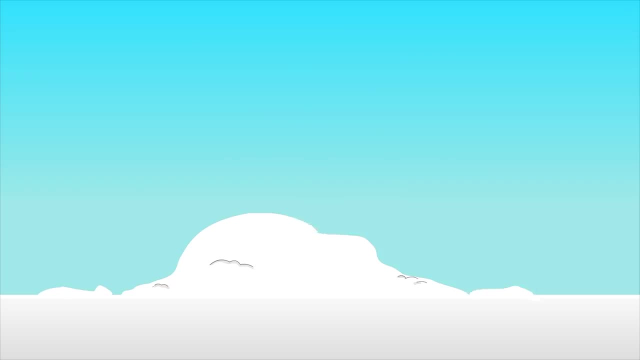 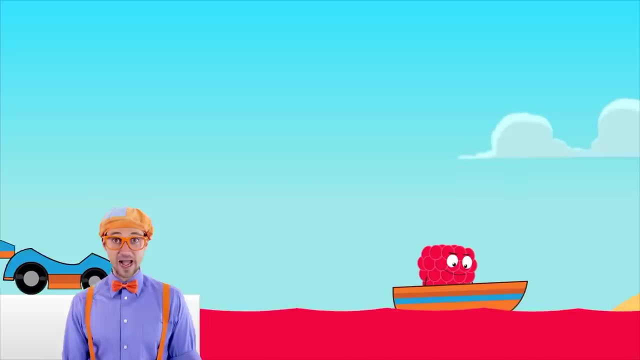 Raspberries. I like them very, very much. Raspberry ras-ras-berries- A-S-P-E-E-R-R-Y. Raspberry ras-ras-berries. And anytime you can make a cool smoothie, drink Frozen raspberries. Hey, can you spell raspberry with me? 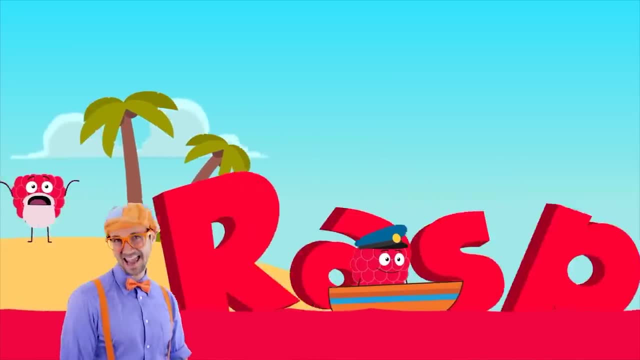 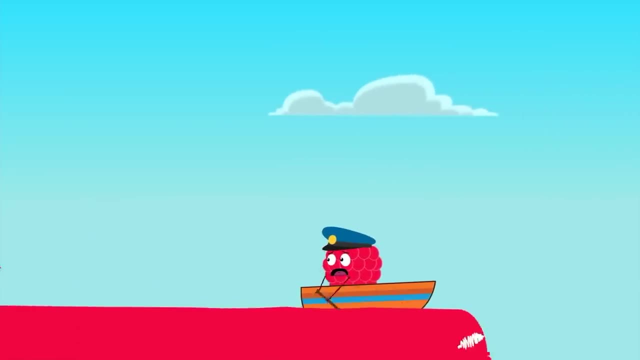 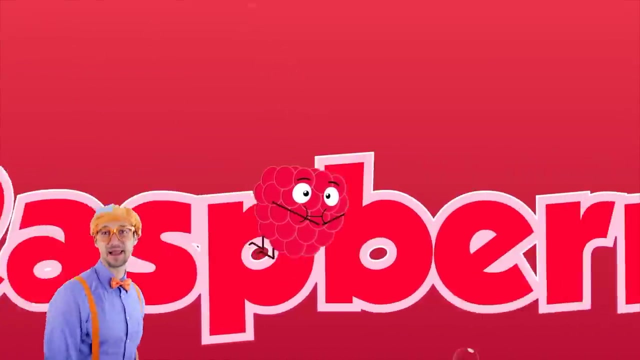 Okay, here we go: R-A-S-P-E-E-R-R-Y. You did it Great job. Come on, everybody, sing along with me. Raspberries, I think they're very, very yum, Raspberry ras-ras-berries. Raspberries, I think they're very, very yum, Raspberry ras-ras-berries. 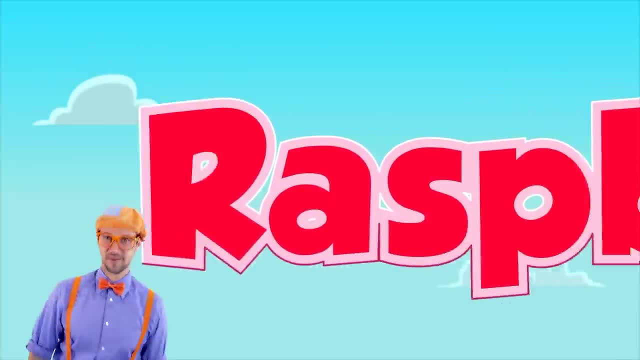 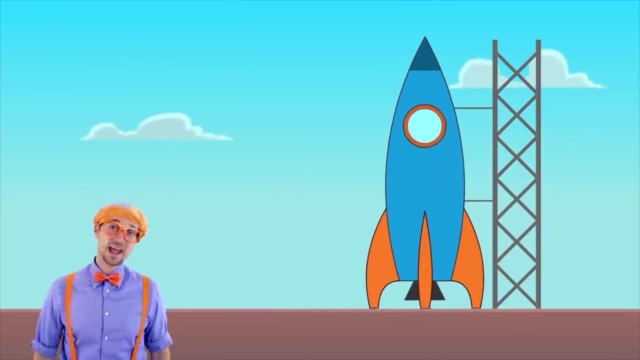 Raspberries are very yum. Raspberry ras-ras-berries Raspberries- I like them very, very much. Raspberry ras-ras-berries Raspberries- I like them very, very much. Raspberry ras-ras-berries. Let's spell it one more time. 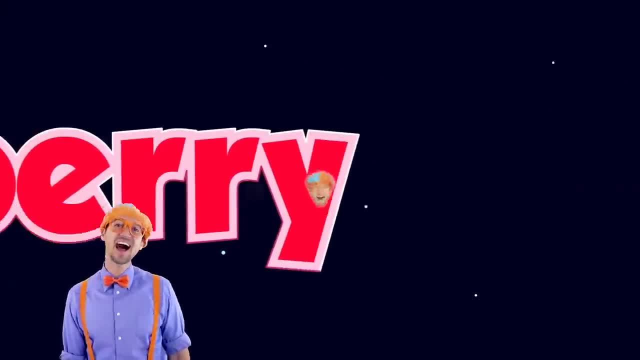 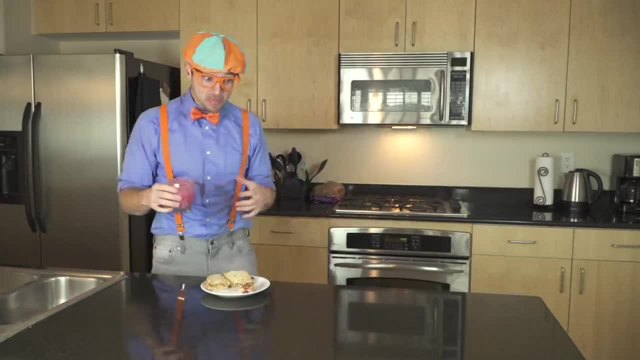 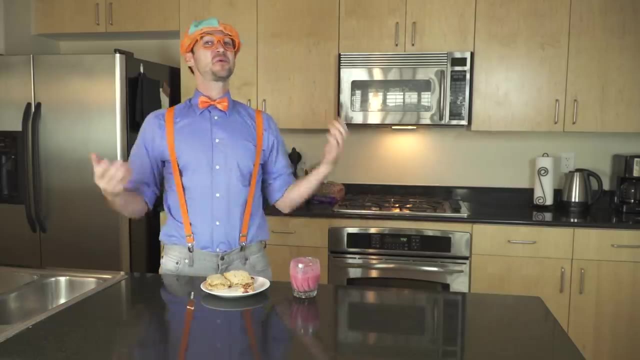 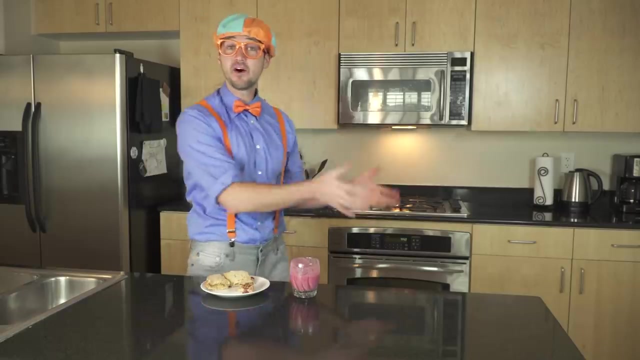 R-A-S-P-E-E-R-R-Y. Yum, This food is so tasty. Well, I sure did have a blast learning with you about how raspberries go all the way from the farm to your tummy. Well, if you want to watch more of my videos, 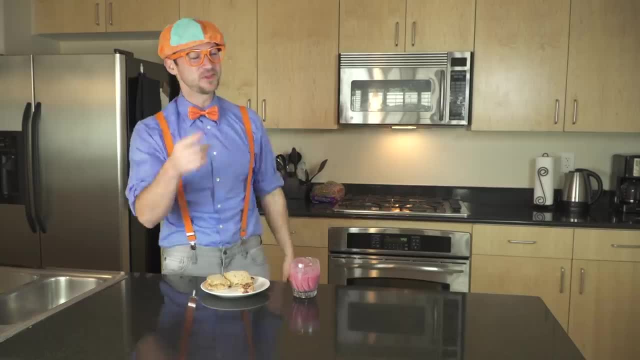 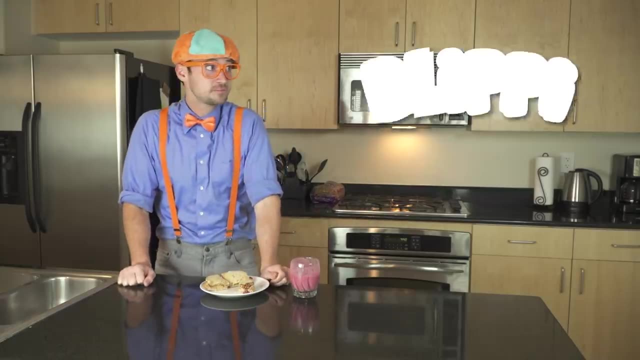 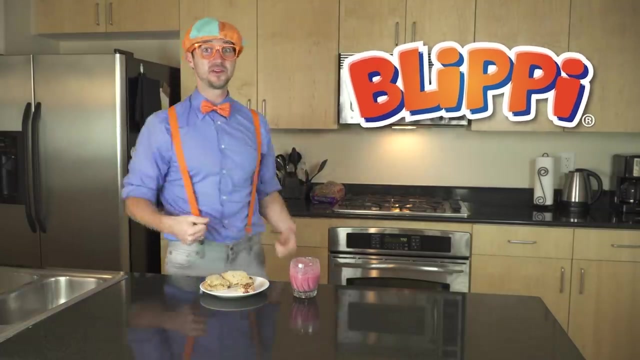 all you have to do is search for my name. You know my name right? Yeah, it's Blippi. Let's spell it together: Ready B-L-I-P-P-I, Blippi. Good job, Now you know how to say and spell my name. See you again, Bye-bye.